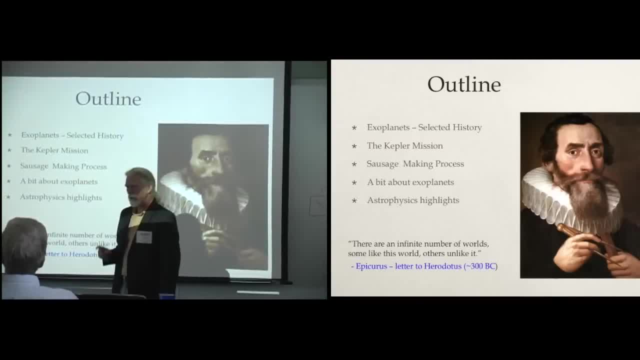 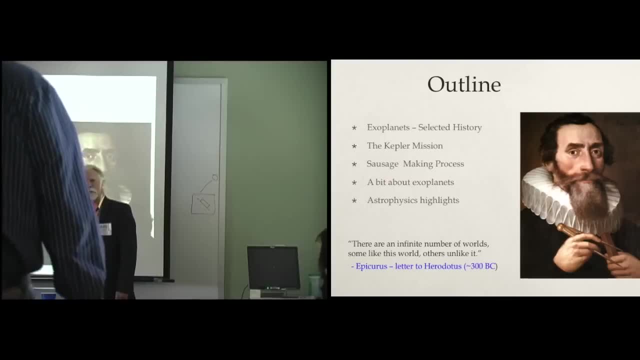 curves out of that. So I hope you'll be interested in some of that. But I wanted to start with a little history. It's always important, I think, to look back on history a bit and see what kinds of things people thought about, what kinds of things they knew or didn't know. 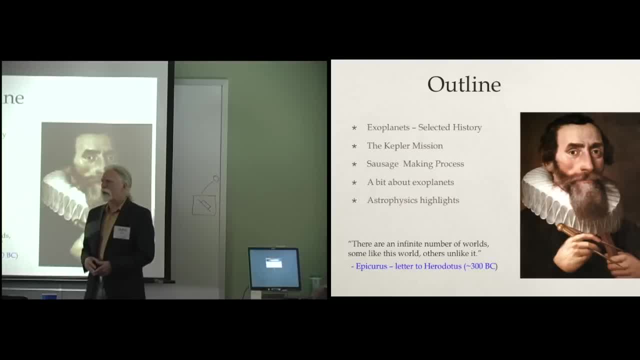 and how to find our place And Kepler's this sort of very philosophical mission at some level. And another talk I could have given but I won't today- is on all the religious aspects that Kepler has realized. So it's definitely brought to light within NASA and within the Kepler Project and people. 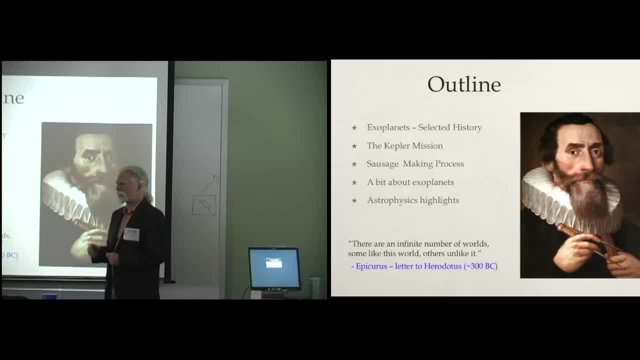 we talk to and people we don't want to talk to. But it's very interesting stuff to pull another thought Anyway. so I'm going to talk a little bit about history. then the Kepler mission. if you haven't seen pictures of it, I'll show you some of the pictures of the 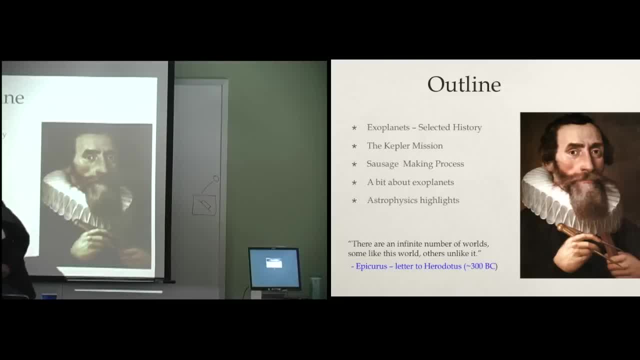 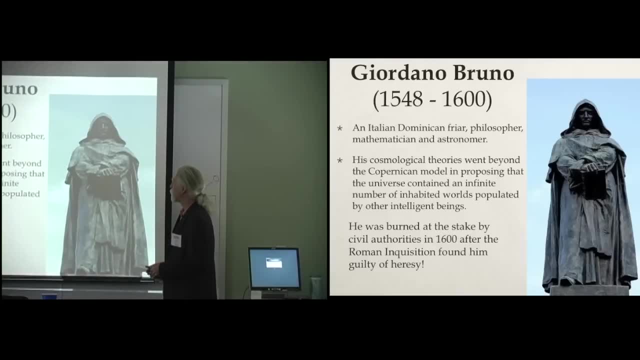 spacecraft and stuff, And then sausage making planets and stars. So Bruno, Everybody knows Bruno. If you take a philosophy class you have to learn something about Bruno. So late 1500s he was. you know everything If you could read the history. 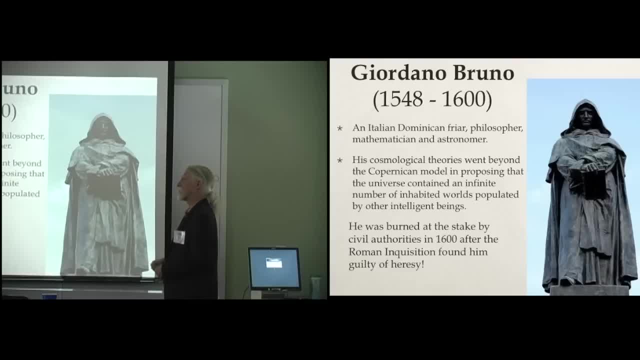 class you could read, You had all these names out to you, You were, you were a mountain fishing, astronomer and everything. because you could read. And he believed in these theories that went beyond sort of the Kernigan model and talked about that there were other inhabited. 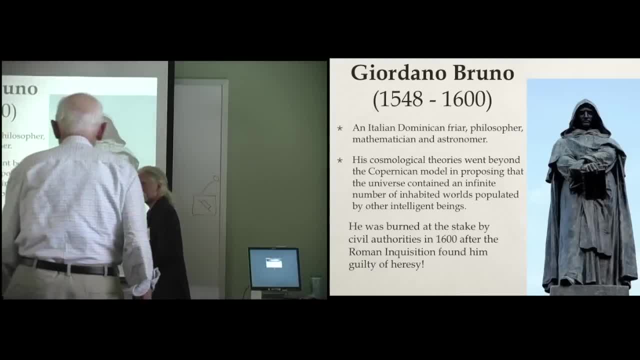 worlds- And of course this is not a good thing to say- in the late 1500s in Italy. And so what happened to Bruno is he was burned at the stake for this. Fortunately, today we can say these things And so far we don't get too burned at the stake. The Roman imposition hasn't 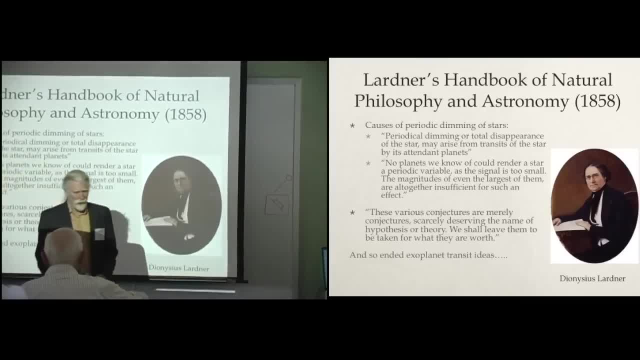 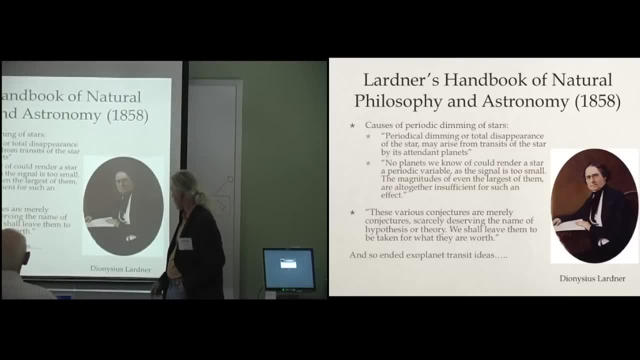 shown up yet, But we have had some nasty vote. calls Another person who I suggest, if you're interested in a loony crazy scientist, look up this guy here, This guy Lardner- I mean he looks a little weird, But look him up. He had a. 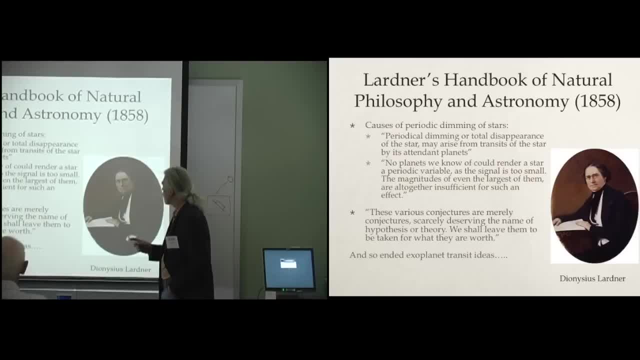 really interesting life as a sort of scientist, But one of the things he did was he wrote this physics or this natural philosophy and astronomy book. It became really popular in the mid-1800s And that's good, you say, But the bad part about it is that people read: 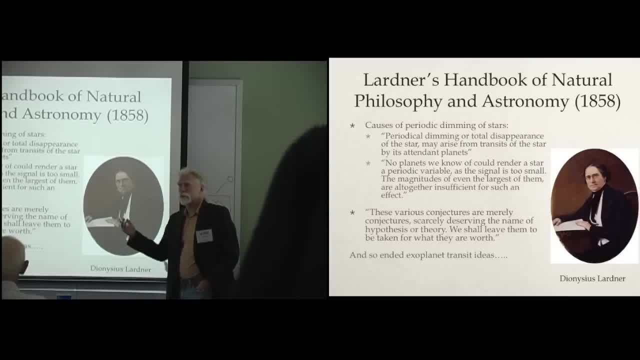 these things And what you say in there they believe is some kind of truth, And that's some kind of a fact or some truth. And this guy was talking about how you explain variable stars, And at that time people knew about variable stars, things like Cepheids and Aralaras. 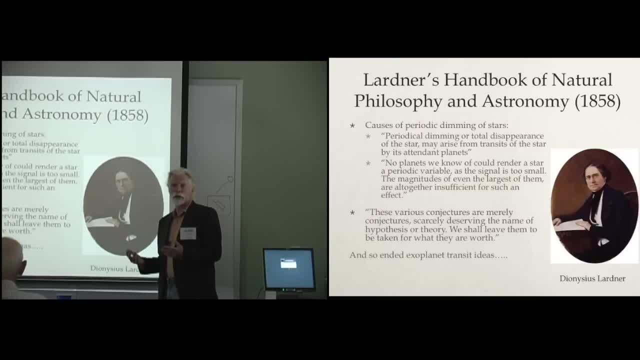 some eclipsing binaries that change their brightness by enough you can see with your eye And it's pretty obvious in some cases. So he talked about them and said, hey, maybe these are due to planets. They're actually passing in front of that star And they went. 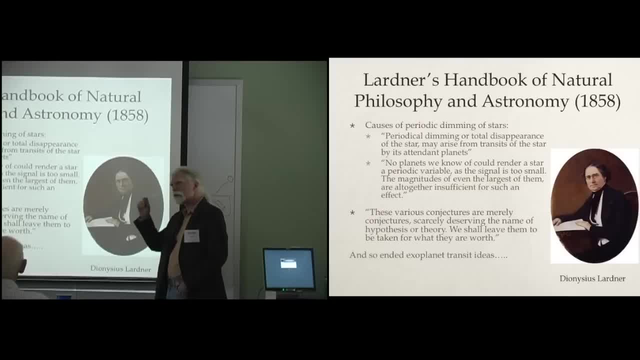 on to say: well you know, if it wasn't a planet, like in our solar system, the signals would be too small for anybody to ever detect. So let's just forget this. This was just a theory, because it's really crappy. So we'll never think about planets orbiting stars anymore. 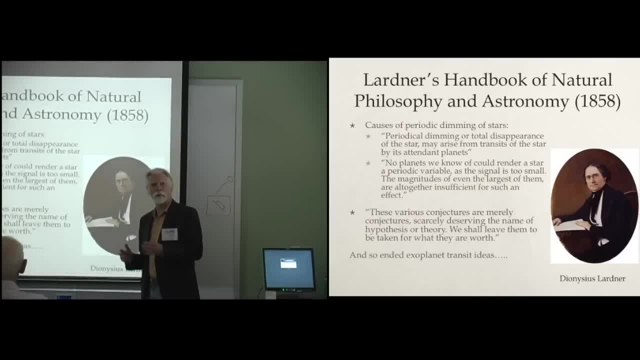 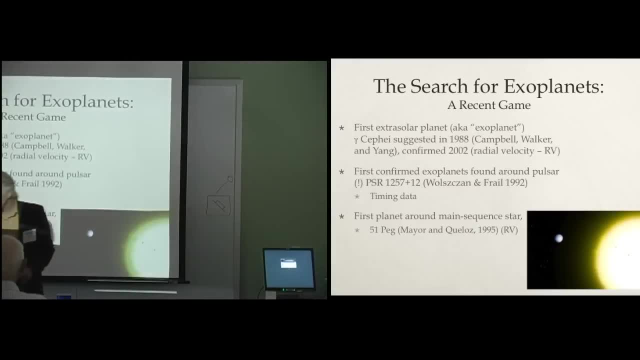 And this really had a profound effect in the literature on people not believing that you could ever detect planets, even into the late 1900s. So exoplanets is a young field. In fact, this field is almost as young as some of you people. 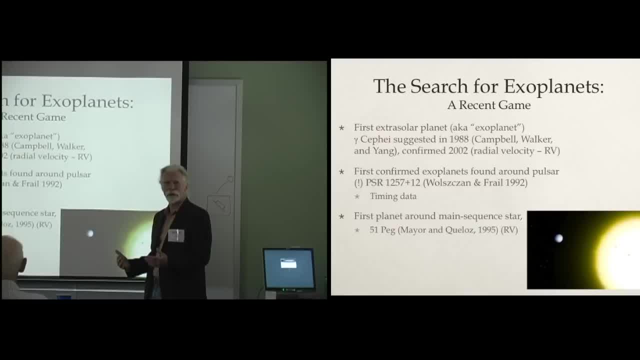 in the back of the room. You kind of are growing up with exoplanets. For those of us that are a little older than the people in the back of the room, we remember a time when we were in the 20s and the word exoplanet didn't even exist And nobody even thought about. 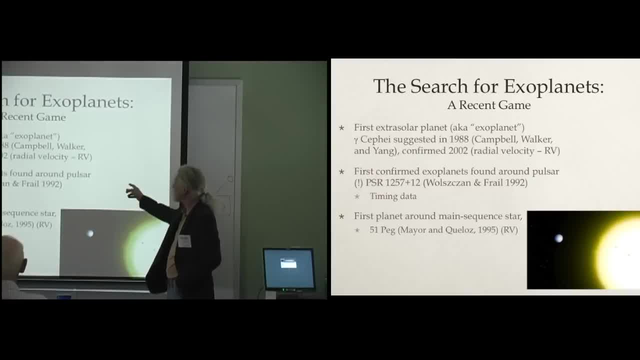 finding planets around other stars, So sort of. the first attempt here was in 1988. And it was suggested and the phrase exoplanet was coined in this paper. but no one believed that they were really going anywhere until a number of years later where it was confirmed. 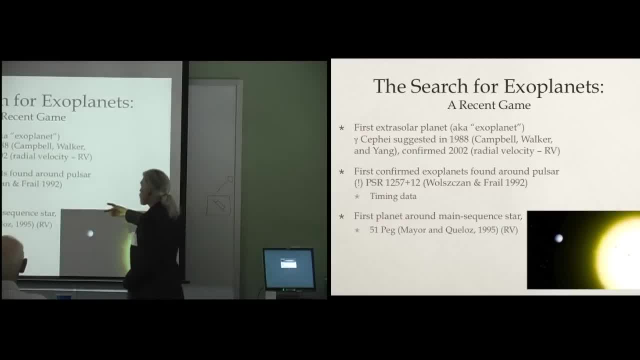 by radio velocities. The famous two are these: These are probably the ones you read about in textbooks and learned about The planets that were found around the pulsar by using timing variations- And that's interesting because Kepler uses timing variations to timing variations, as well as transit detections for different things. they can learn about planets. 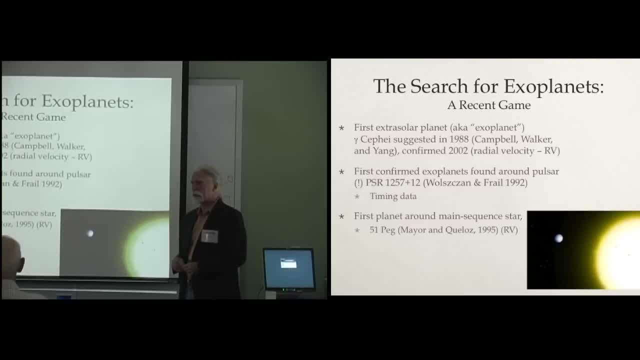 and then 51 peg, the sort of first hot jupiter famous planet that was found in 1995. it kind of set the stage for the fact that we believed at that time that the most common solar systems were solar systems with inner large plants, the so-called hot jupiters, because those were the 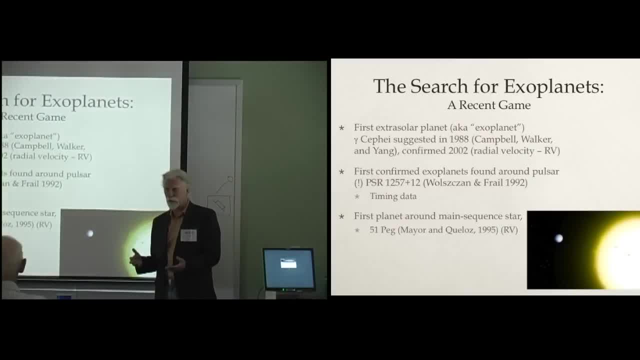 ones that were being found from the ground. we knew 15 or 20 of those and our solar system seemed to be completely wrong. so, if nothing else, kepler has shown that our solar system looks like pretty okay, so you can breathe easily again. it's okay, jupiter's probably not going to come screaming. 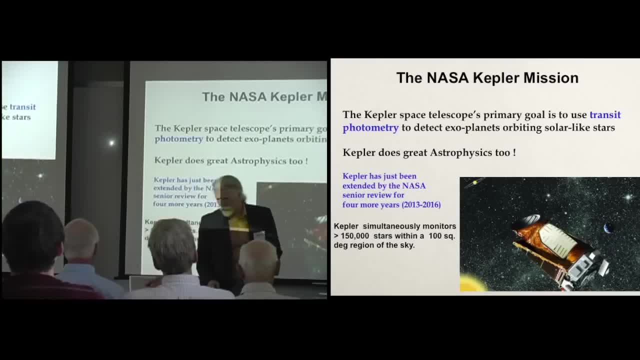 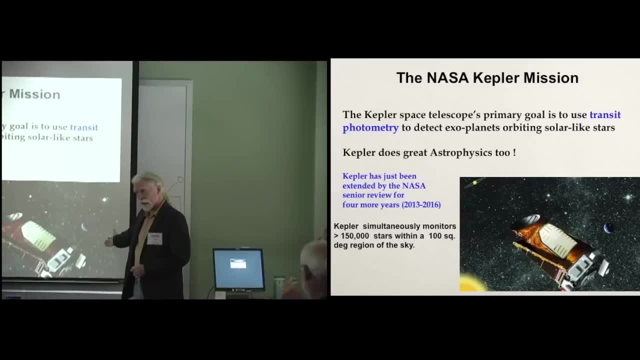 in and kill us anytime soon. all right. so kepler was launched three years ago- in two months or something like that, and this is what it would look like if you were out in space and stared at it just like that. so it was made to do really precise photometry to find exoplanets, but it also does. 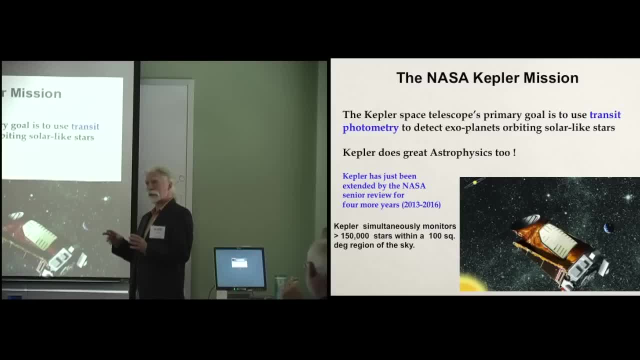 really great work on stars too, on astrophysics, not only on the planets, the stars orbit, but also on- uh other, i'm sorry, the stars- planets- but also on other stars as well. and we were just extended by nasa through the senior review process for another four years. 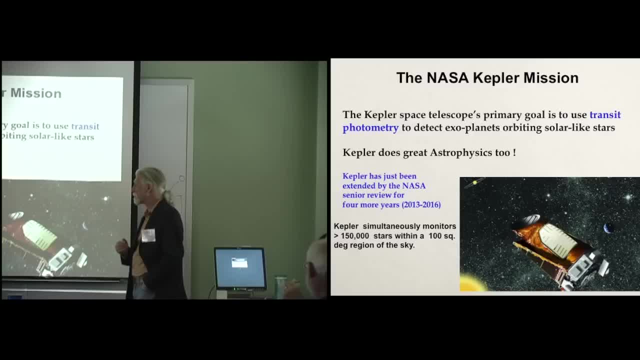 and that's very exciting news for us and for the parents. thanks a lot for all your help. so we it monitors 150 000 stars in 100 square degree region of the sky. so how many of you know how big 100 square degree region of the sky is? if you looked up, how big would 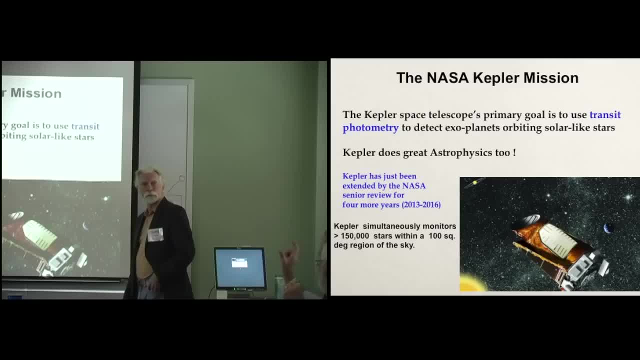 it be okay that big man got people like this, the hand, the old hand, right your hand, and arm's length about 100 square degrees. so as a homework assignment, if that's 100 square degrees, how big is the hubble field of view when you look up in the sky? so you guys can figure that out? i'll ask you after your answer. 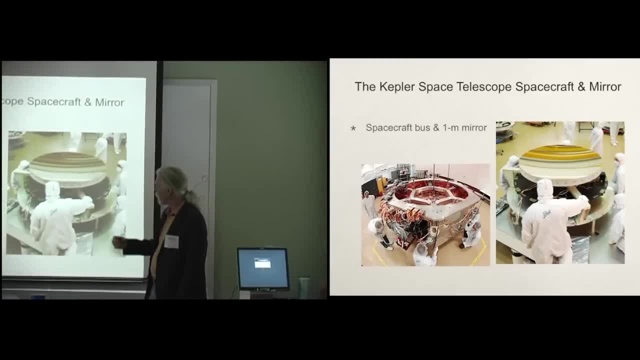 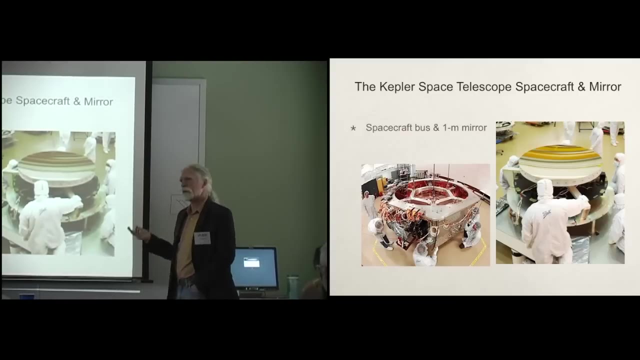 okay, if you haven't seen kepler, i know at least one person here used the working balls probably probably sold this before. so this is the spacecraft over here where the mirror will sit on top of this in the telescope. this is the one meter primary mirror. kepler is a schmidt telescope. a schmidt telescope is a great way to get a big field of view. 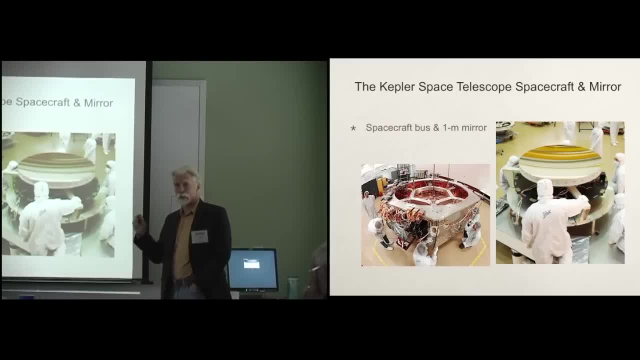 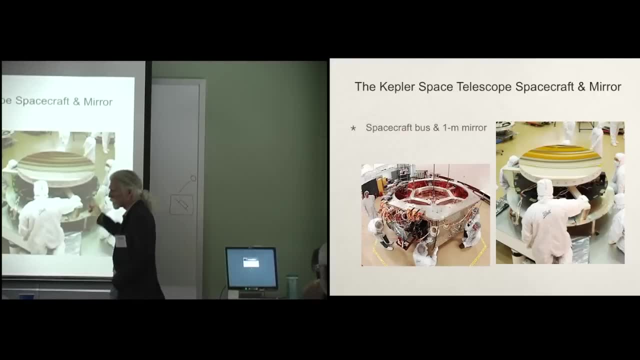 but it's not such a great way to get a really good plate scale or a really good arc seconds per pixel that you get a big field of view and for photometry you don't care so much about the plate scale. so this was the reason a schmidt telescope was designed and used. this is the imager. 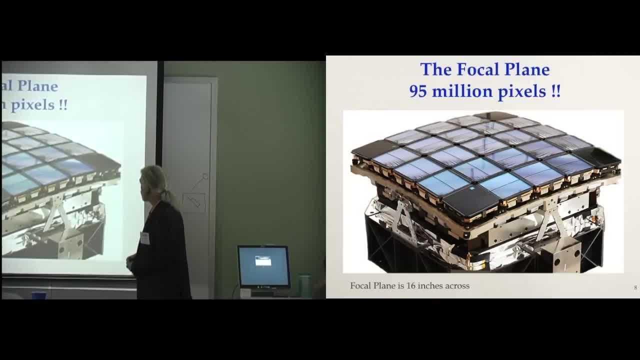 that kepler uses. it's an array of ccds, and this is the image that kepler uses. it's an array of ccds. there are 42 ccd pairs, and then in each corner there's a small ccd which is used for the. 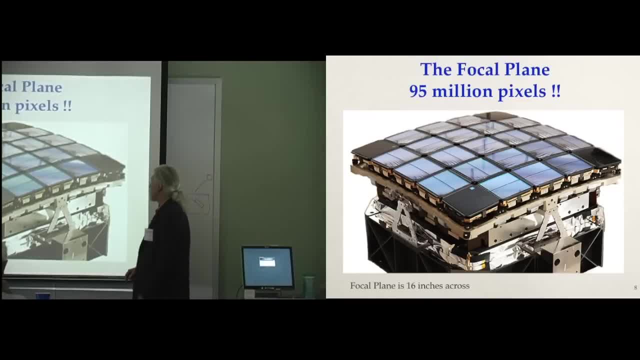 guiding of the telescope for the fine guidance. so these ccds are read out in five sections. there are five rows of them across here. they're read out using similar and the same electronics. there's a lot of crosstalk that goes on because all the electronics are sitting in this box right behind. 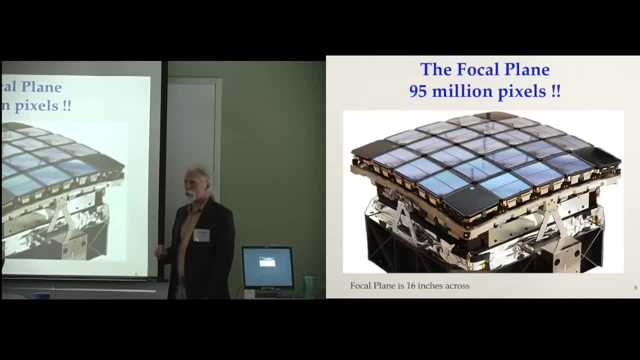 the ccds. so if you were to design an instrument with no crosstalk, you wouldn't design this instrument. this is the only way you can pack all the electronics into something that's small and can fly in the spacecraft and hide behind your focal plane. so you don't have any. 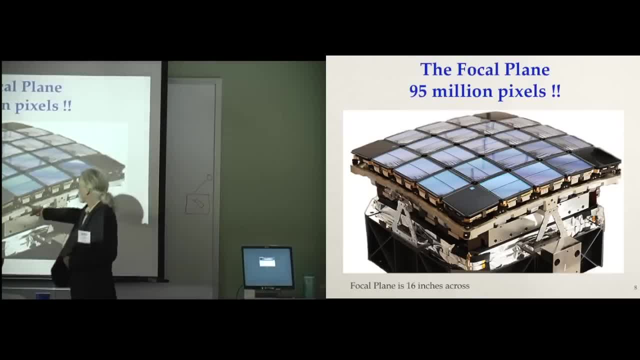 light losses and these small ccds here that are used for the fine guidance and kepler's, a really impressive telescope. you ever want a telescope? you know all aerospace does a pretty good job. so these, uh, we turn the spacecraft, as you guys know, to download the data and turn back. 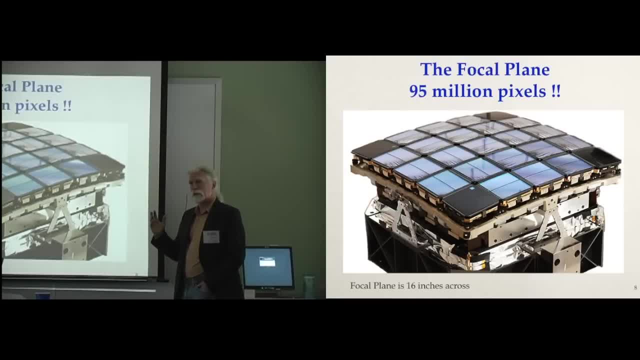 and it refines its position- points to within one hundredth of a pixel when it points back, and that is really critical for kepler photometry. it sounds like an amazing thing and why do you care? but that difference between one or, say, three hundredths of a pixel changes the photometry of a given star by two to five. 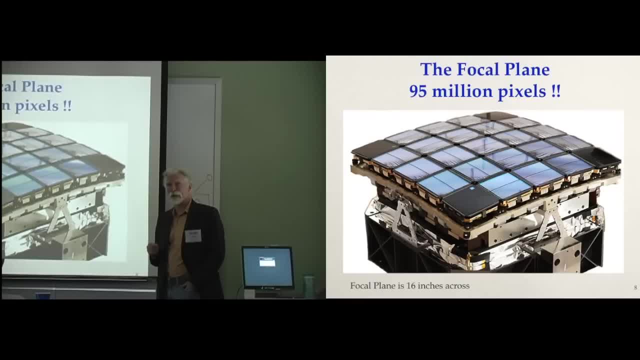 parts per million and we can detect that and that's bad because it looks like a transit from a very small planet and if we see these things, we go and spend a lot of time thinking about transits. that may end up being some little motion, so it does a really good job. 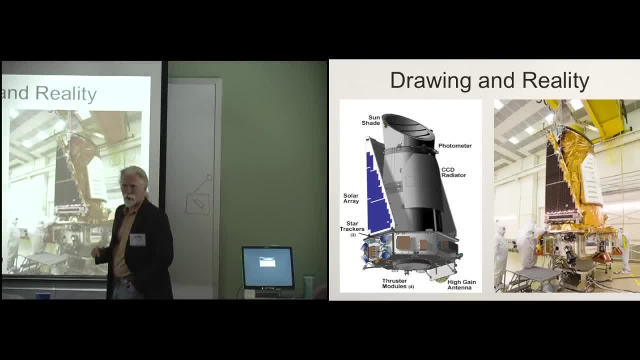 and this slide is one of my favorite slides and i show this in all my talks. if i can, even if i'm not talking about kepler, i throw this in. i think it's a cool slide because i remember that day and i remember that day and that's just really pretty cool to draw something up and then here. 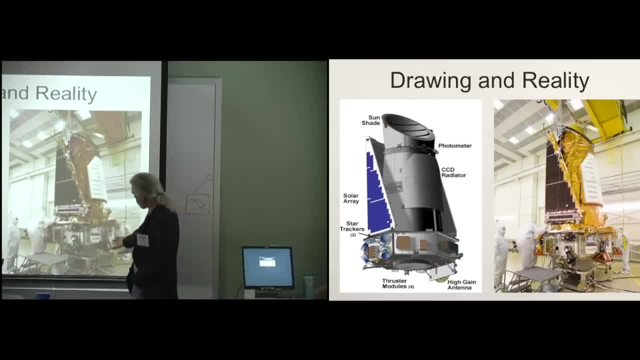 it is put together and at all. so this was the part we saw before. down here. this is a spacecraft which now has some extra stuff on it and this is the tunnel scope up here. this is the radiator to move away all the heat out in space from all those electronics, the solar panels, back here. 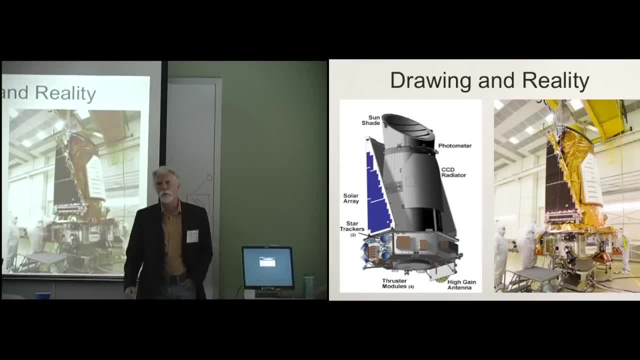 that are always pointed to the sun to give us our energy, and it's basically nothing but a schmidt telescope in there with that large focal plane sitting in the middle. so it's a very simple thing. kepler has one moving part in the telescope and that one moving part is the focus, and we never 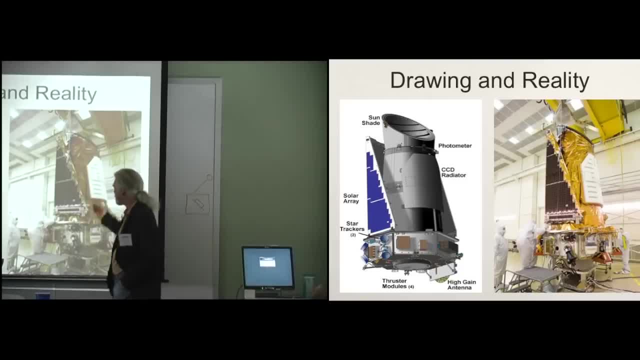 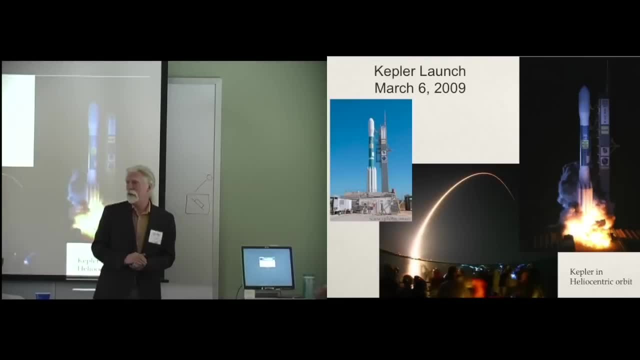 move it so and we probably never will. so it basically is a really, really simple design. that was very nice. this is the proof we really actually did it. We actually have a person who doesn't believe we were launched, so it's kind of fun This picture here. I don't know if you've been to a launch, but if you have, you don't see all that much. 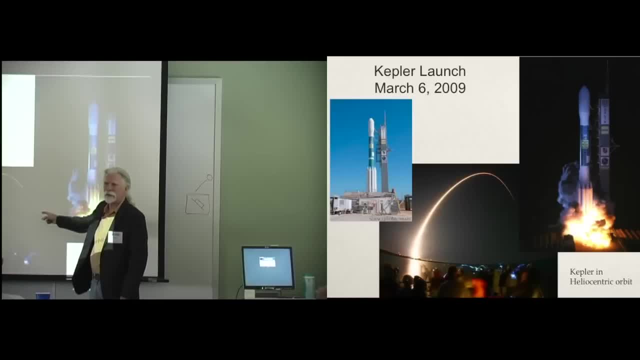 It's a time exposure, but it looks like it's going right down into the ocean. It's really not a great picture to show the public off. They don't understand. you know the curvature of the earthquake. Anyway, this is a lot of fun. Launches are always great. 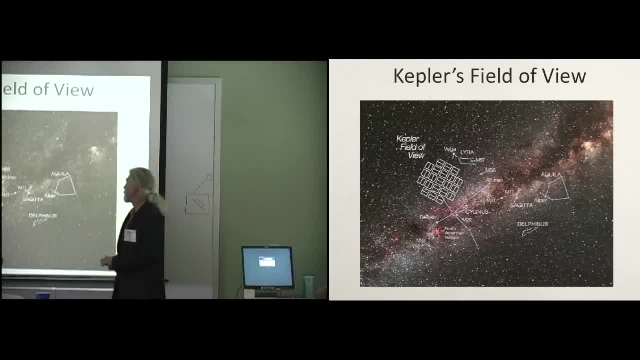 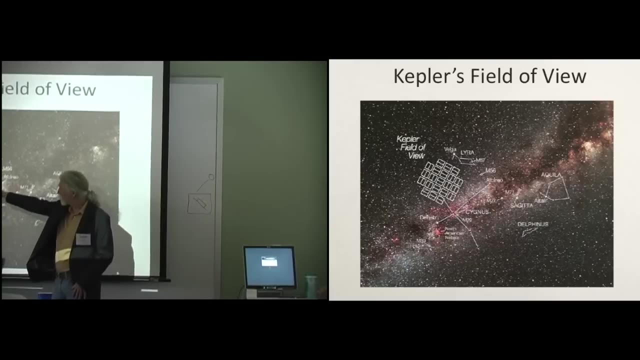 And here's the field of view on the sky. You know the constellations and all. We're looking at the constellation Cygnus and a little bit into Lyra. This is the Milky Way, if anyone's here- And Kepler's original field of view. these represent those 42 CCDs, those little pairs of CCDs. 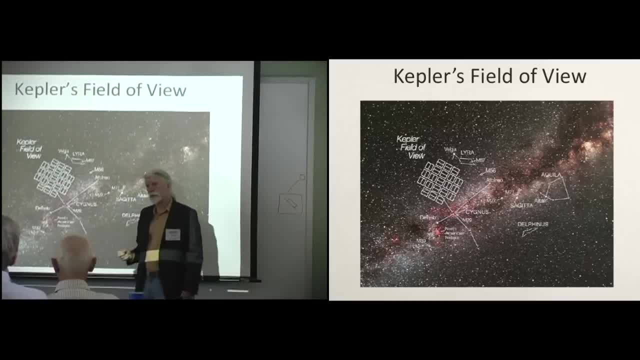 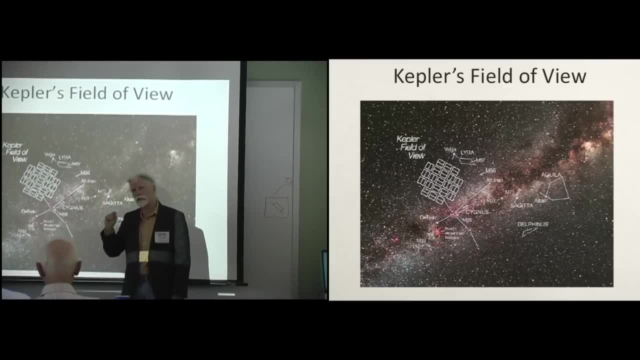 And you notice there's gaps in between there And those gaps are pretty big. They're about three degrees in depth. But the nice thing is- and you can't tell so much from this picture- but a lot of the very bright stars purposely were made to fit in those gaps. 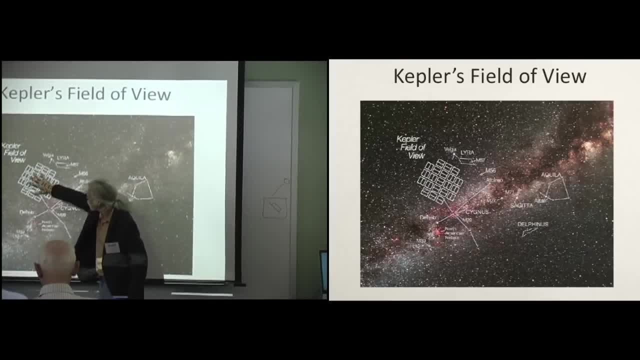 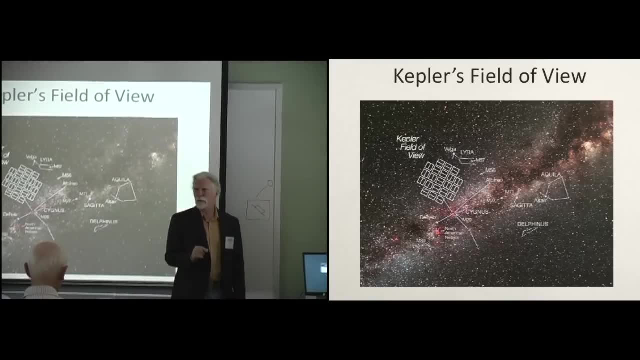 so we don't image these very bright stars, But the original field of view was that orientation that was sitting about here. And it was sitting here because originally it was thought where you can get the most stars is looking right at the Milky Way, because that's where most stars are. 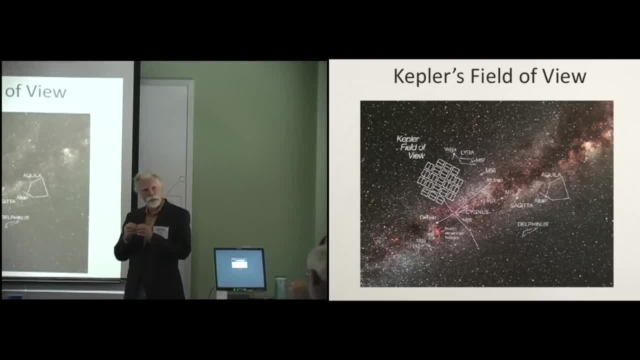 But unfortunately, if you look right at the Milky Way, blending of stars is a tremendous problem. There are just so many stars and every star is blending with some background, And disentangling a background variable on a transiting exoplanet would be nearly impossible. 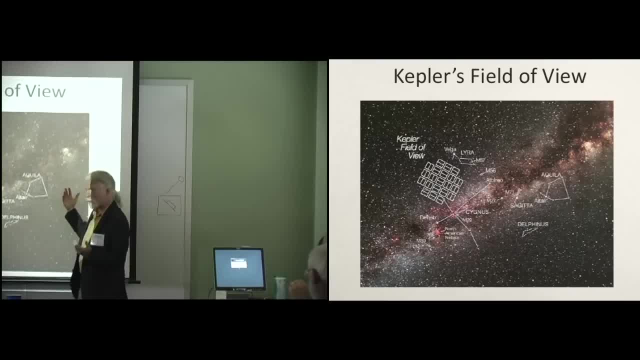 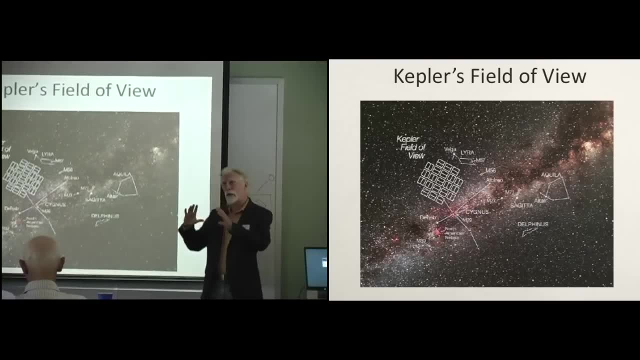 The other thing you know if you see this picture of the Milky Way or know about the Milky Way, there's these dark regions in there, this dust that hides stars in the background. So by putting it right on the Milky Way, you're actually losing stars as well. 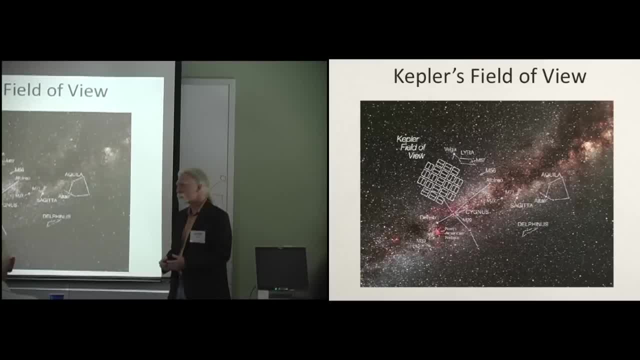 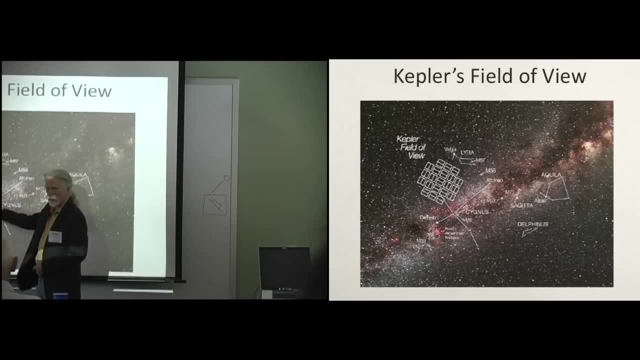 because this dust hides a lot of background stars. So we pushed it off about five degrees off the Milky Way and now we have a sampling of a very high density region down here and a fairly low density region up here. In fact, a lot of the stars up in here are giants or stars that are in the old disk or the halo. 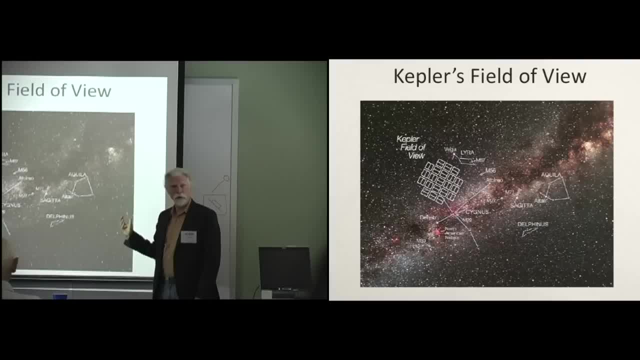 So it works out really nice to have this field move, because we also can look at the planet distribution as a function of different kinds of stars in different locations in the galaxy with different metal contents. So it's kind of a good thing for many reasons. 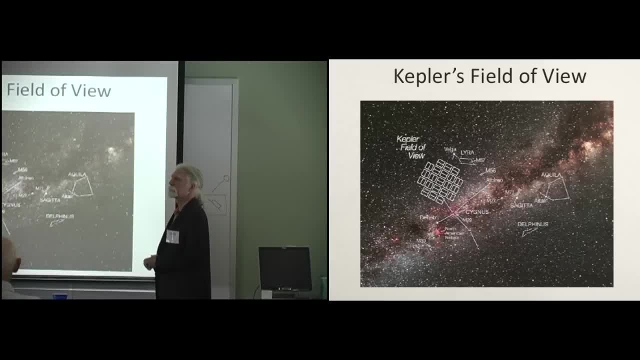 Was the field positioned to turn in before launch or after launch? Before launch: So you figured all of this out before We did. yeah, And it's the only field of view we've looked at and chances are it will be the only field of view we'll ever look at. 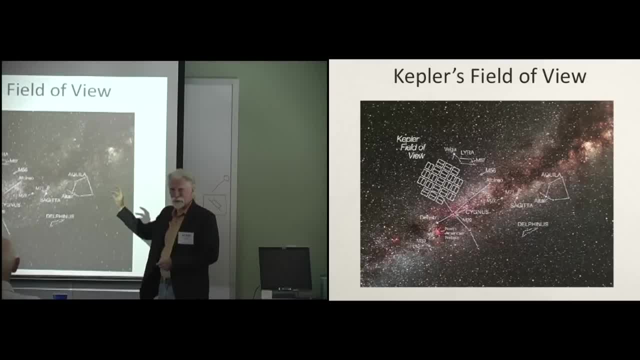 This field of view is going to become the most studied part of the sky. It hasn't already? Every satellite, every telescope has studied this or is studying this, So it's going to have multilayering data across everything. It'll be pretty amazing. 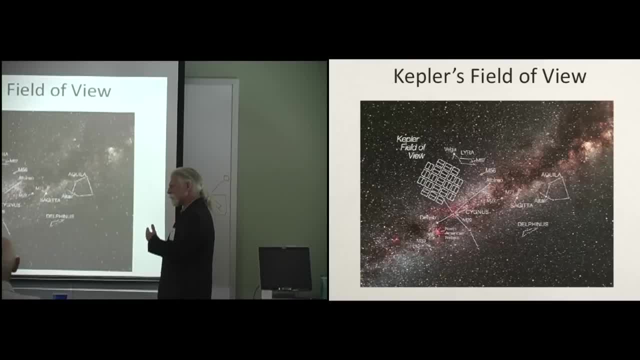 Maybe we'll learn something from that. So the field of view had two choices. They were easy to do. One was in the northern hemisphere, the northern sky. The other was at an equivalent point in the southern sky, But we chose the one in the north. 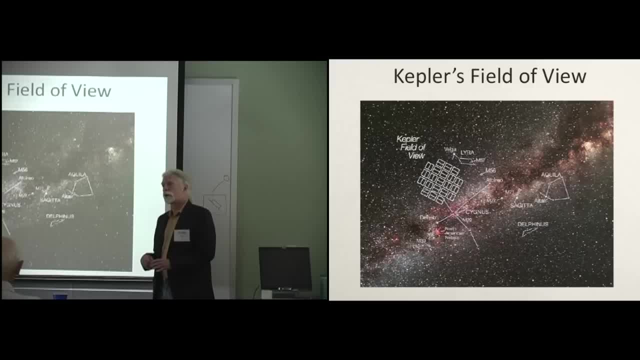 because most of the people that worked on the Kepler project worked at or for observatories or universities in the northern hemisphere and they could get access to northern hemisphere telescopes to do a lower ground-based follow-up and help us understand the stars and the planets. 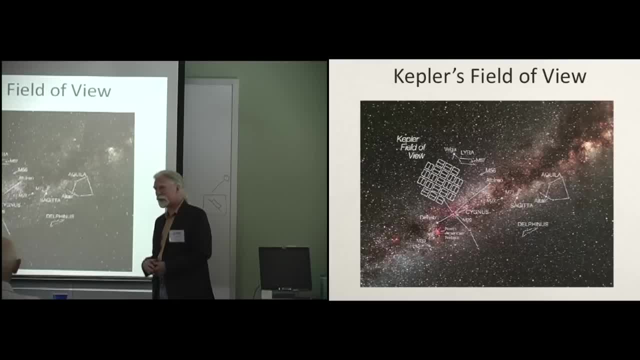 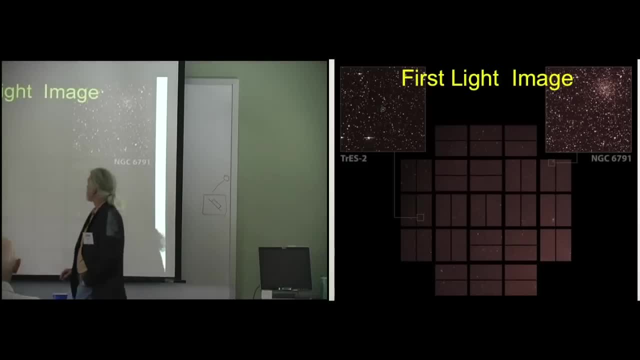 And in the southern hemisphere we would have had a little more difficult way to do that. So that's kind of how it worked. Okay, and here's the Whoa. that's pretty awful. It doesn't matter, It doesn't look very good anyway. 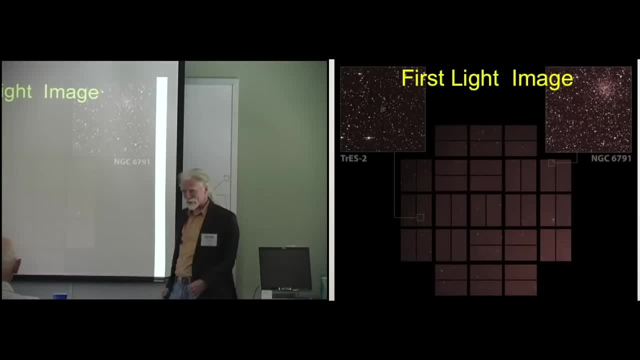 This is the first light image. If you go over by the mock, there's a great poster of the first light image that looks just like this. So I really just didn't want to show you this image, except to show you that there are open clusters. 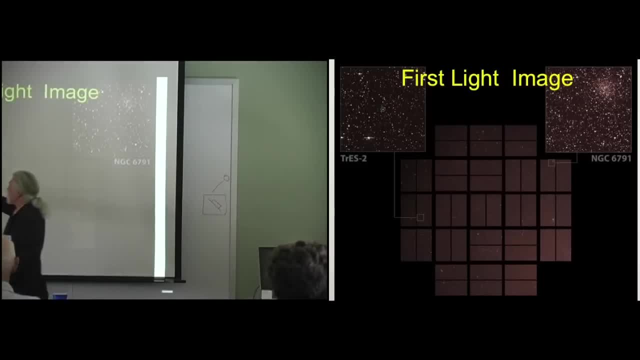 You can kind of see that's an open cluster over here And this is TREZ-2.. This is a hot Jupiter. It was known before Kepler was launched. It happened to be at Alistair Field As soon as we were at Alistair Field before launch. 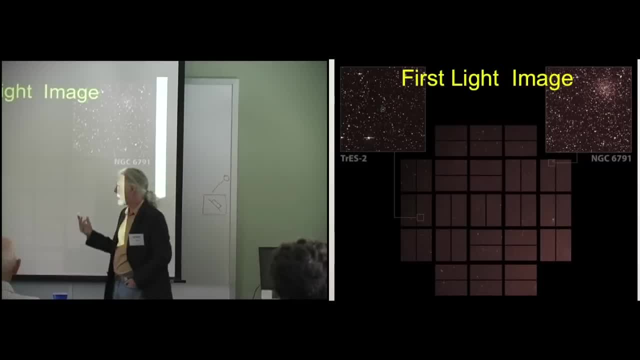 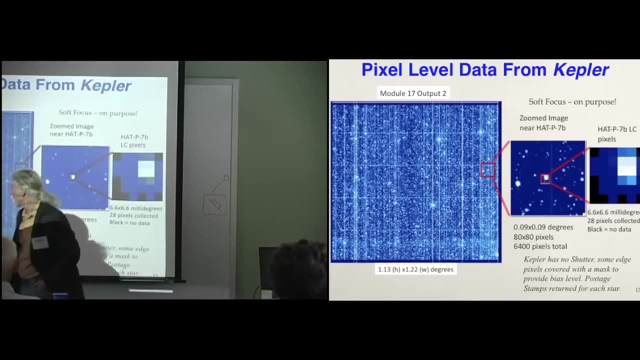 everybody who was doing planet surveys started studying our field of view, And I think four planets- three or four planets- were found on all hot Jupiters before we launched. But what I do want to show you is this image. So this is one of those CCD modules. 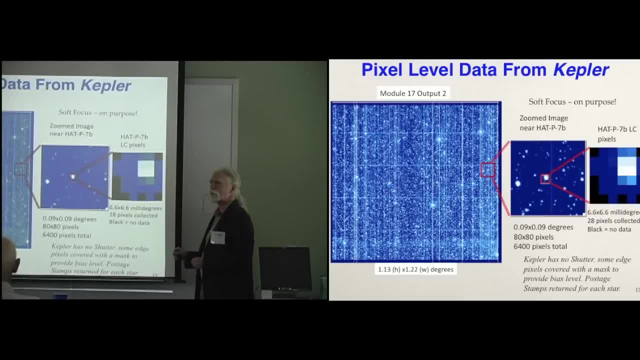 And they all have numbers and names. It says 17 output 2 here in the lingo, And if you took an image like this at a ground-based telescope, you would just think the instrument was a piece of junk And you wouldn't ever use this thing. 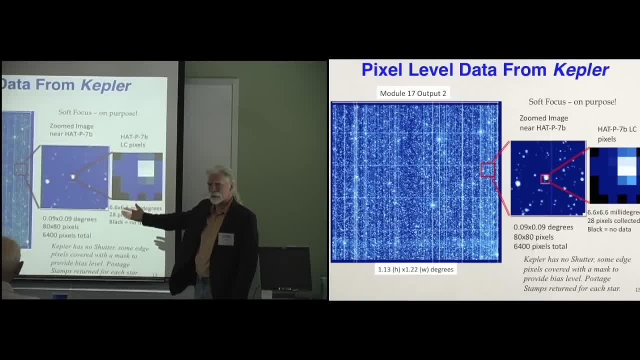 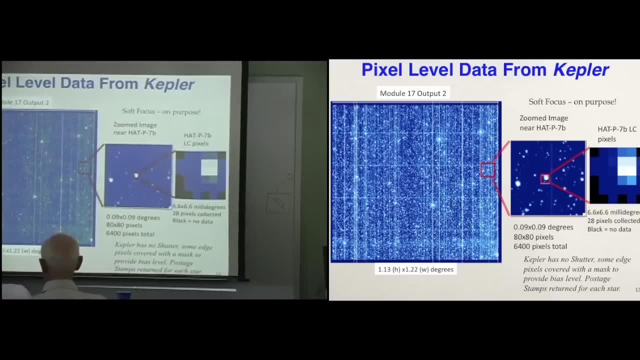 You would go and complain to the director and say, look, this is a piece of crap. But what you don't know is: this isn't a piece of crap, This is good stuff. So Kepler has no shutter. Sorry, I can't stand it, I can't see. 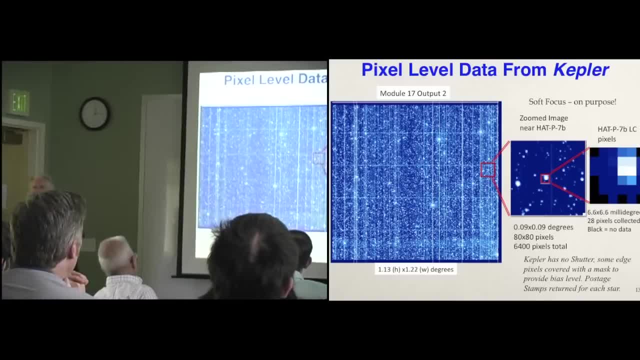 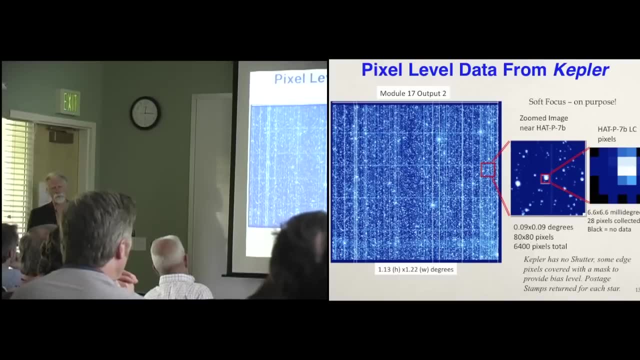 Kepler has no shutter So it's just read out continuously. We integrate for six seconds, We read it out And we store 150,000 plus about 20,000 more little postage stamps around the stuff. We don't store everything. 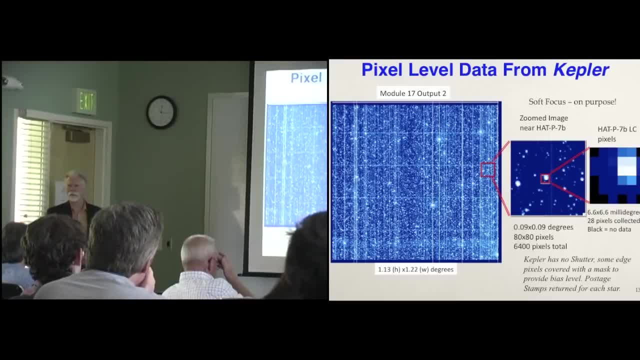 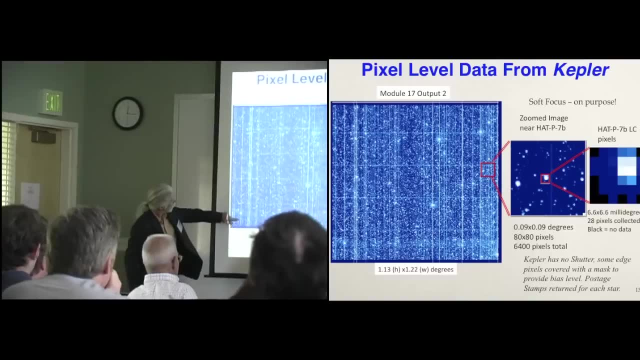 We read it out again, And we do that over and over and over And co-add the data either in one-minute samples or 30-minute samples- Many more 30-minute samples than one-minute samples. But all of these long streaks are these bright stars that just bleed all the way across the CCD. 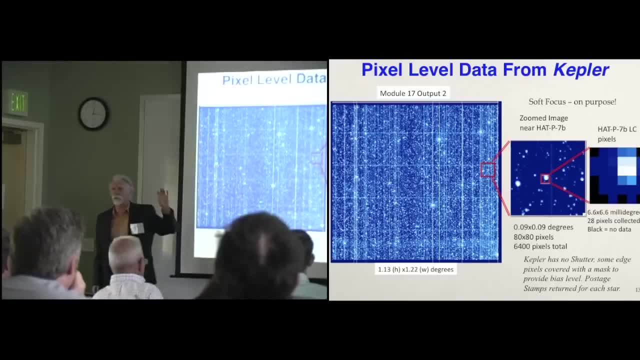 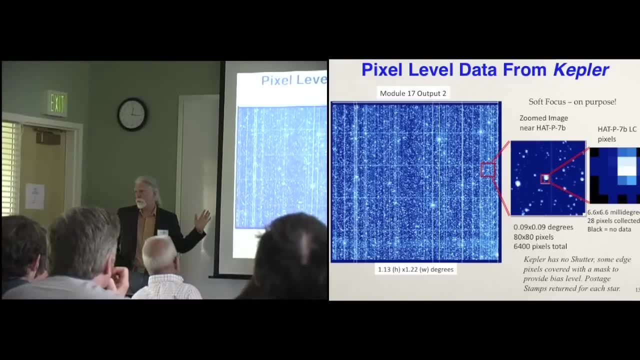 And you see, every one of them is associated with a bright star And these stars break. These might be fourth magnitude to eighth magnitude, So they're pretty bright stars even for such a short exposure, But the nice thing about it is that bleeding is incredibly constant. 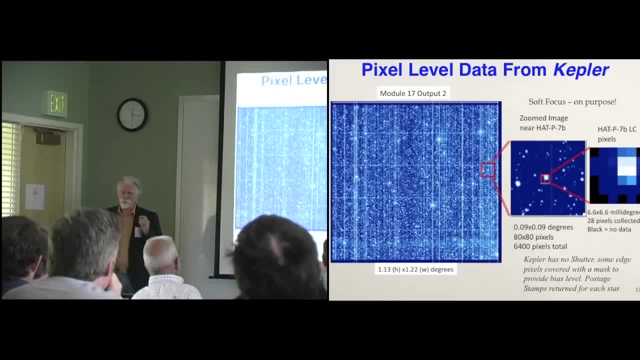 So you can remove it, Or in fact, you can do photometry on it. We now have just found- No, I can't say this, We may have just found something which might be a planet orbiting a star that's brighter than that object. 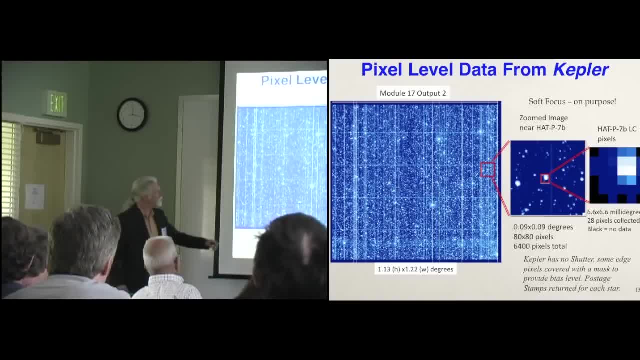 which just bleeds tremendously across. And all you do is you just add up all those pixels, Because all the light's there, It just is spread out over many, many pixels And you add it up and you get a great light curve. 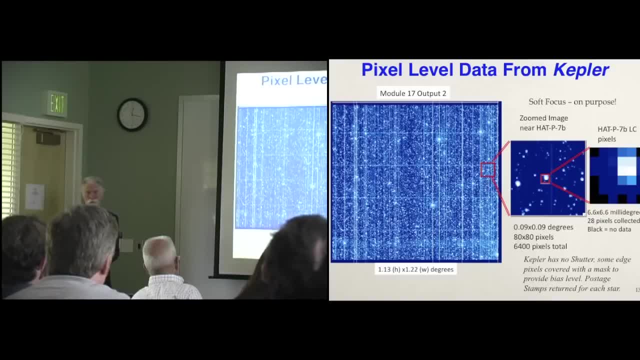 In fact, it's really fantastic because your signal-to-noise is phenomenal. in that kind of light curve, You also can see lines going across this way. These are those lines of crosstalk between other CCDs that are reading out at the same time. 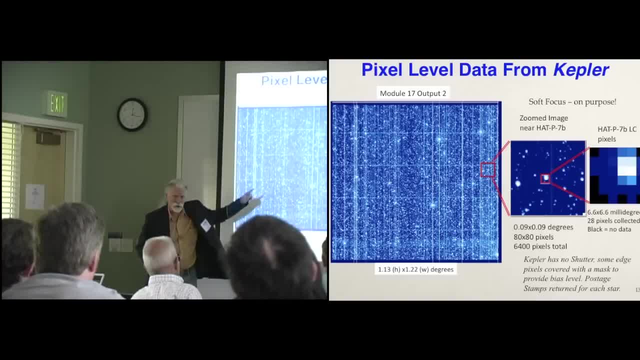 There are also lines that you can't see in here that have these sort of diagonal stair-step shapes, And those are crosstalks from the guide, CCDs reading out. At the same time the science CCDs are reading out, But again, all of that is constant. 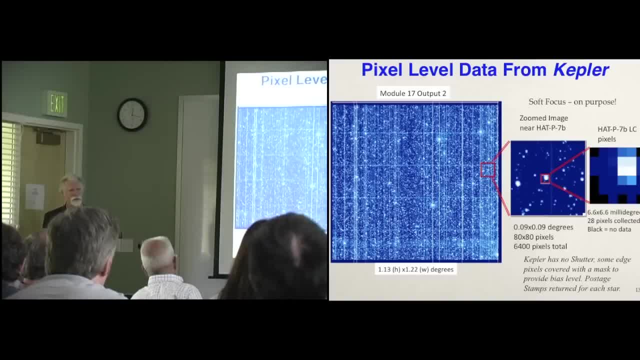 It has exactly the same time all the time, Exactly the same level. You just remove it all and you get an image that looks like this. So this image over here is the same stretch as this image over here, So I'm not trying to pull one over on you by hiding all the crap in the background. 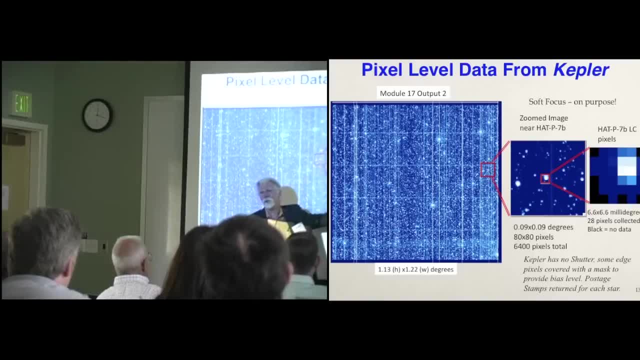 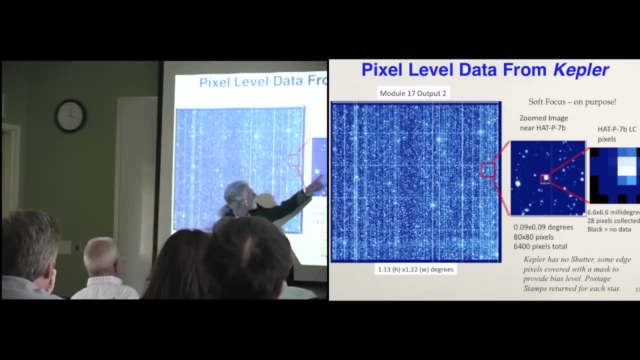 And you can see now, the background here looks pretty smooth. You'd like this image, Except you'd say, Oh, the focus is pretty awful. Look at that. All the stars are squares And if you blow it up, that's what they look like. 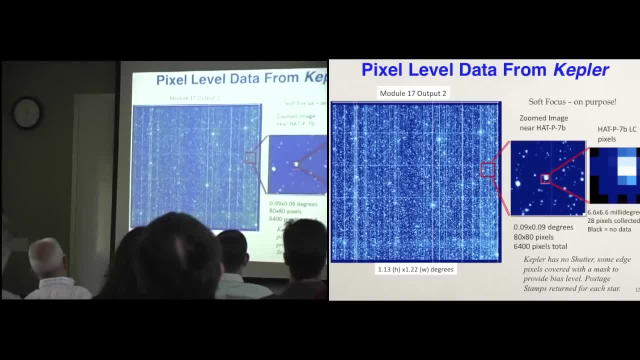 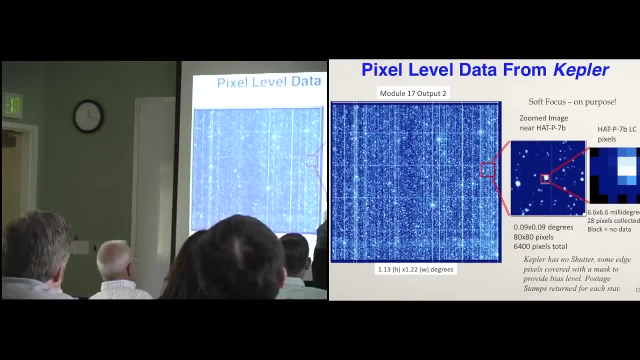 Kepler's pixel size on the sky is four arc seconds in one pixel. So this star here you can maybe kind of tell these two grays are a little less than those. So this has something like a full-width half-max of a pixel and a half or something. It's like six arc seconds. You're in space. Six arc seconds. It's nutty. Well, it was done for two reasons, And they both actually turn out to be the same reason. If you have a Schmidt telescope, that's perfectly in focus. 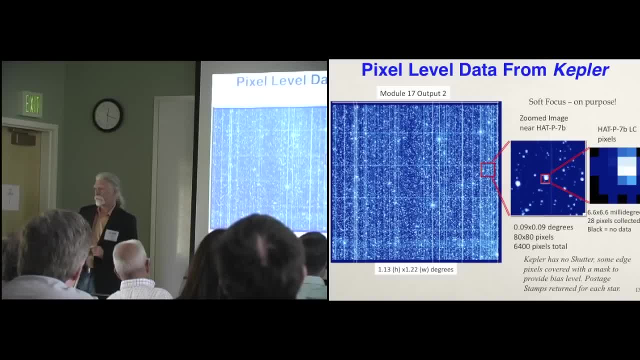 you make a star shape, the point spread function, we call it. that's very spiky And then it has very broad wings And if you know anything about doing photometry, you never want a star to look like that if you want to do accurate photometry. 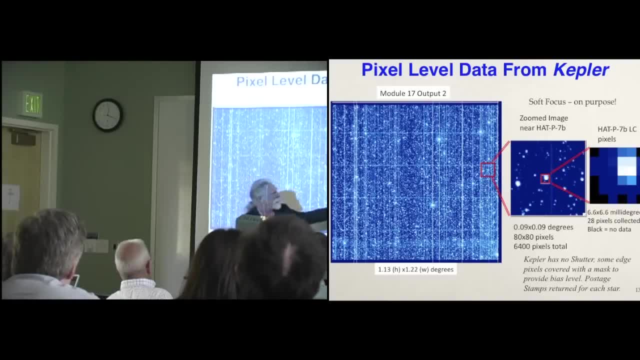 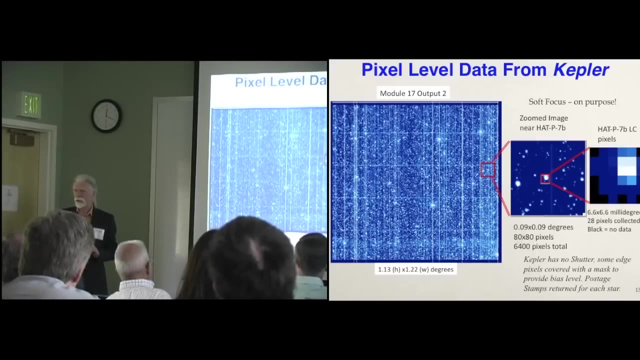 The reason is that sharp peak falls inside one of those pixels And, as the spacecraft jitters- albeit very little, maybe one one-hundredth of a pixel- that peak moves around within that pixel And the quantum efficiency of a pixel is not constant across the pixel. 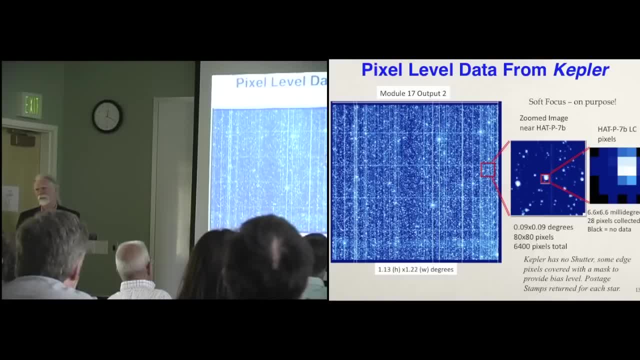 Within one pixel. it changes by a little bit, But at these levels of precision that would matter. So you want to blur your star image, You want to blur your point spread function, And so we purposely do that. It's a soft focus, purposely. 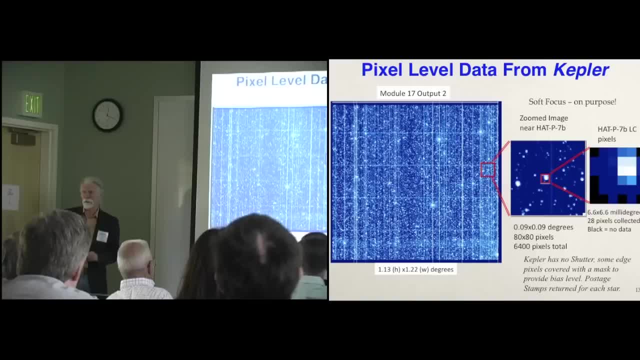 So, unlike Hubble when it was launched, that had a soft focus, not on purpose, we purposely have a soft focus. Now. that's bad in the sense you can't show any pretty pictures because they all look like that or they all look like that. 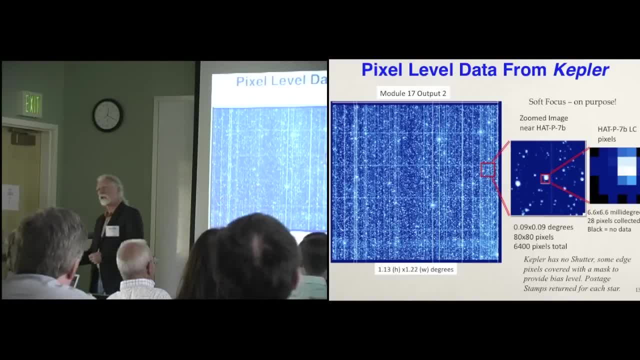 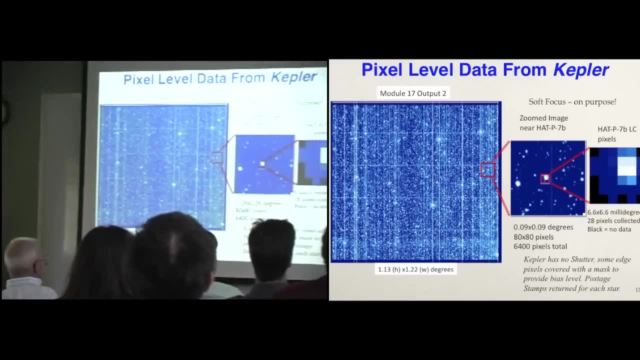 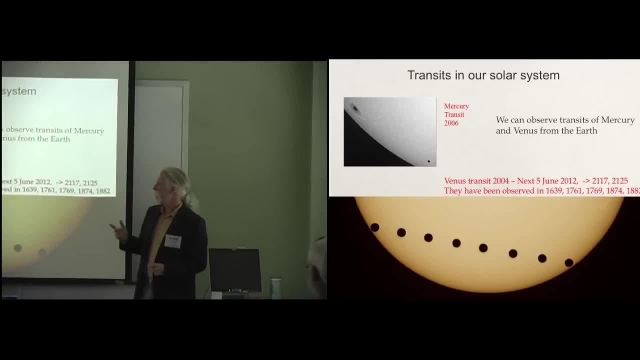 So you have to kind of change your thinking and show a beautiful light curve and get all excited that that's a pretty picture. You'll never see light curves as good as Kepler. So let's talk a little bit about how Kepler finds planets. So how many of you saw the Venus transit in 2004?? 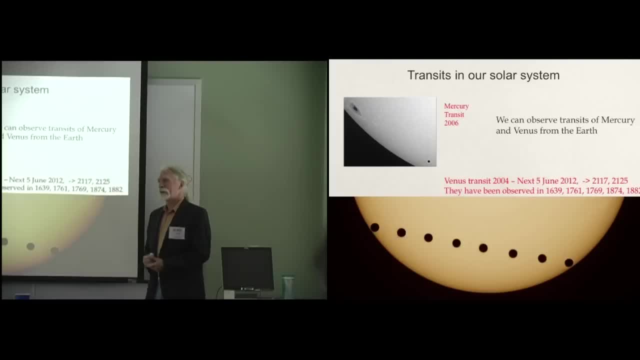 Anybody. Excellent, Wasn't that cool? Okay, so you were acting just like Kepler. You see Venus go across the sun and you can detect it. Now, that's not quite true, because you can resolve Venus on the surface of the sun. 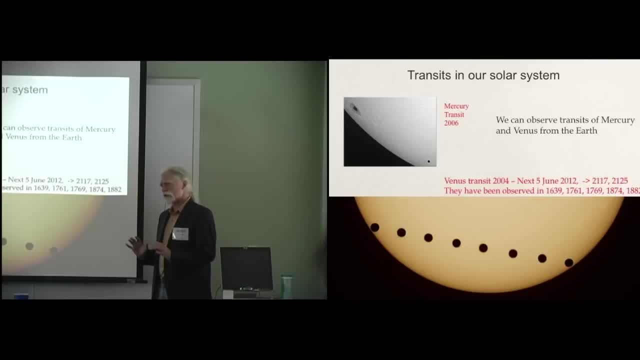 It's hard, It's time, But you can do it. Kepler cannot resolve the planets going across their stars, But he can see the drop in light that that planet blocks out as it moves across the stars. It's pretty amazing that he can. 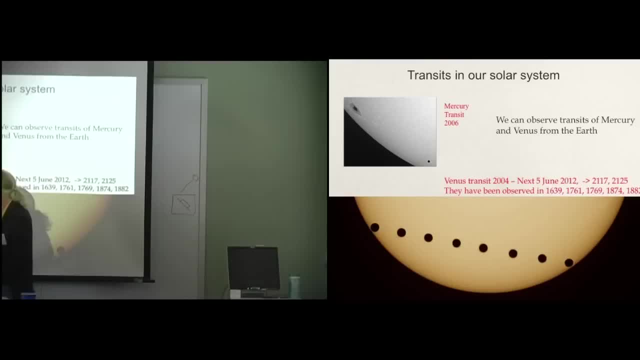 So this is Mercury, This is a real Mercury transit And this is a time lapse of Venus. And if you don't know, June 5th this year is another Venus transit. Some of you are young enough. You can wait for the next one in 2017.. 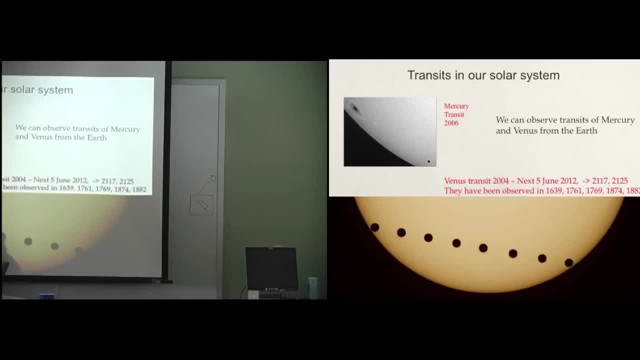 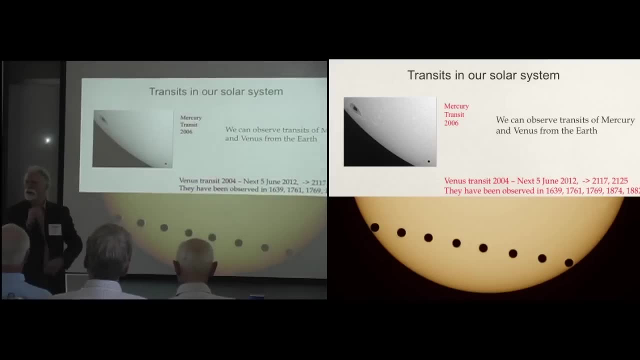 There you go. Don't worry about the one. this year We've got another one coming up. So this is what Kepler does: It finds transits, But again, it never can see this. It sees the star as a dot and it can tell about this little bit of light that gets blocked. 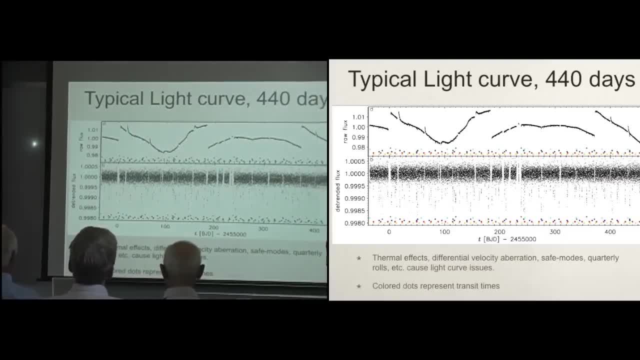 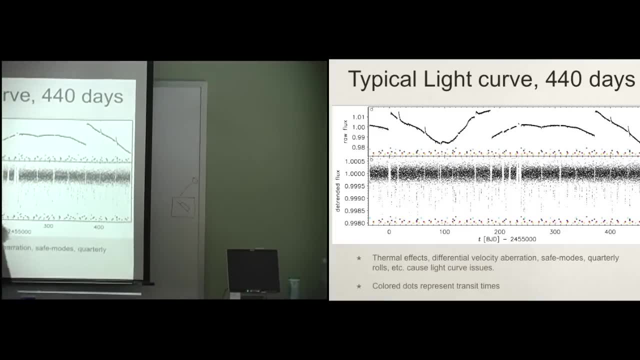 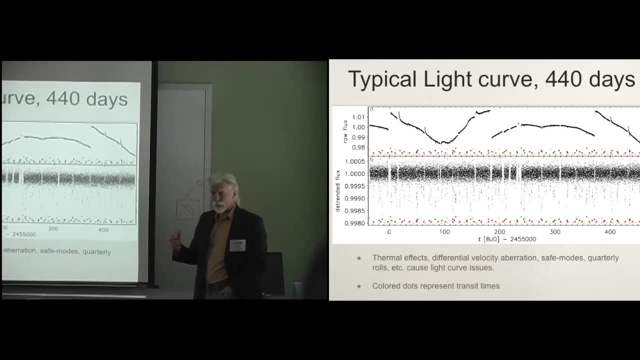 So here's a light curve. On top is a raw light curve that comes from a set of pixels around a certain star. Each of these chunks is there's four of them showing up. here are these so-called Kepler quarters, So each of these is a three-month chunk, roughly when Kepler's pointing at one orientation. 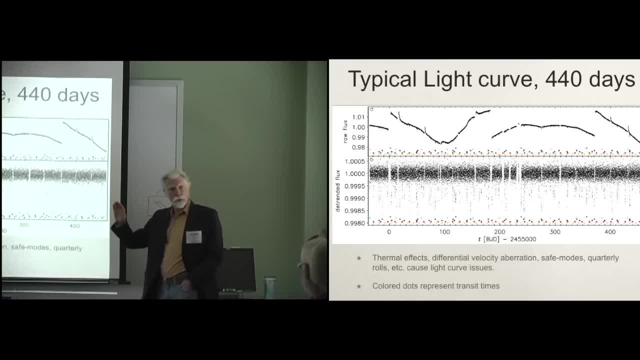 After three months it rotates by 90 degrees. But if you remember that focal plane, it's symmetric to rotations. So you rotate by 90 degrees to keep your solar panels pointed at the sun. Your stars are pretty much the same stars, but now they fall on different pixels, on different CCTs. 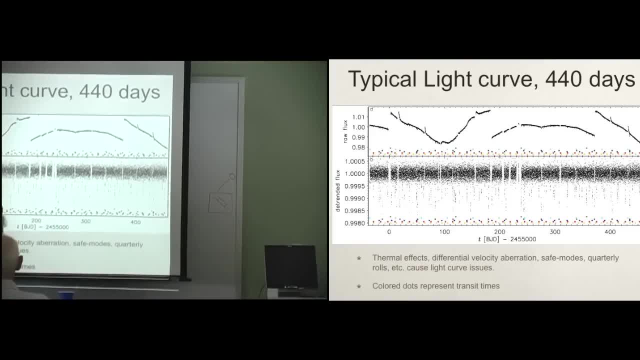 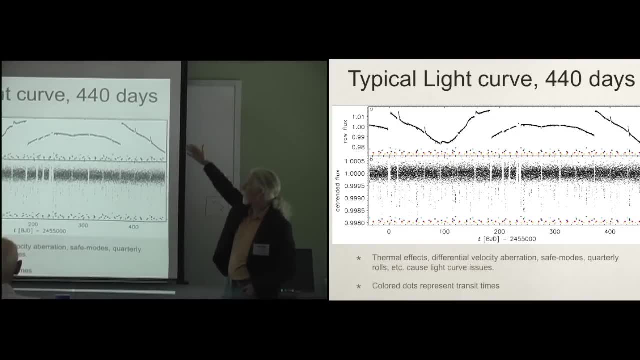 So what happens is this star: when it moves to a different set of pixels, it changes by a percent or something in its flux, up or down. They don't all go up, They don't all go down. In addition, there are these drops here that you see. 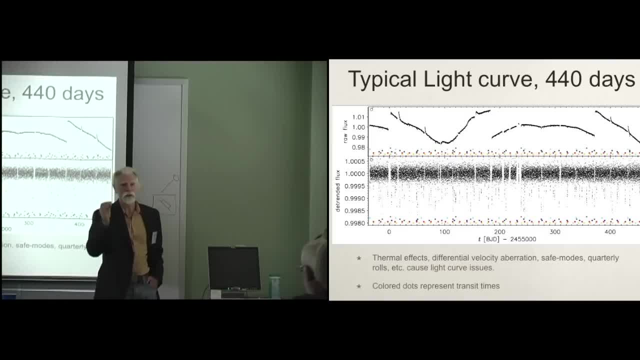 Those are thermal effects where the CCT changes its temperature very slightly and it takes a while to equilibrate, And that changes the expansion of the telescope And that changes the actual star range. It gets slightly bigger or slightly smaller And this is what happens. 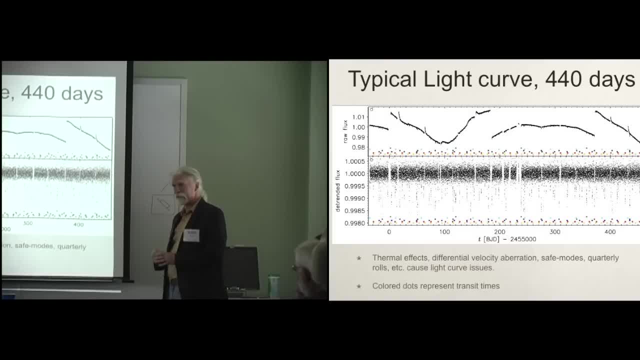 This is slightly differences here, But that's maybe a half a percent, a third of a percent or something. So the things we notice, So this is what we get out of the spacecraft, This is what we get from the pipeline once we run some magic on the pipeline. 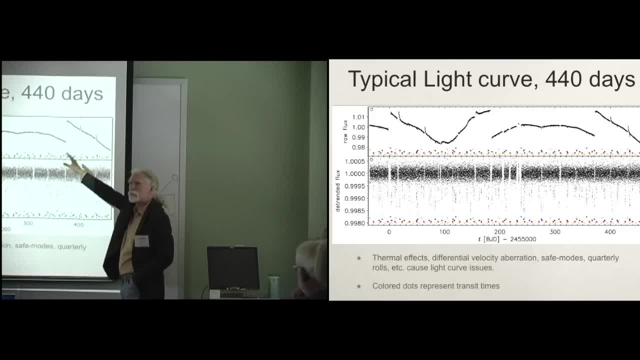 So you take that you basically stitch it all together, try to remove the artifacts. We know a lot about them. now, Again, they're all pretty constant. We know how to deal with them And you get a light curve. that's like this: 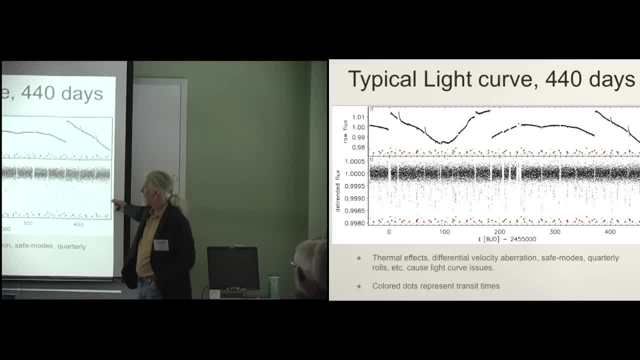 And I think this is pretty easy with your eye to see the planets here. This happens to be a light curve of a star with multiple planets. You can see some of the transits here match up in their depth. It's kind of like a puzzle when you see a light curve like this. 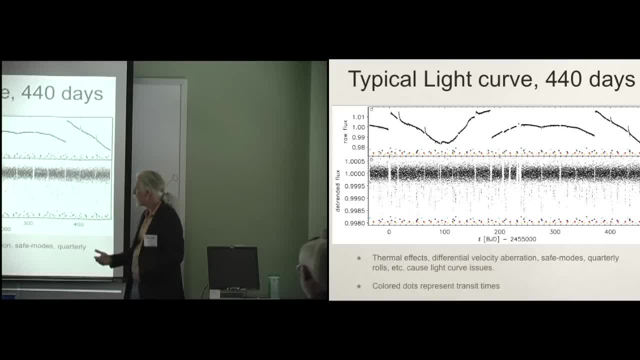 Which transits match with which other ones? What's the period where the planets meet? I think this has five planets in this particular one. So here it's pretty hard to see them, But here it's pretty easy, And we don't look at every light curve by eye. 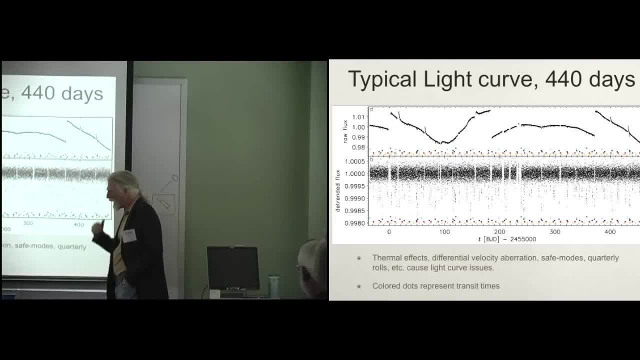 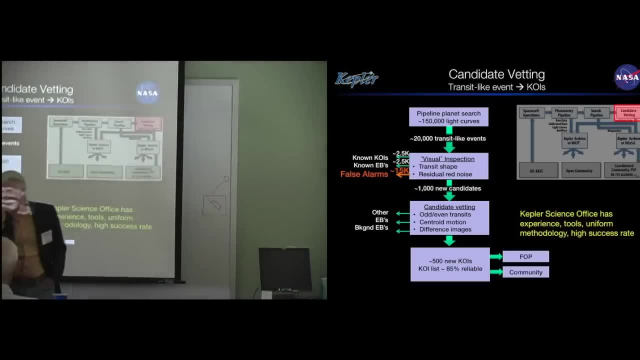 We used to. There's a lot of light curves, We learn about them, We know how to do it better, So we can just run this through And let me tell you a little bit about this sort of sausage process of how much work is done. 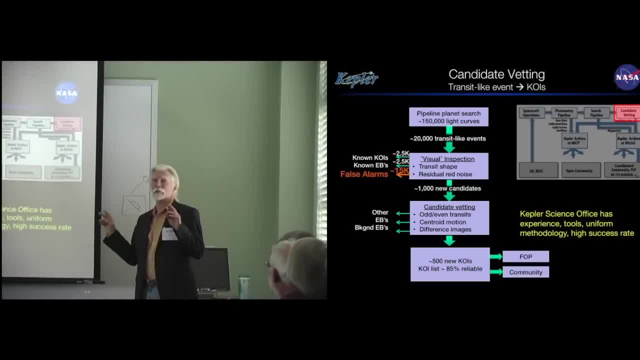 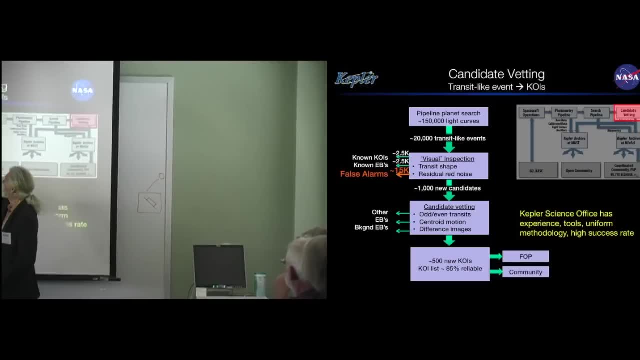 Unfortunately now it's mostly all done, as they say in software. So if we start with a typical search of one quarter of data, so a three-month chunk of data we find from the 150,000 light curves. so we're looking at 150,000 stars. 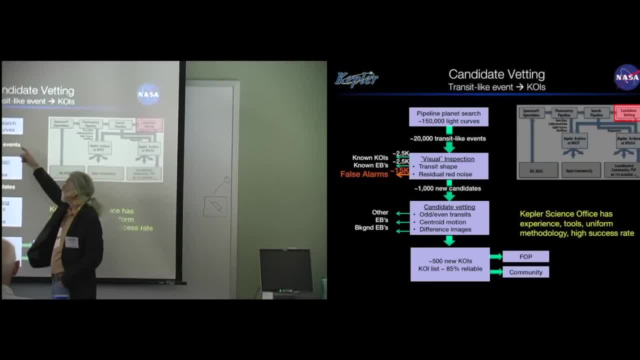 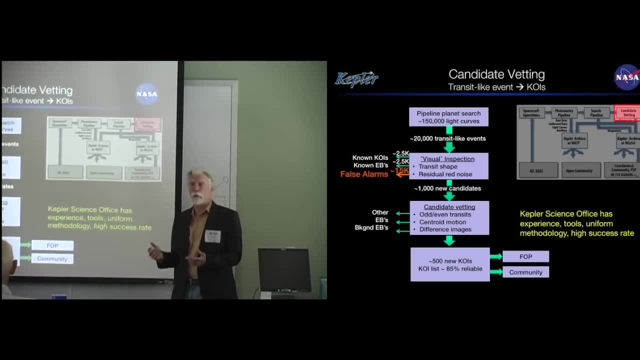 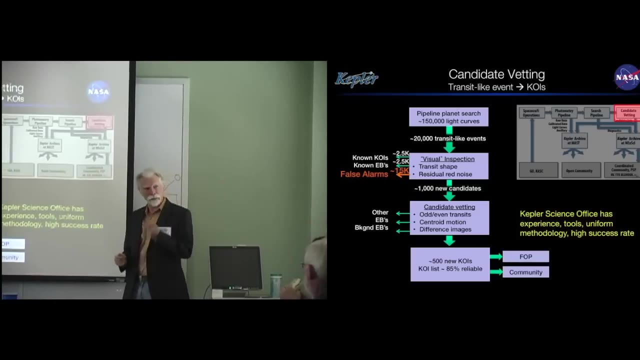 most of them sampled every 30 minutes. we get about 20,000 events that look something like a planet transit, So that's a pretty high number. So the first year we would literally look through 20,000 light curves And we had each light curve looked at by at least two people, just to make sure. 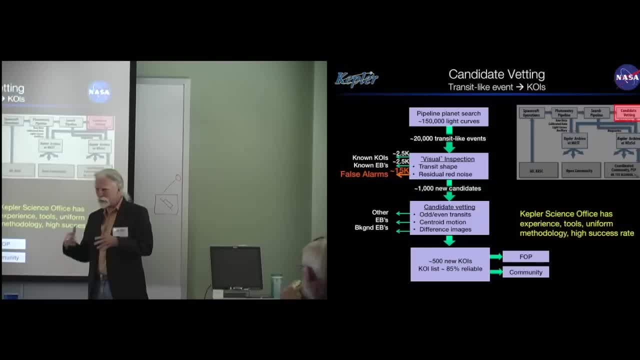 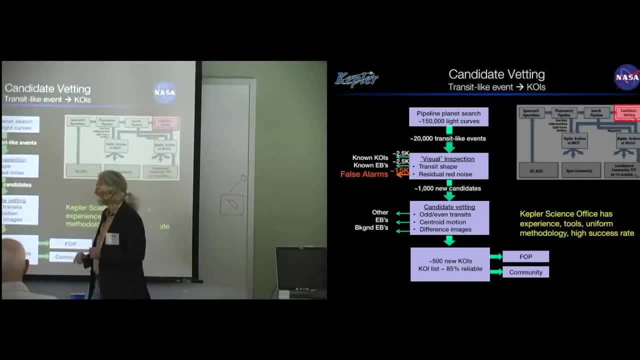 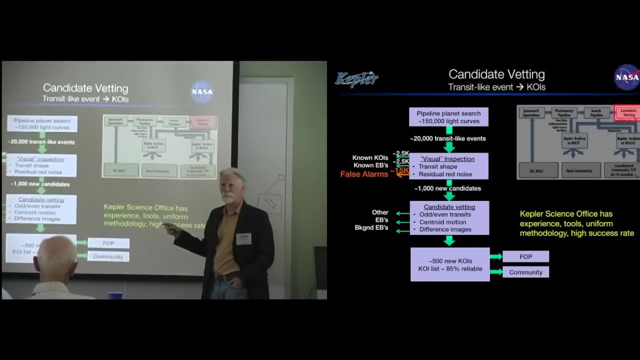 Now we look through maybe 500 light curves that are weird for some reason. So of these 20,000 events, this visual inspection, visual analysis, which is mostly done by computer, finds that something like 2,500 of them are already planets. we found the last time 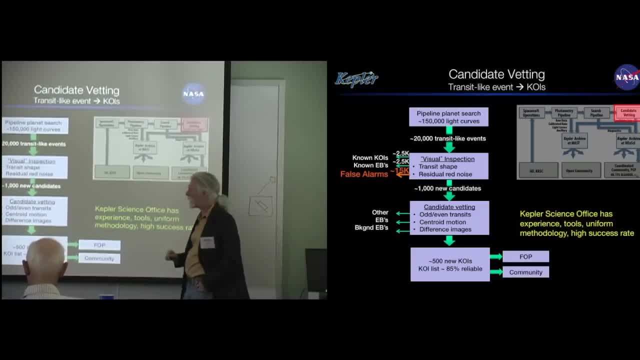 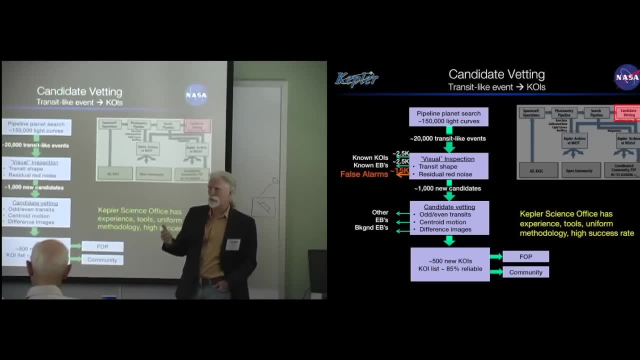 So that's good, We feel good, We pat ourselves on the back and push them off to the side. Something like 2,500 of them are eclipsing binaries that we mostly already know about. That's good. We found them again. 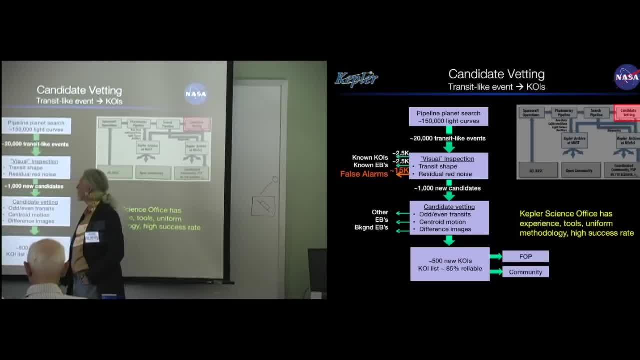 Something like 15,000 or so of those things come out to be false alarms, So they're not really a planet transit, And false alarms can be all sorts of things. The largest false alarm is literally just something that's junky data. 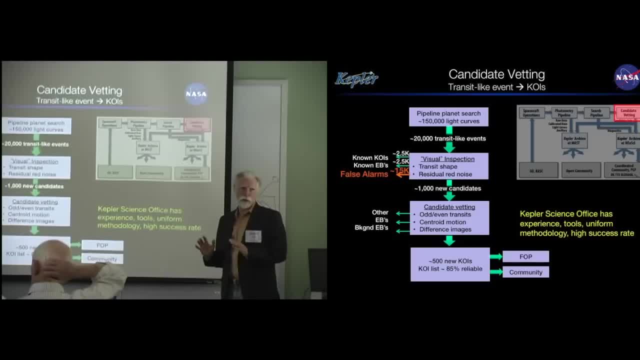 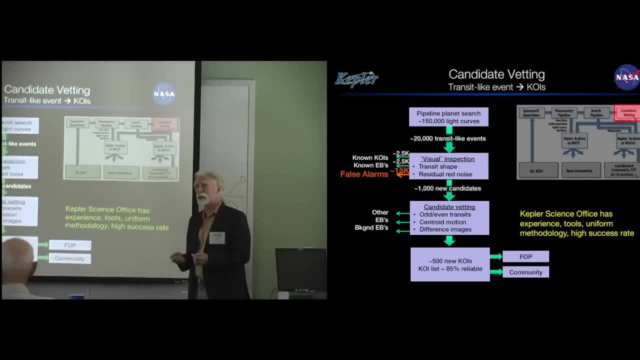 It's a cosmic ray, It's a bad pixel, It's something that's not real in any way, And so those are hard to throw out, because they often look like something. We're talking about 10, 15 parts per million signals here. 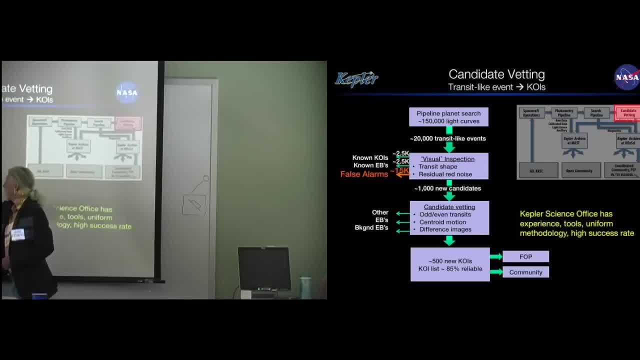 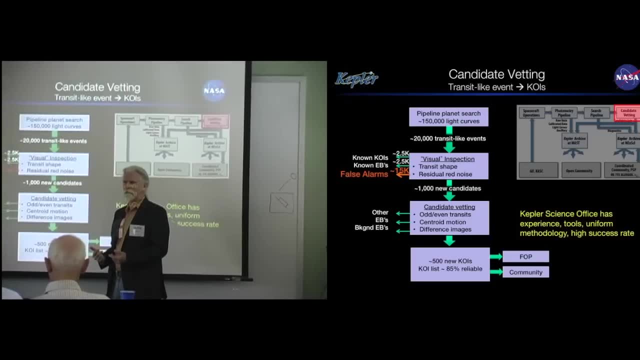 It's pretty tough, But again we're doing pretty good. now to throw these out. We use other things like the shape of the planet transit, The shape we believe We got fooled on that actually with planets that orbit M stars. If you know something about a planet transit that orbits something like the sun. 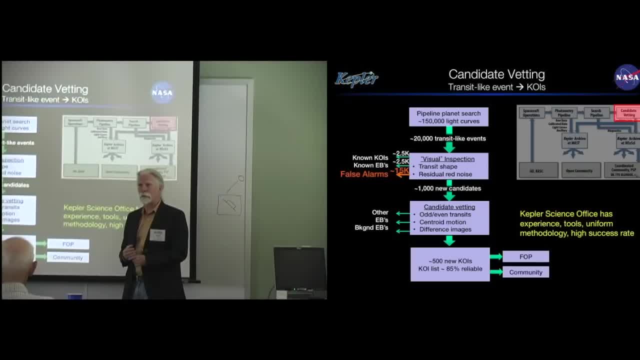 it has a U shape to it. I'll show you some beautiful examples here in a moment. If you have an eclipsing binary, it often makes a V shape- eclipser transit. So we thought this is easy: U shaped planet, V shaped eclipsing binary. 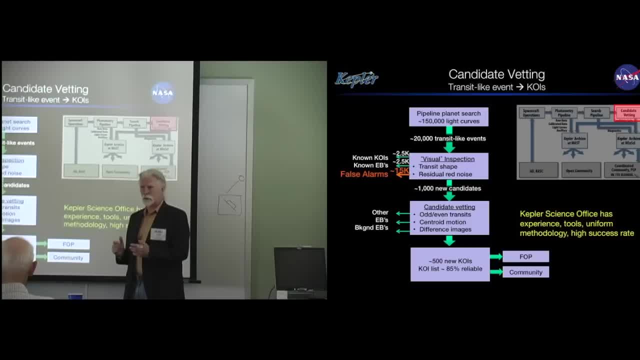 Well, take yourself a nice model of an M star, a really cool M star. lots of limb darkening and some spots on it. You run a planet across it and all of a sudden, the planet transit looks like a V shape. Wow, there's a surprise. 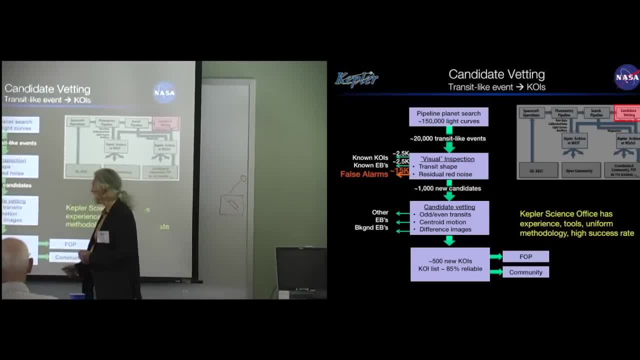 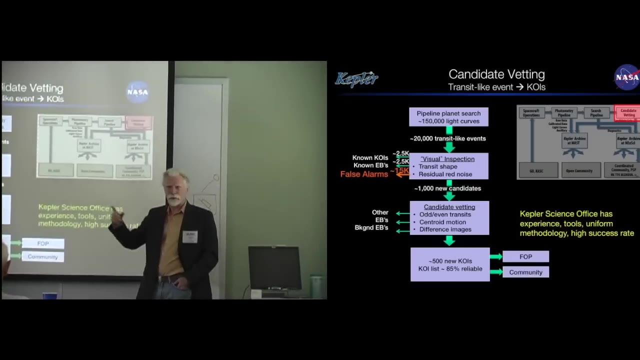 So you learn here. It's a learning box. So you get maybe a thousand new planet candidates. You then go into some more serious vetting of these candidates. Easy things like odd, even transits. If it's a planet transit, the first, third and fifth better look like the second, fourth and eighth. 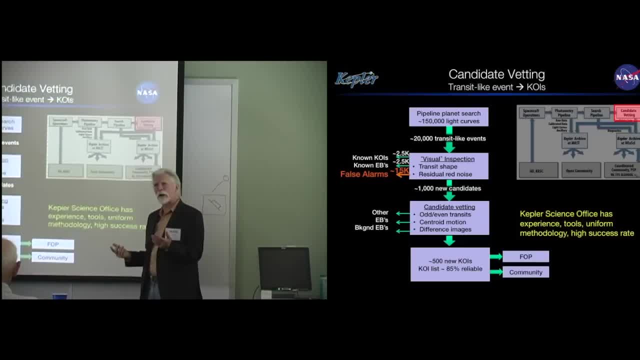 because it's the same planet. If it's an eclipsing binary, they often look different. Simple thing works pretty well. We can take Kepler data itself and look for centroid motions on those blurry images. But we can do it And we can look at difference images. 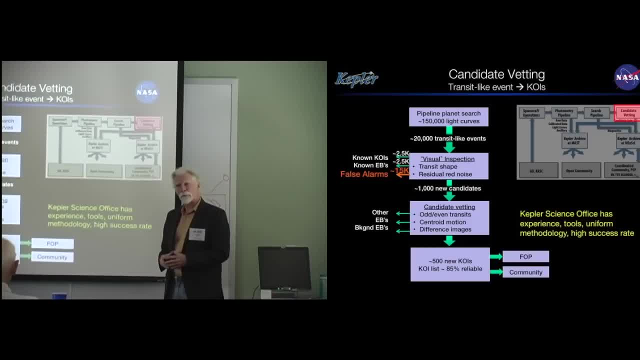 And that works to help you if it's a background eclipsing binary. So if I have a bright, blobby star and nearly co-aligned with it and I can't tell the star is there because it's blended, but much farther in the background is an eclipsing binary. 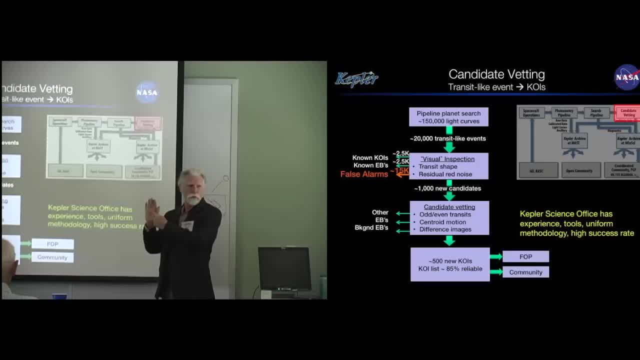 Well, every time that binary eclipses, this bright star looks like it gets fainter, like it has a transit, But it's really the summation of this faraway binary in this one star. But what it does is it changes the center of light during the transit. 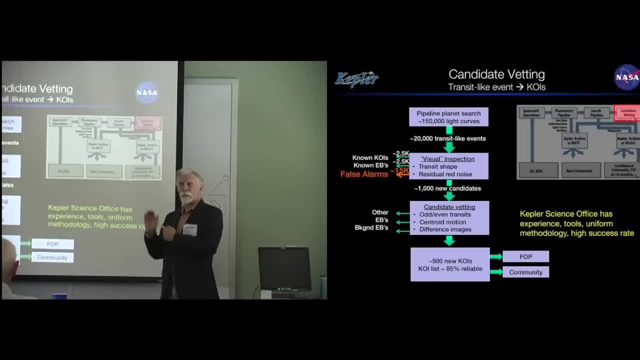 compared to not during the transit, In this case during the eclipse, Because when that thing eclipses, this all of a sudden becomes slightly brighter in a centroid sense, And you can tell, You can see this thing move by again a hundredth of a pixel or so. 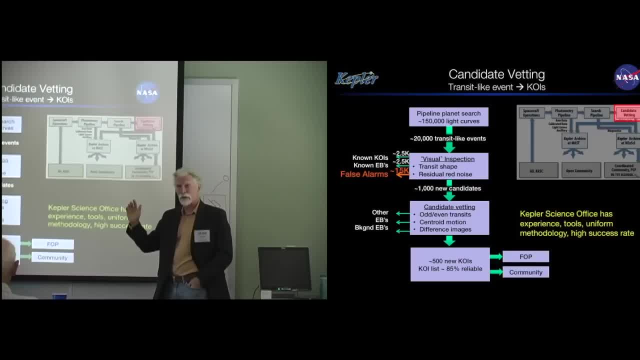 And if you see this shift during the transits in the right direction, then you know it's not really that star that's at the transit point. So there's a lot of neat things that we've learned how to do, but Kepler made it itself as blurry as it is. 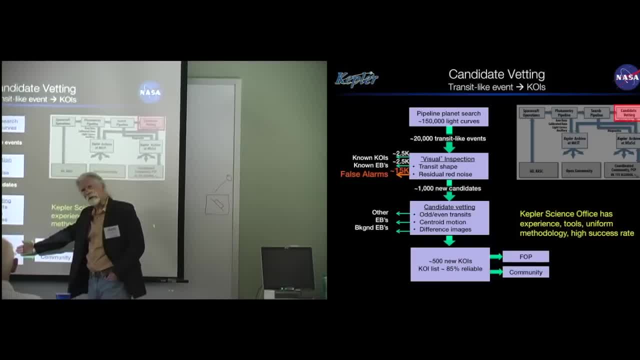 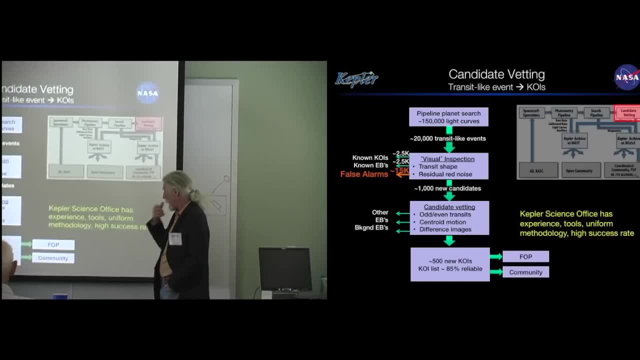 So out of this initial star of 20,000, you might find 500 other planets. These KOIs are called Kepler Objects of Interest, but they're more or less the planets that we get out Now. this is a list that's maybe only 85% reliable at this point in time. 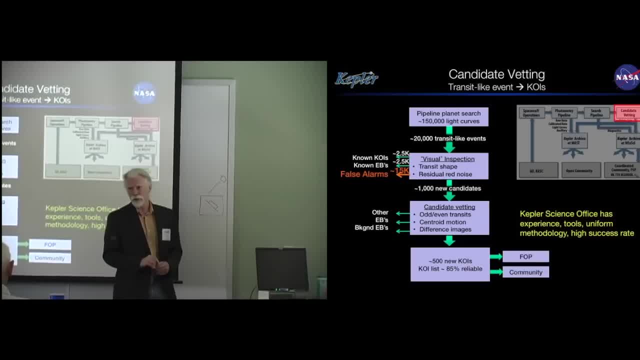 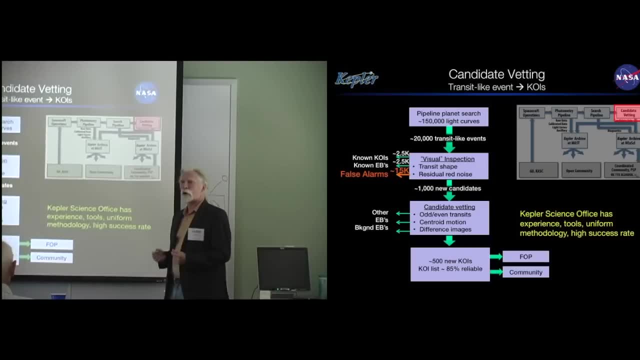 And that's because there's still- there still can be- a set of false positives, For example hierarchical triples, which are really ugly that it's hard for any of this decision tree to get rid of. So these are passed on to the community. 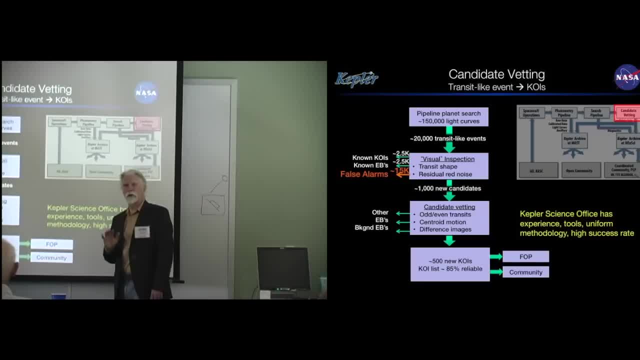 They're passed on to what's called our follow-up program, where we use our ground-based telescopes to go out and try to observe every one of these stars and every one of these candidates and see if we can provide additional information to prove that that's really a planet. 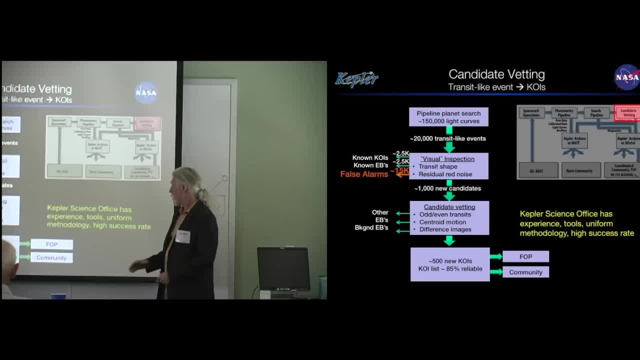 or they're a planet or it's some other kind of false positive. Once we've done this, we believe we're maybe 95% complete, but it's never going to be 100.. So at the end of Kepler's life, whenever that is, 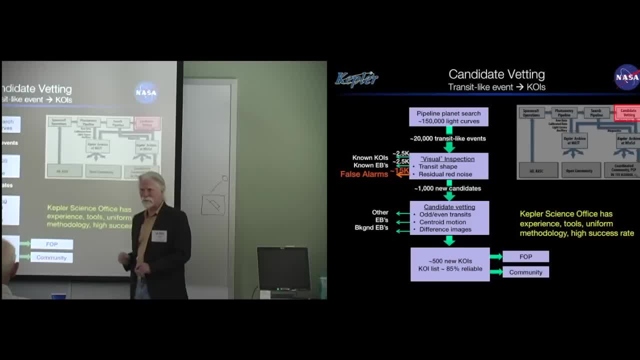 we will never ever have 100% reliability that everything we find is a planet. But if we find 100 planets like the Earth, who cares if 5% are wrong? right, That means that there's 95 that are real. 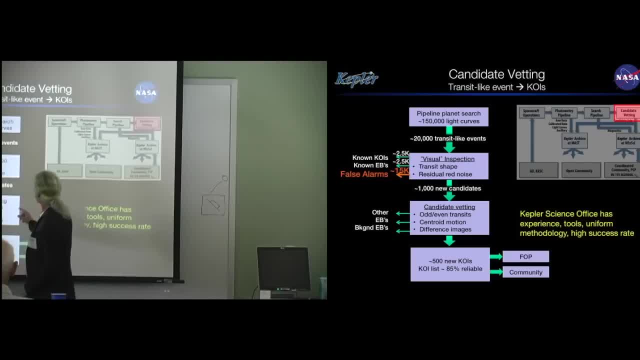 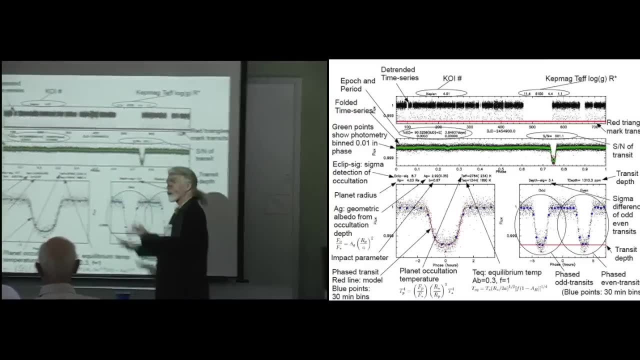 You may know at least one, but that's okay. Now, part of this- this part here is visual inspection, and down into this part here, Let me show you one of the kinds of tools we use. So this looks like a mess. 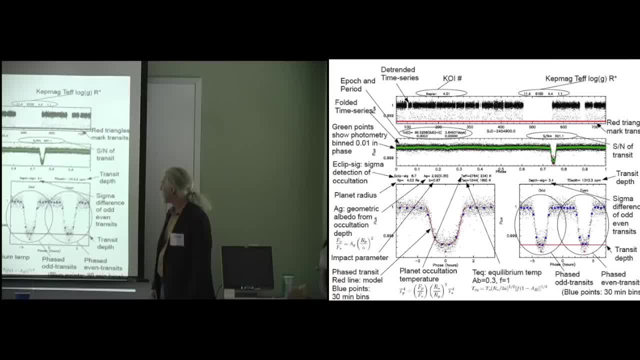 But this is one of our computer-generated products we get And what it shows us. these tell you what the things are down here. They're not all in every form, This is obviously to tell you, But here we show the flattened light curve. 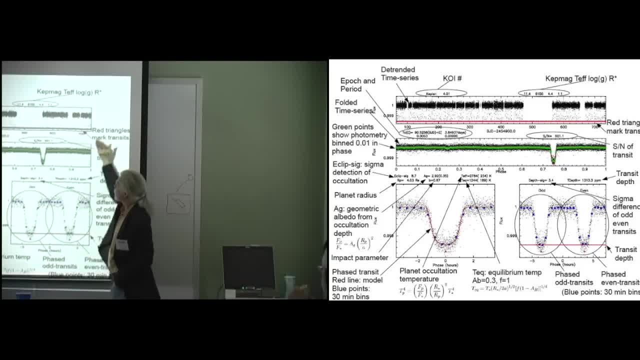 red places where we think a planet transit is. So that's the original light curve. Then we phase-fold the light curve, So here would be the transit. we put it at 0.75, so that we can look and see if there's something over here at 0.25. 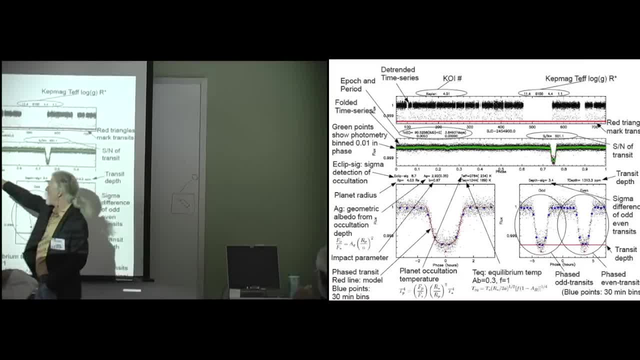 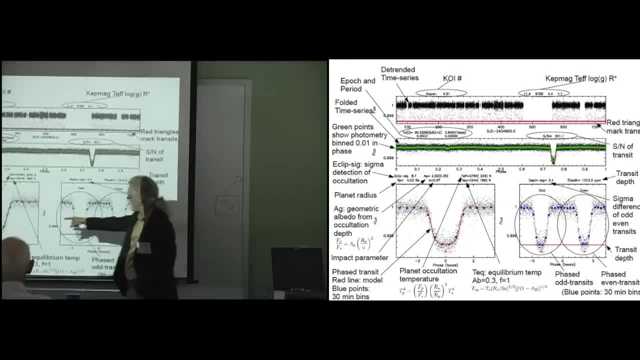 Because if this is a planet transit, there should be no so-called secondary eclipse. You can probably see it right here: It's a little secondary eclipse there. Then we look at a planet model fit. This is the model fit. The red line and the blue dots are the average points. 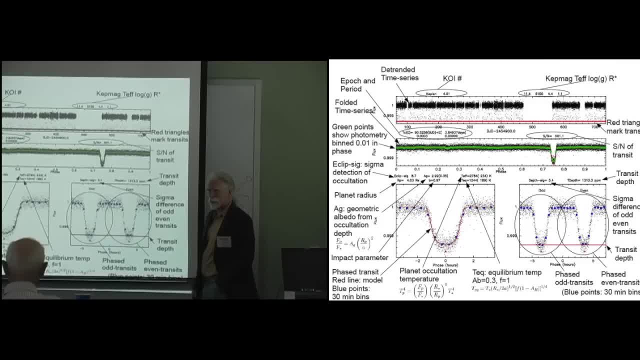 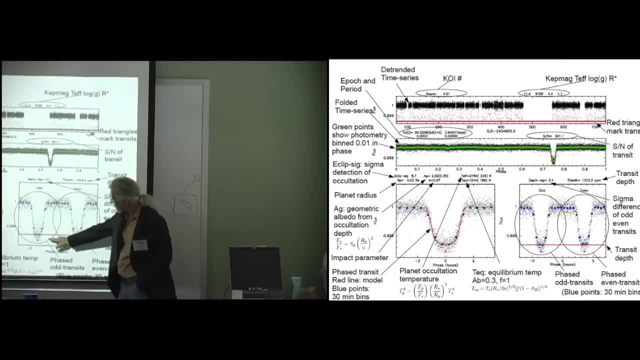 Then we look at the odd-even transits And we model fit both of those. We take that model and lay it on the odd transits and lay it on the even transits And you can see it doesn't quite fit very well. 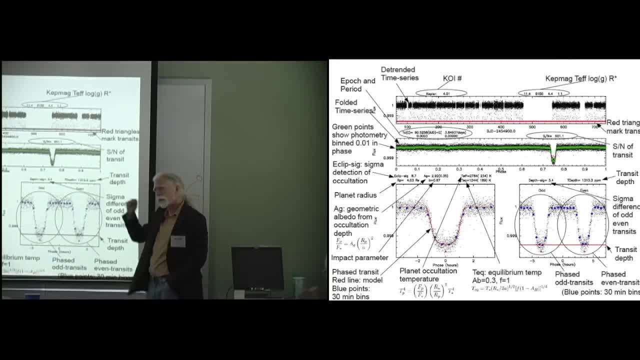 It has this little bottom that's too deep. So this would be a real quick way, once you get good at these, to see this here and see this not quite fitting and you toss it aside and say it's probably an eclipsing binary. 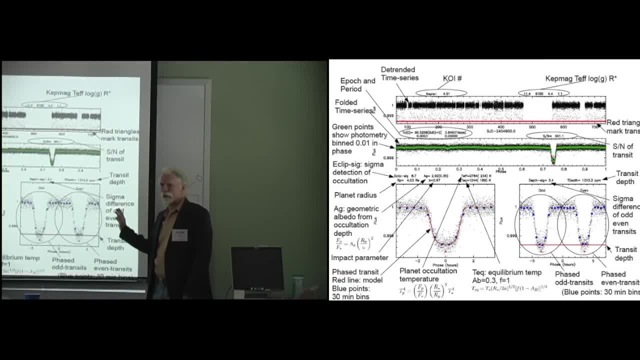 And you put it in the eclipsing binary kit And most of them that aren't bad pixels, most of them are pretty easy like this: You can see them and you just toss them on. And so the group that does this in the so-called science office. 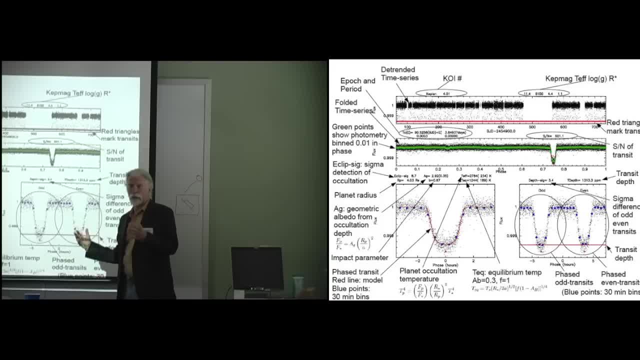 it's about six people that do a lot of this work. Not all day, every day. They spend time doing this once or twice a month. They get down to viewing one of these about every two minutes. That's sort of their rate of viewing these. 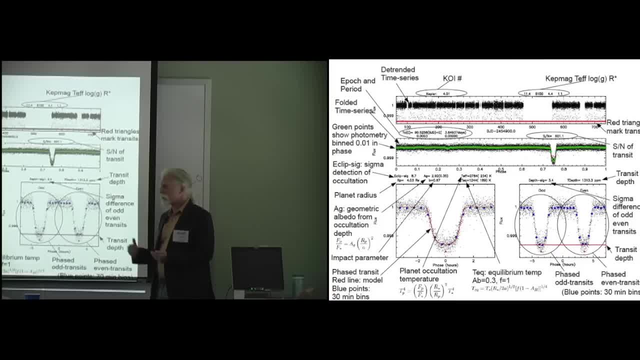 But as more tools and more knowledge is cast, more computer stuff is done to find this. Because we now are searching this light curve to find that And if you find that, you can throw it out and waste somebody's time looking at it. 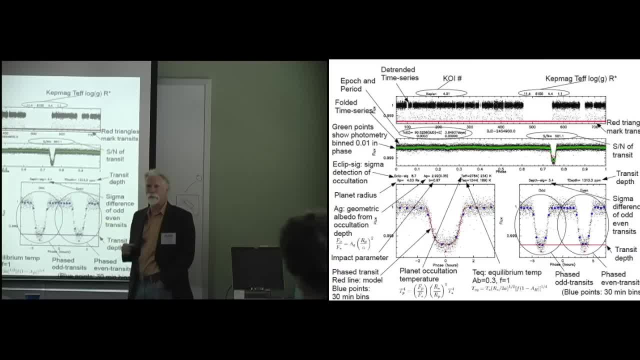 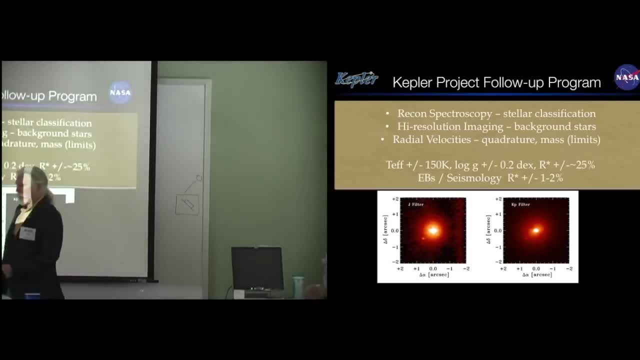 And searching these two phase light curves and throwing them out. they don't look good. So you start learning about your data and you can do a lot more to put things out automatically When we move to the ground-based work. so, as I mentioned, we have this 85% reliable list. 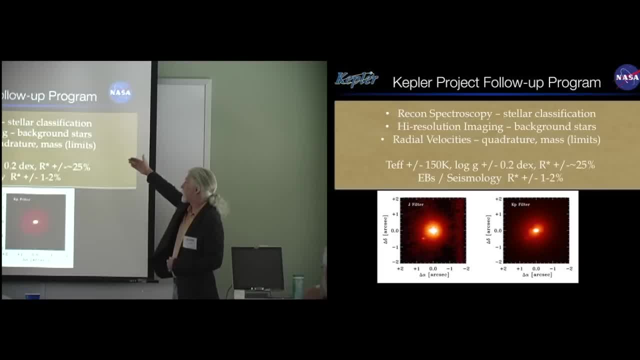 of moving to ground-based work. We do three things, basically This top thing, we do reconnaissance spectroscopy. So this is pretty low resolution spectroscopy, pretty low signal noise. So maybe one or two angstroms of resolution, maybe a little better. 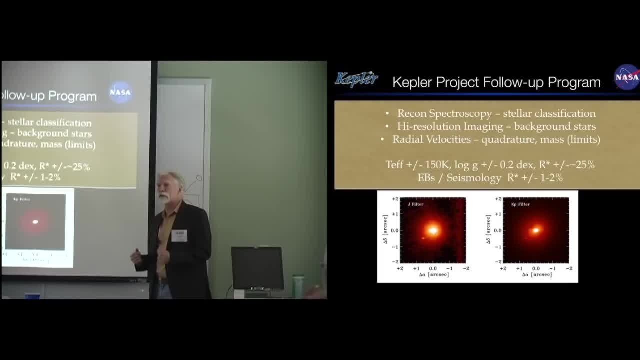 Maybe a signal noise of 20 or 30.. So this isn't anything you're going to do great science on, But it's enough to tell you a few things about that star. Does it have the right temperature, the temperature you think that star has? 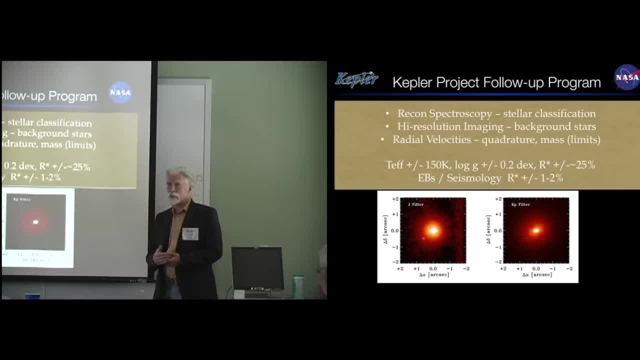 Does it have the right classification? Is it a main sequence star or is it a giant? We'll see in a moment that the way you know the size of a planet, you have to know the size of the star. All we measure is the relative ratio of those sizes. 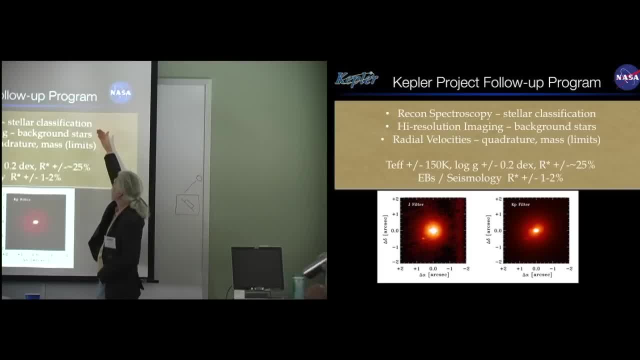 and that's not good. So this is a first step And some things are thrown out here because they look like an eclipsing binary. You see two sets of spectral lines. Some things are thrown out because we thought the star was a G star and the spectrum shows. 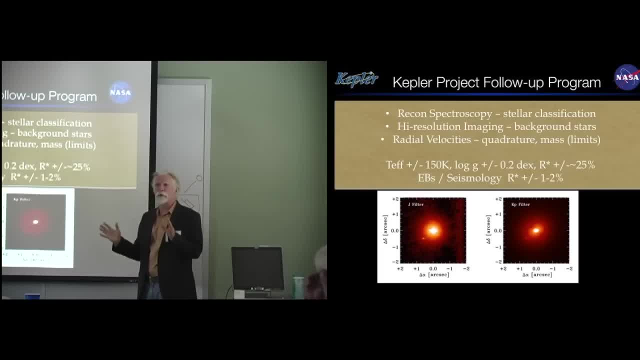 that it's an F star or a K star just because there was a problem with photometric calibration. So this maybe throws out 5% or 2%, not a lot, but something We also do. high-resolution imaging: We take adaptive optics image and speckled imaging. 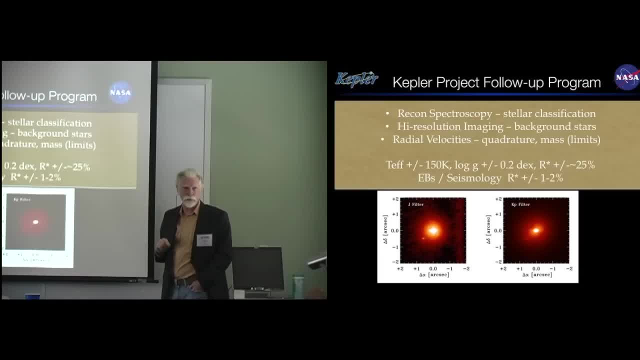 and look for very close companions- not physically close, but co-aligned companions- to see if there's a possibility of some star, that's say sitting 0.1 arc seconds away from this star that is either in front of it or far behind, that could be causing this transit signal. 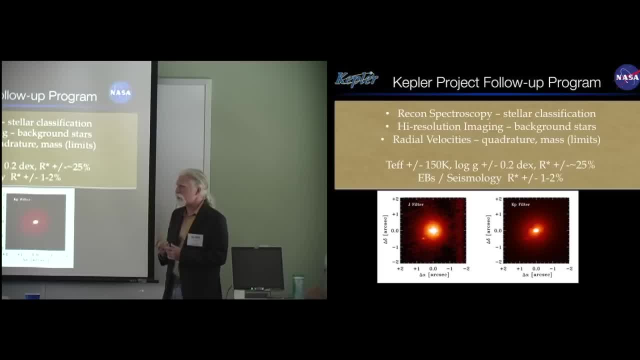 And then if it is, if we find that star, we can't prove just because we see it there that it's causing the transit signal. but we then work harder with the Kepler data to see if we can tell if that star is causing motion or not. 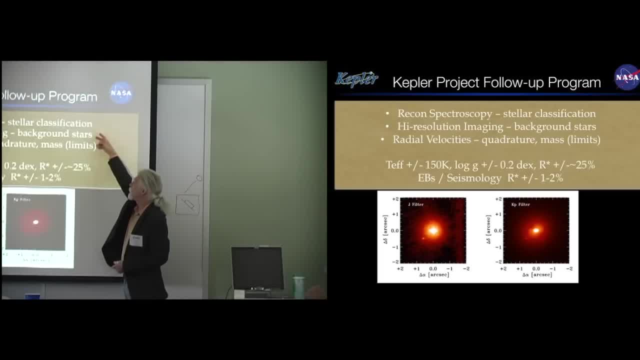 or if it passes these two tests. we then go to this level here, which is usually done with the HEC telescope in Texas or the Keck telescope- some big light bucket that has a very high-resolution spectrograph and we measure it at quadrature. 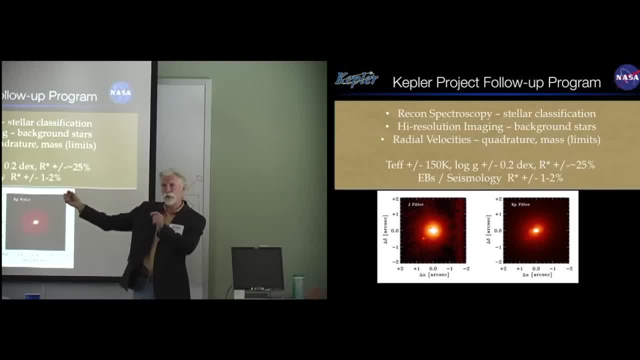 So that's the point where the planet is either out here, moving toward you the fastest, or over here, moving away from you the fastest. If it was a binary star instead of a star on a planet, that would be your best chance of separating the two lines. 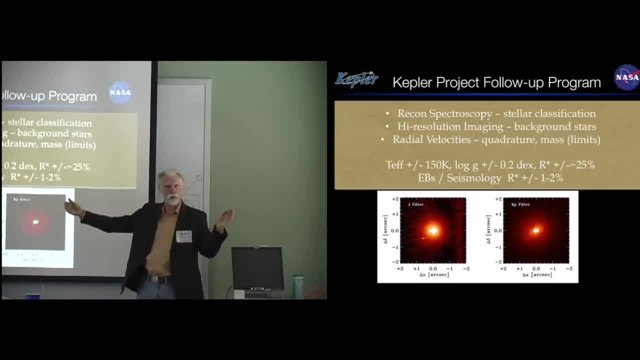 the speckled lines from these two stars. So you look at those two points and see if you can find a second signature of a star. You also try to get masses or mass limits in most of our small planets By looking for radial velocity of motion. 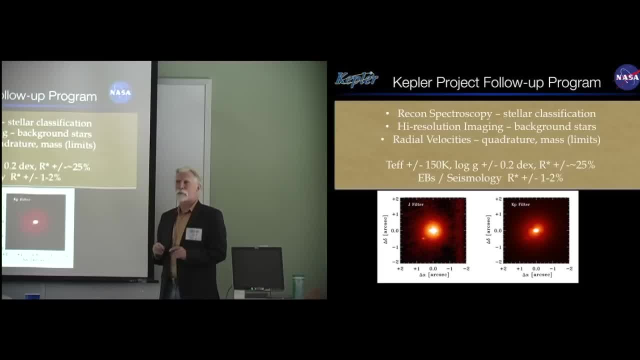 looking for Doppler shifts. If you don't see a Doppler shift, you get more excited because it probably means it's a small planet and not a massive star that's causing the collision. So these are the typical values we get from those three kinds of follow-up. 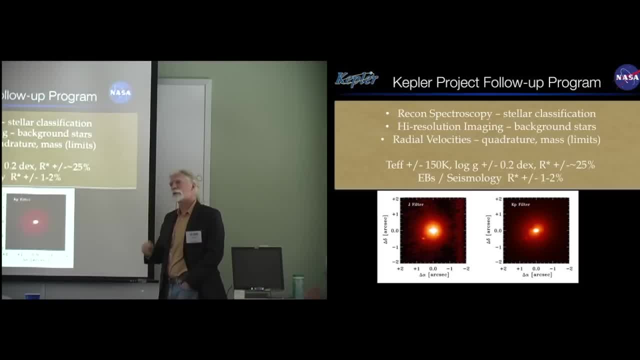 And again, they're not super great but they're enough to raise that reliability level up pretty high, 95% or more. So the temperatures go 150 Kelvin. log G is 0.2 V, and this is the one here. that's still really pretty tough. 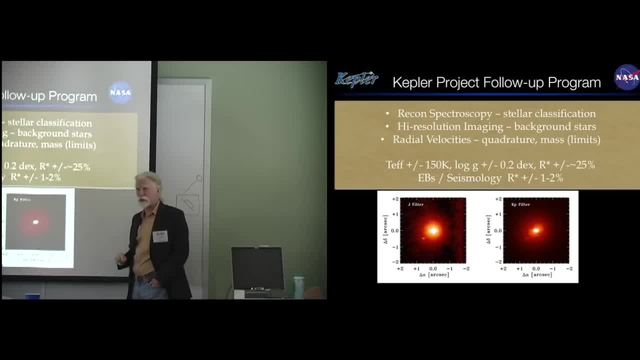 So you only know the radius of your star to about 25%. So again, that means you don't know the radius of your planet all that. well Now, if we can get seismology or if we find planets around eclipsing binaries. 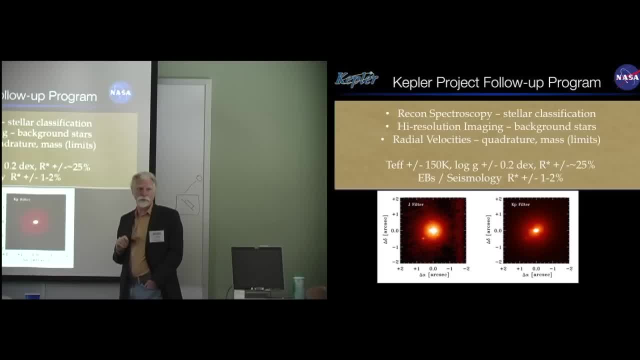 then we can get the radius of the star to about 1% or 2%. So this is sort of the holy grail. but so far there's not many planets in eclipsing binaries. We have nine, but not anything like the thousands of them. 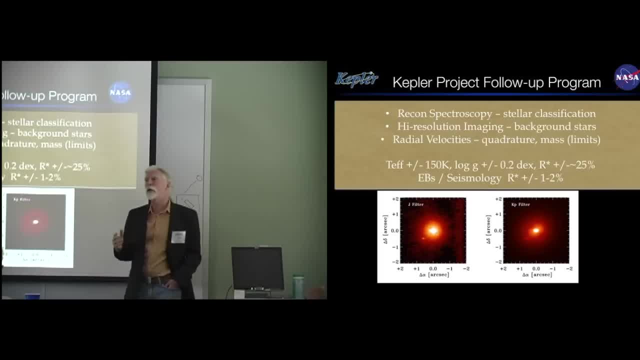 And seismology works really well, but it can only work on the very brightest stars, maybe the brightest 100 or the brightest 200.. Yes, So the reason you don't know the size of the star from the duration of the transit is because you don't know the inclination of the star. 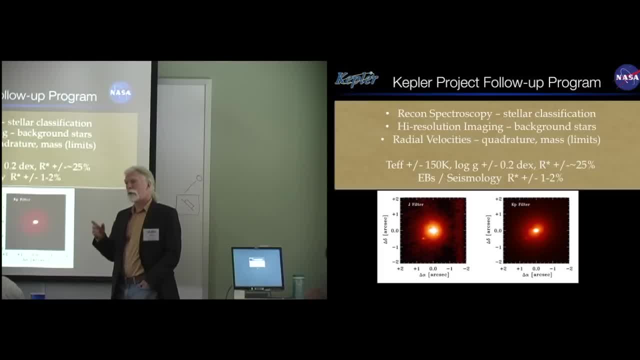 That's right. We don't know the inclination and we don't know if it's a circular orbit. So we make our model fit, based on a circular orbit, and we can have some information on the inclination. And then that depth is the ratio of the size of the planet. 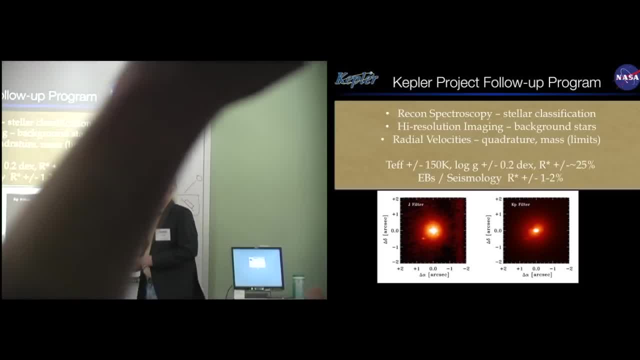 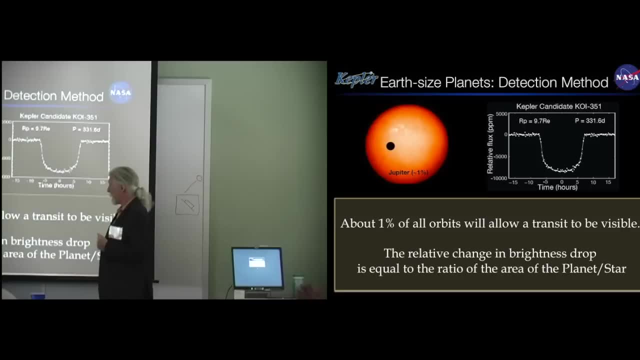 to the size of the star. So there's a couple of factors in there. we just don't know very well. Okay, so, as I mentioned, this is how you do transit. It's very easy. So if you could see a Jupiter transit, 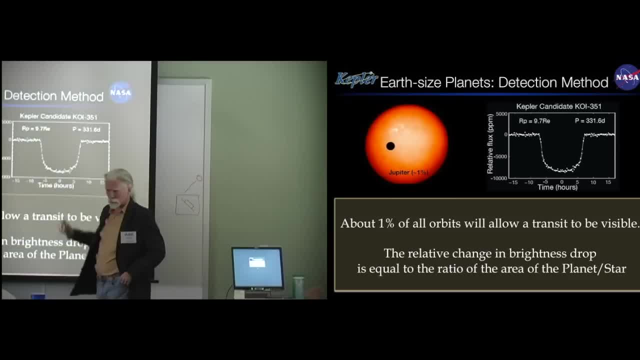 you can't from the Earth. If you could, Jupiter would look crossing our Sun. So wow, that's pretty big. You can resolve that very nice. And this is the light curve it would make. It would have this cool rolling pattern to it. 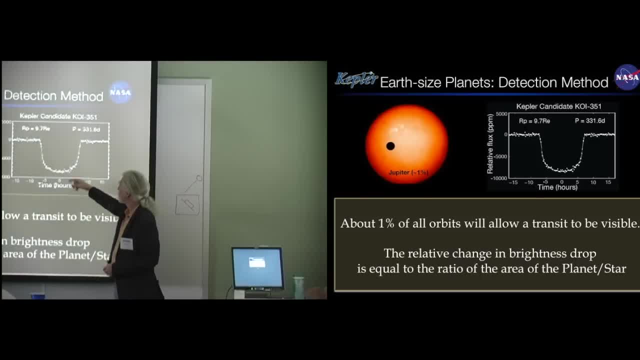 So this is the light curve we make. So this is a real Kepler light curve. It's a planet that's 9.7 times the size of the Earth, so that's about Jupiter's size. There's absolutely no doubt. this is real. 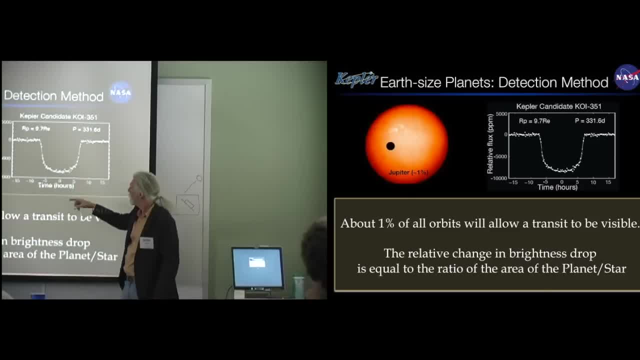 This has a signal noise of 820 or something like that And you can see the characteristic U shape here. It's not a square, It's not an inverted top hat And that U shape is because of limb darkening. It started looking darker on the edge of the sun. 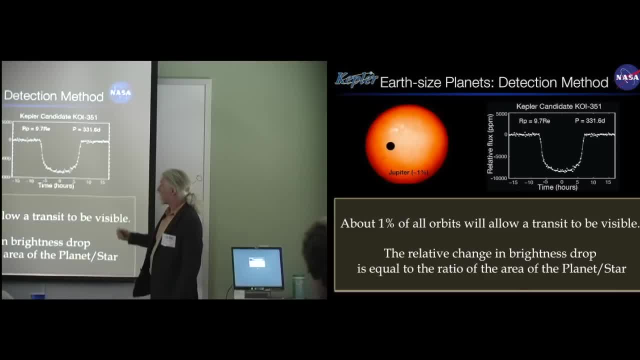 So you get this characteristic U shape. So 1% of all the stars. if every star had a planet, we would still only see transits for about 1% of them, because we have to have the orbits perfectly aligned with the point of view that Kepler's looking. 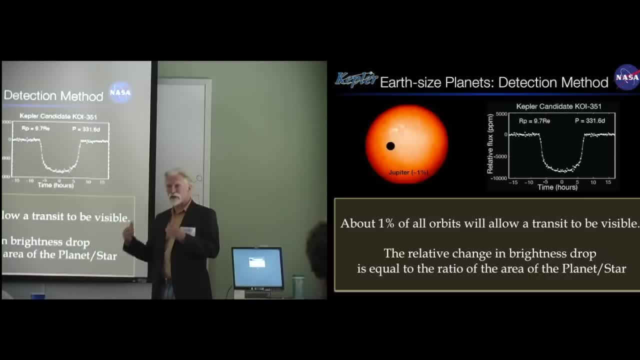 So anything Kepler finds you have to take into account. you're only seeing the edge-on system, so there's many more you're not seeing. And it's the relative brightness, It's literally that drop in brightness that just gives you the ratio of the size of the planet. 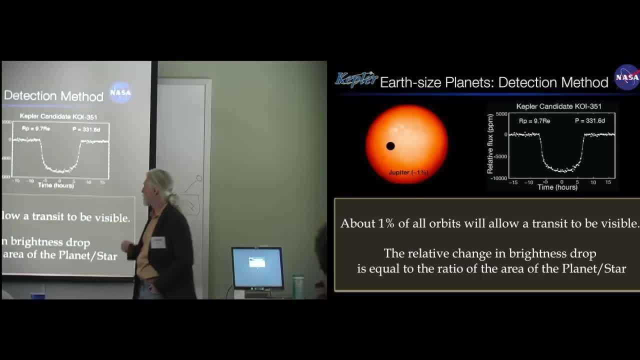 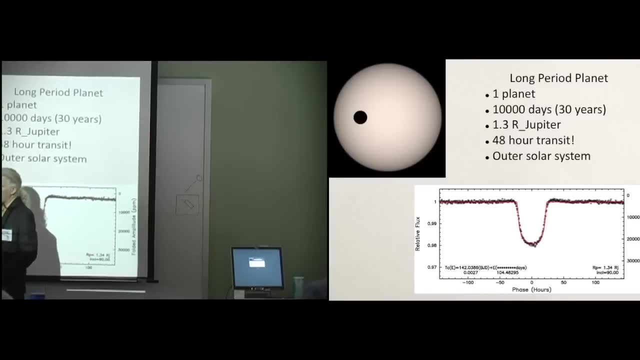 to the size of the star. It's such a simple experiment. It's amazing how simple it is, but it works. So let me show you a few examples of these. So over here is not a Kepler picture. This is a drawing of what the planet 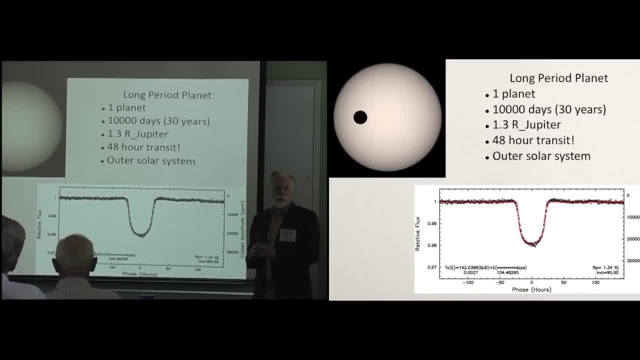 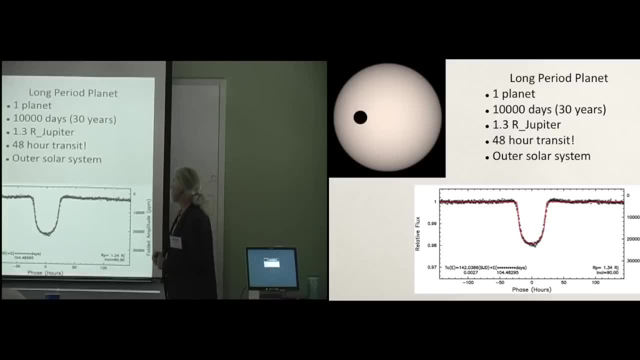 and the star's size would be if you could actually see the transits of this planet. You can't recall the Kepler. This is a pretty good-sized planet orbiting a fairly, in this case, a late K star. So we've only found one planet in this system. 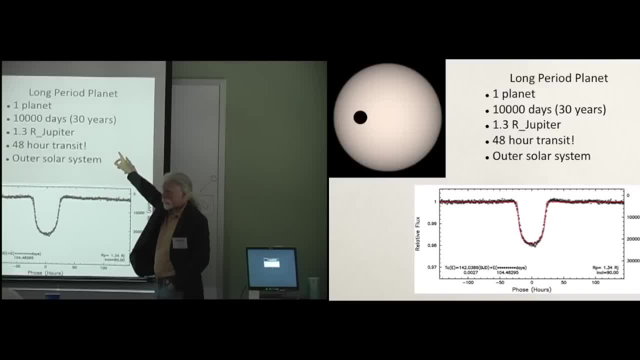 We think it has a 30-year orbit, 1.3 times the size of Jupiter. Its transit is 48 hours long, so it has a long period. Now the way we estimate this- 30 years- is we take that time. 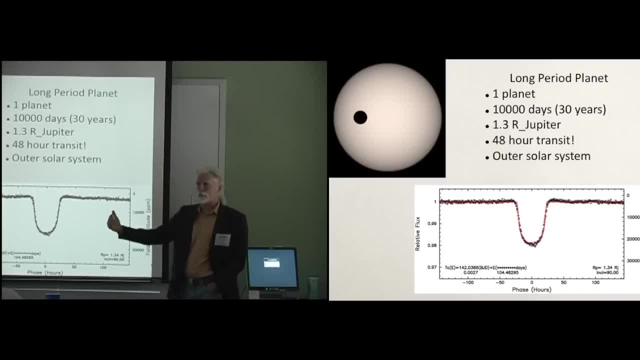 assume it's a circular orbit and then say what would its orbital period be? We will never see this transit again, so we will never know about this. I can't imagine even Kepler would work in 30 years from now, But this is at least some evidence. 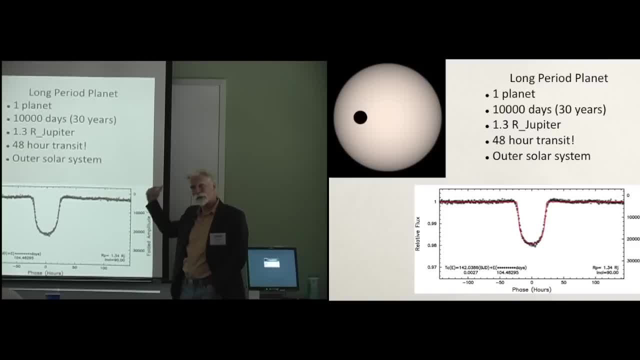 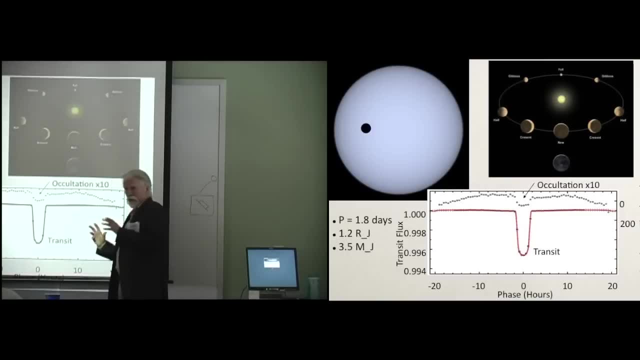 that planets like our, Jupiter, exist in at least 100 solar systems, So they belong up here. The hot Jupers, the so-called close-in big planets, are becoming a real interesting goldmine for people that like doing planet weather and planet atmosphere. 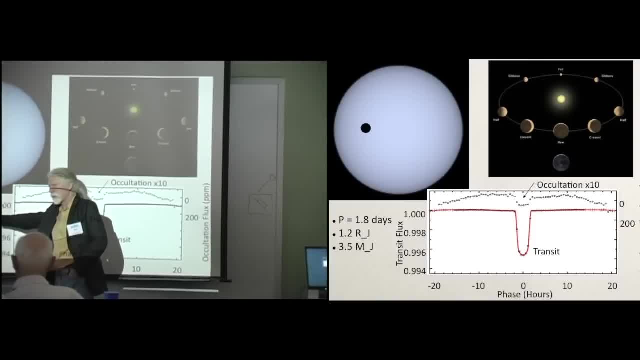 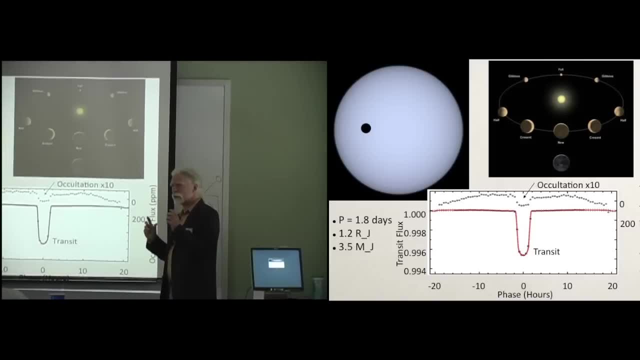 So here's a planet that has a period of 1.8 days, It's 1.2 times the radius of Jupiter and it's 3.5 times the mass of Jupiter. This is the so-called hot Jupers. 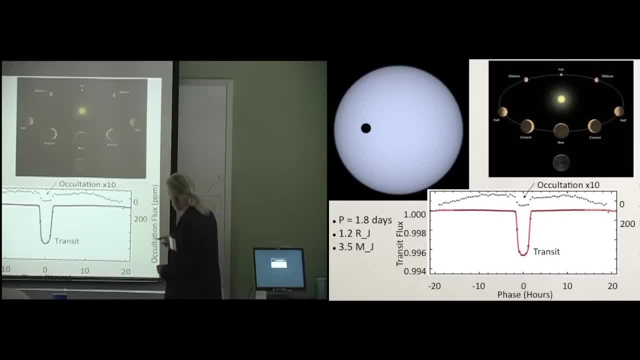 These things are just screaming along the surface of the star they're orbiting. Here's the transit down here. The red is the model fit to the data. They are indistinguishable in this case. We have so many transits: Every 1.8 days we see a transit. 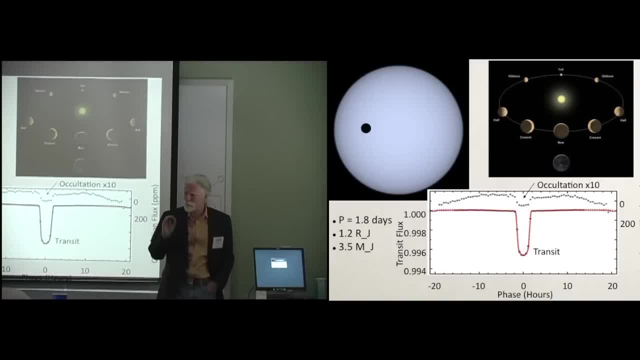 So there are literally hundreds and hundreds of transits that you can go down here. It's just spectacular. But the neat thing is, if you look at the light curve on the other side, when the planet goes behind the star, you see this thing that's called a phase curve. 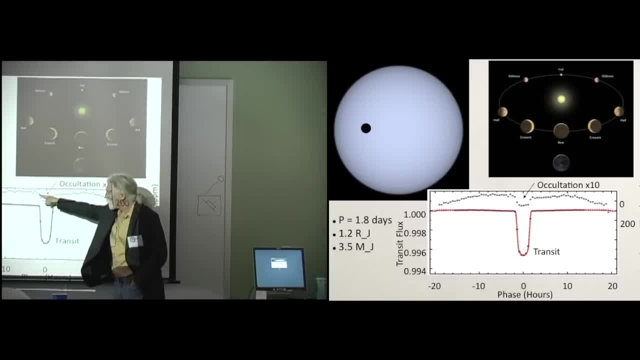 and you can see the depth here of light. You actually can see the drop in the reflected light from the planet's surface as it passes behind the star And this kind of works. my little ad up here. it kind of works like Venus. 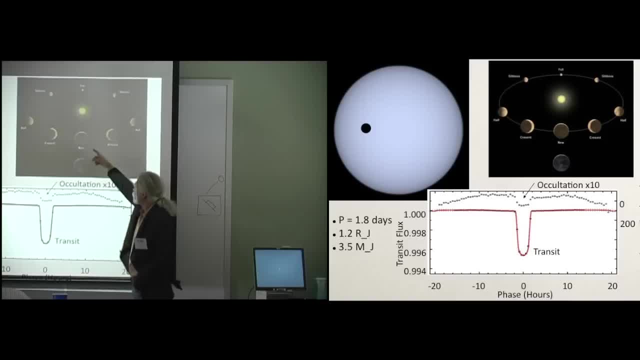 You have these phases of Venus where it goes around in the sun, These transits, and that would be the occupation of Venus. They have a full moon there when they have a full Venus or a full planet. So this shape and this shape can validate these planets all by themselves. 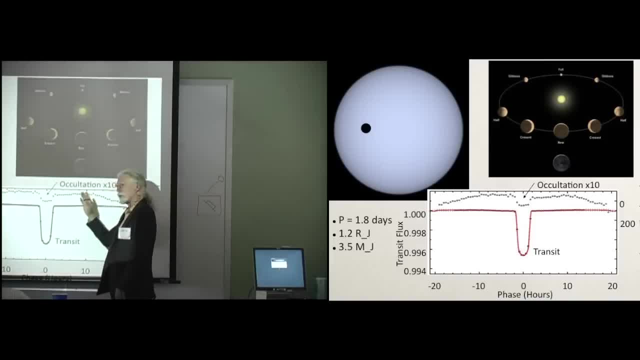 because you can fit models to both of these. You can tell if it's a circular orbit or not and you can eliminate the possibility that it's a binary star or some other triple or some other background eclipsing binary. But even more interesting, 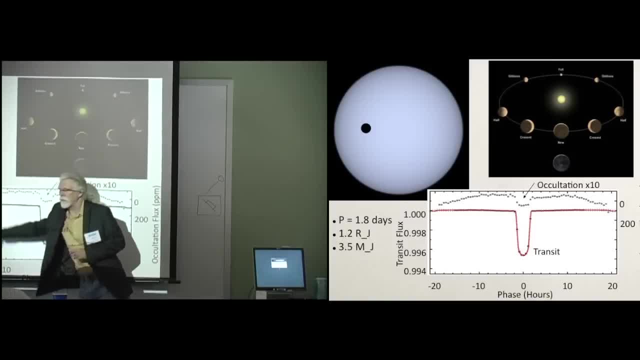 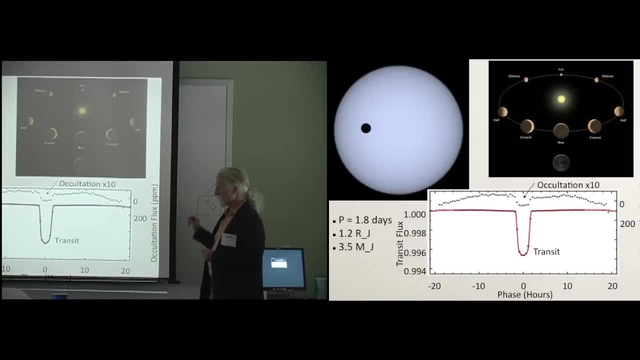 this curve going up and this curve going down tell you about how light reflects off that planet's atmosphere. And so far, in the five or six cases we can do this for- and there'll be many more as we collect many more transits- 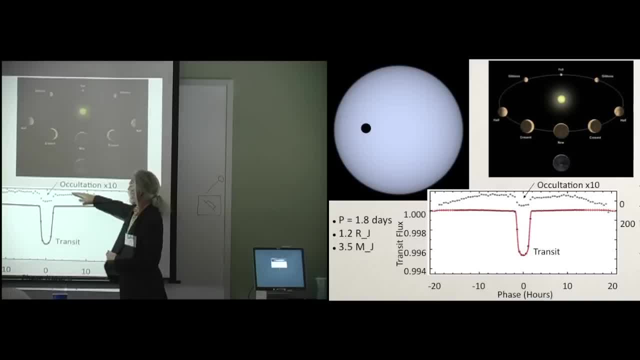 none of them have a symmetric up versus a symmetric down, So they should if the planet's just sitting there. But what this tells you is there's heat circulation on the surface of this planet. It has a rotation. There's atmospheric motion that's carrying some sort of heat. 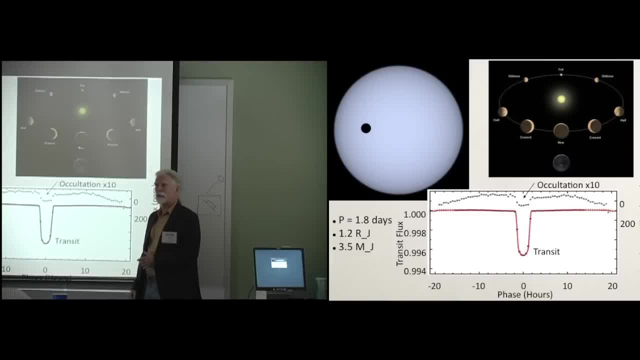 in one direction, making the planet slightly brighter in that direction. So we'll be able to do planet weather from these and as time goes on maybe you'll see a change. So it's a really interesting new branch of work that's coming out of Kepler. 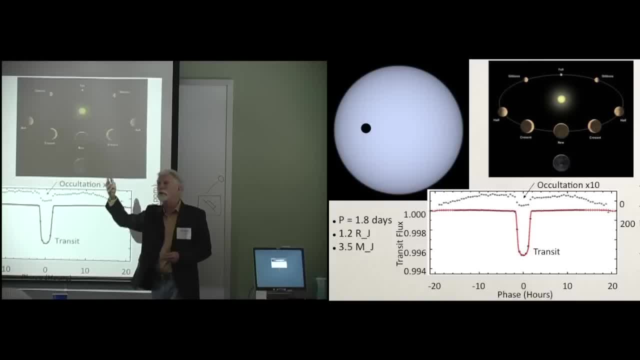 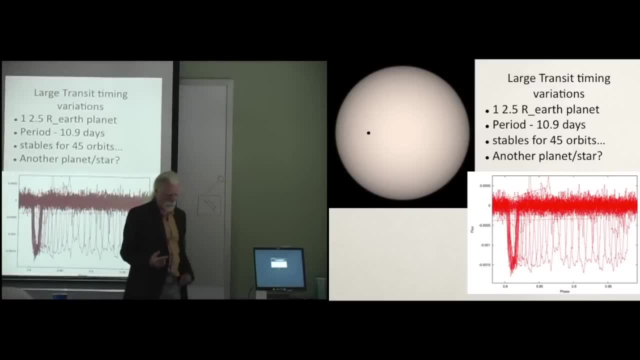 And there's just so much to do here and we have a bunch of people back here, so we'll be doing this afternoon. You know this is a lot to do, so that's pretty neat. Another neat thing that's come from Kepler. 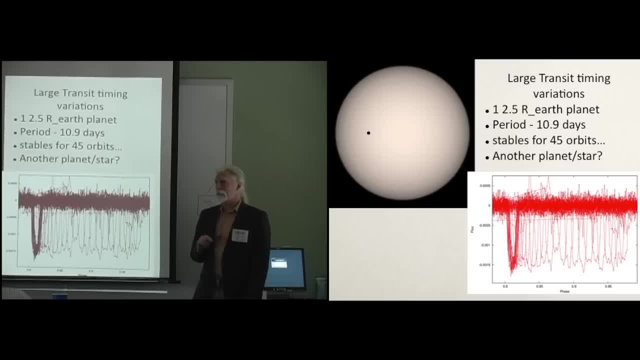 is the discovery of non-transiting planets, And there was just a paper announced about finding one of these. Well, there's many, many of these that are probably going to be found, So here's an example. This is a relatively small planet in this case. 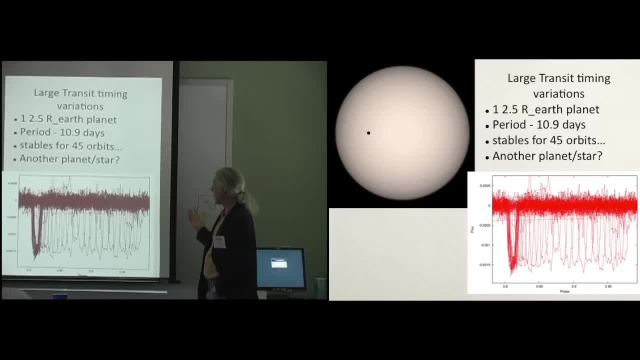 two and a half times the size of the Earth. It has an 11-day period. So the first 45 orbits- this was the phase light curve- and these are the first 45 transits stacked right on top of each other, Starting in orbit 46,. 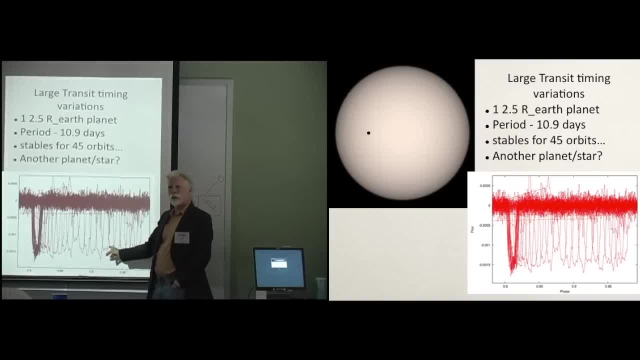 the transit started becoming a longer and longer and a longer and a longer orbital period, by a little bit each time. The transit had changed its time. The orbital period was getting longer by a few minutes each time, And it is almost certainly due to some other planet. 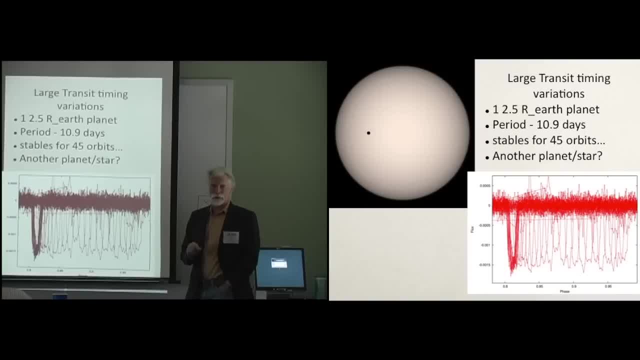 that's in this planetary system which doesn't transit but has a relatively close orbit to this one and is gravitationally interacting with it and causing these two to exchange energy and exchange orbital periods. And if you plot the so-called O minus C diagram for this, 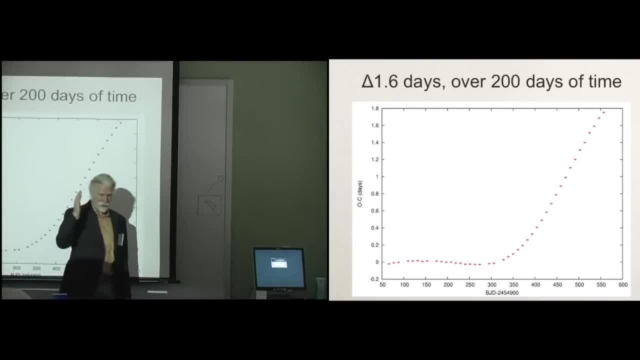 so it's the time that would be. the transit would occur exactly when you predict it to occur if the orbital period is constant. Here's the first 45 days And you can see on this graph that, even though we thought it was pretty constant, 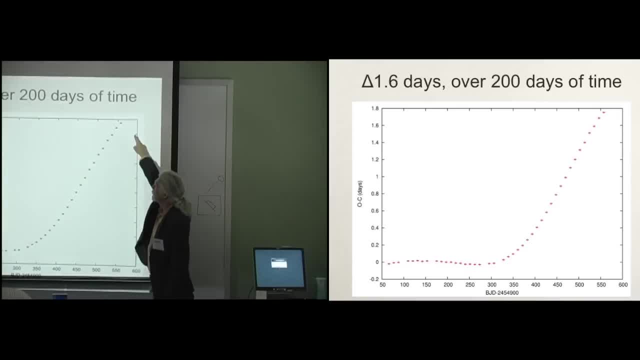 it had this little curvature to it here, But after day 45, it changed and over 200 days the orbital period of this planet changed by 1.6 days. We're now watching this one and this curve has started to roll over. 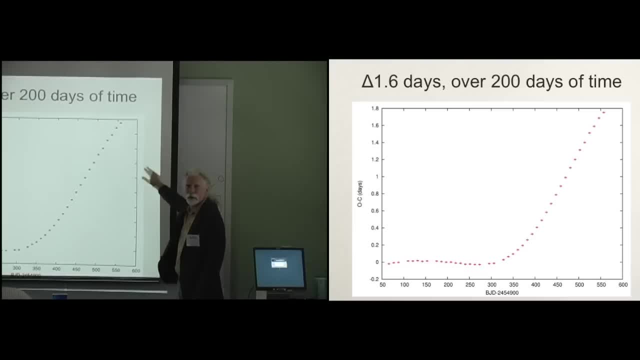 So eventually the orbit of this changing transit here will allow us to estimate the mass of this planet and its perturbation in this particular solar system, And there's a lot of it. We see lots of planets where the transit times change, and then you can use that to estimate masses. 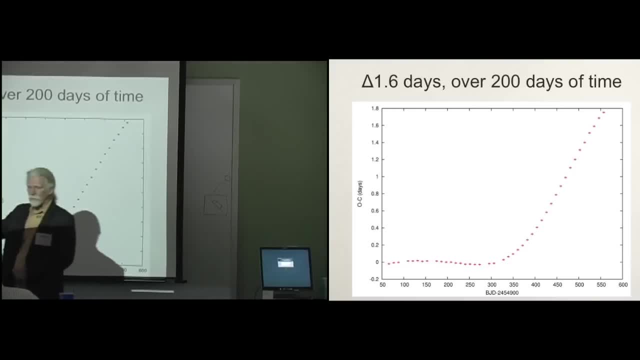 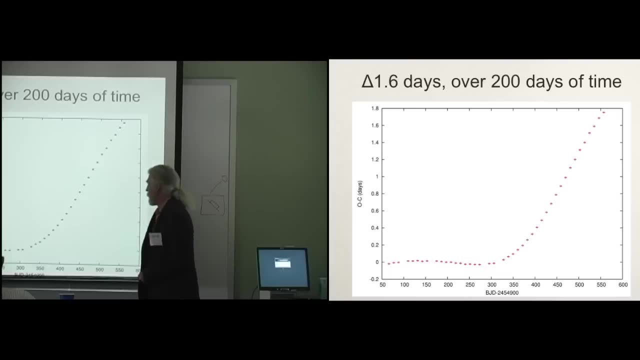 and orbits. Very funny- Correct me if I'm wrong, but the traditional secular interaction through sinusoidal equations. why is this not a sinusoid? Well, probably the reason is because there's more than one other planet In the complex systems that we see. 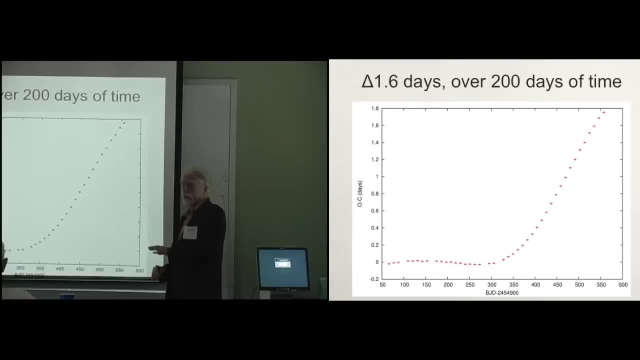 with 3,, 5, and 7 planets, and there's 4s and 6s, but the 3,, 5, and 7s seem to be the ones that occur right now. anyway, the patterns are incredibly complicated. 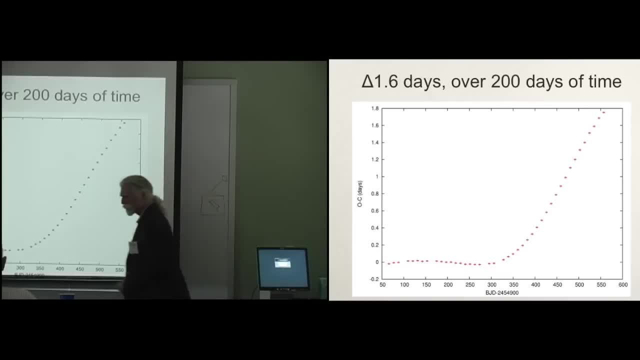 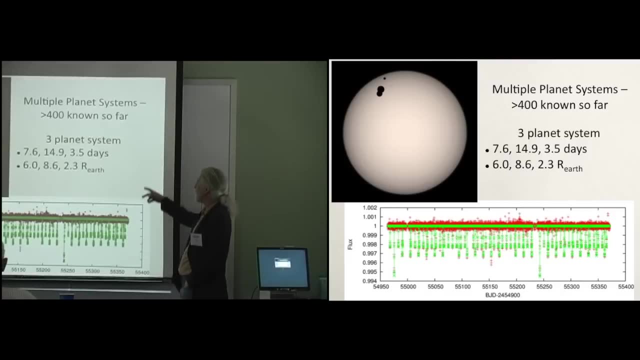 as three planets are exchanging energy, So a lot of neat dynamic science is coming out of this. And then multiple planets. as we've talked about before, we have over 400 solar systems for things with multiple planets. here, This particular one has three. 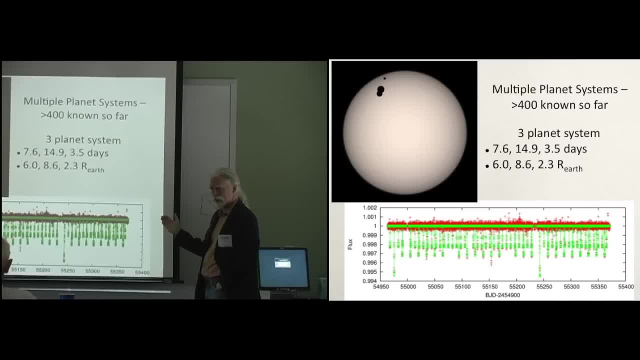 For three planets. our record so far is six, but three of them have six now. So if we're long there'll be seven, eight and that's going to be nine, like our solar system, And again, they're pretty easy to see here. 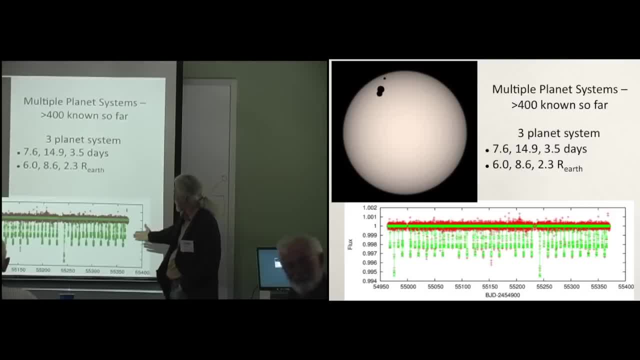 Just start matching them up. It's a little puzzle game. This is the famous Chapter 11, the first really multiple solar system. we've seen kind of a nice light curve here, And this is of course, what you find when you look for a short amount of time. 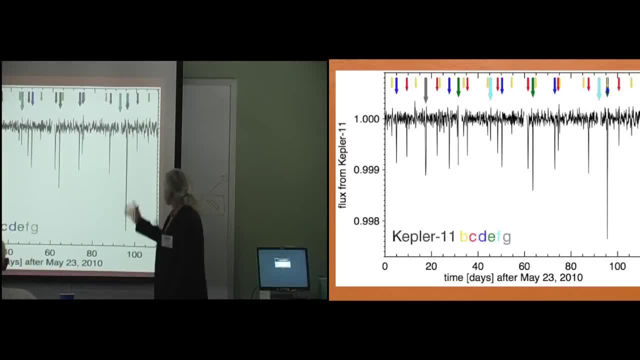 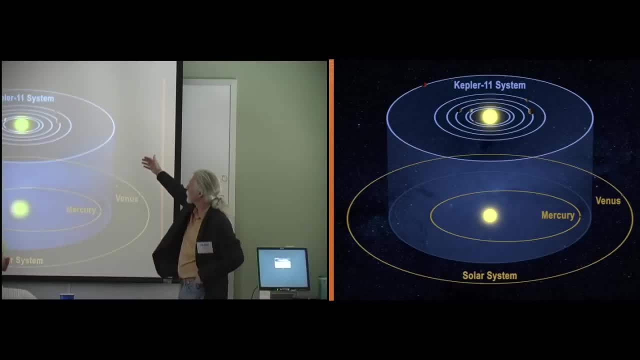 So this is the first time that we've seen a really multiple solar system, And this is, of course, what you find when you look for a short amount of time. So this is the first time that we've seen a Kepler 11 system. 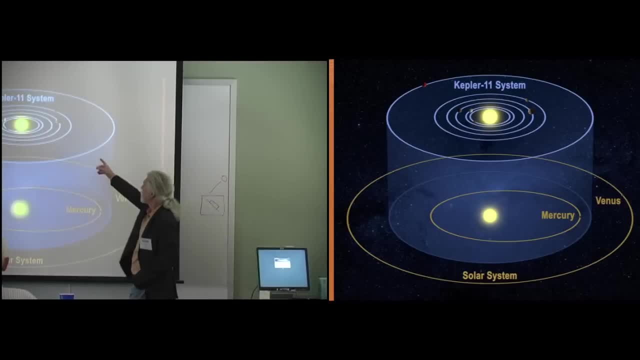 on the same scale as our solar system And you see that all the planets here are basically jammed almost inside the orbit of Mercury, So they're really close in And, of course, when you look for a little bit of time, you find close-in planets. 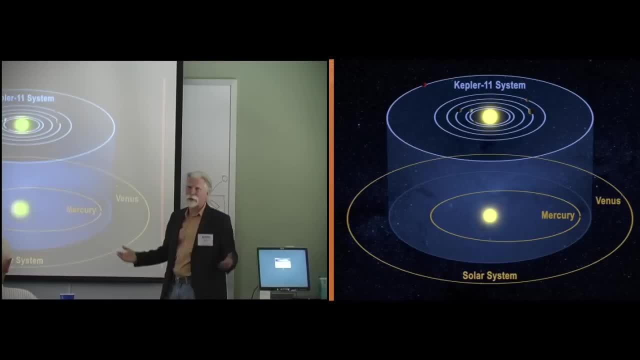 As Kepler continues to look for longer time, you find longer period planets. So it seems like that planets are everywhere. They're in all kinds of orbits And you know we're going to eventually find something that looks just like us. and people are coming out. 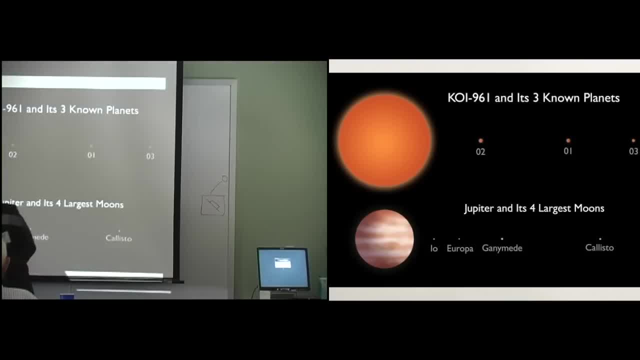 So that's pretty cool. Another one of my favorite solar systems is this one. So the other one, the one that's jammed inside the Mercury's orbit, almost Here's a small M star with its three planets, And on the same scale, 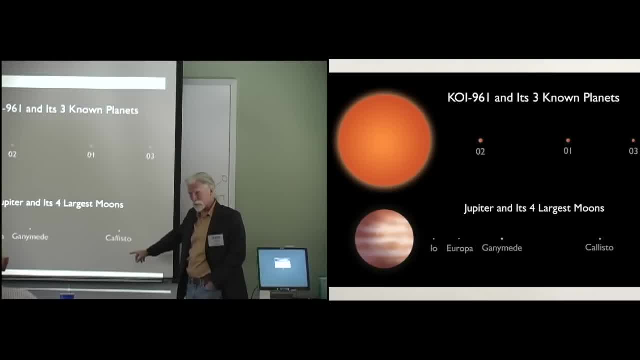 here is our planet, Jupiter, with its four largest moons, And this is just pretty cool. So here's the entire solar system, Here's our planet. You name the size, you name anything and you'll find it Okay. so we talked. 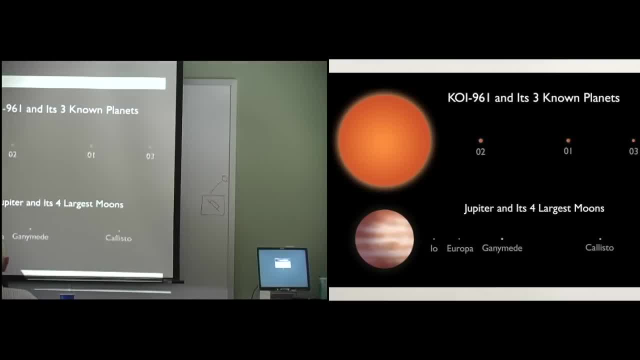 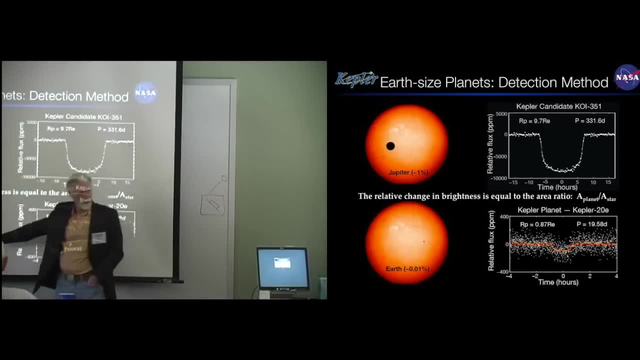 about Jupiter before. So here's the sun, or here's the Earth transiting the sun. I don't know if you can see it. So this is the excitement you'll see if you actually take a look at it. So this is the Earth. 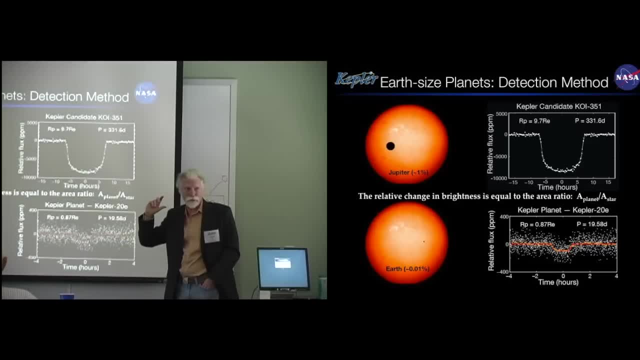 transiting the Sun. So this is the Earth transiting the Sun. You just use your eye to look at the transit of Venus. It's possible, but it's tiny. So this gives about a 1% drop And this gives about a 1-100% drop. 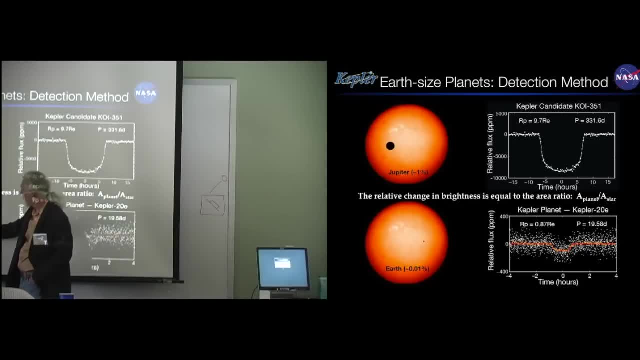 And again, it's just the ratio of the planet's size to the star size, So that transit's really easy to see. This one's not so great. That's the real light curve down here And again, if you average over time. 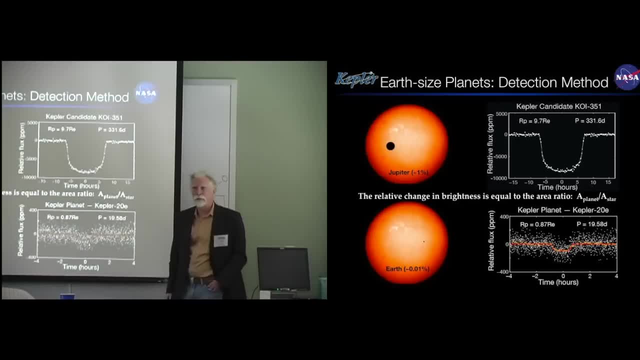 the transit shows up. So you just have to collect many, many of these. Now that sounds easy. Well, when you look at the Earth transiting the Sun, it is easy in this case, because this has a 20-day period. So if Kepler 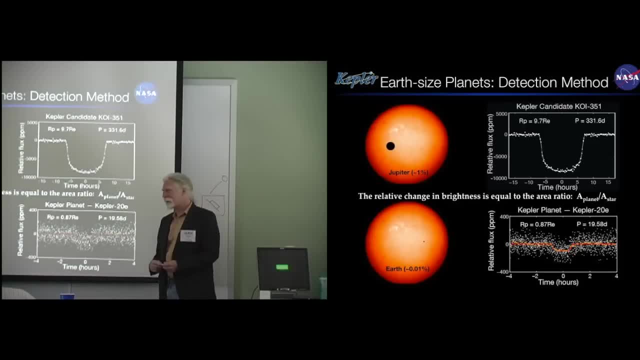 looks for a year. you get a lot of transit so you can come out of lunch. But we're trying to find planets this size that have one-year orbital periods. So if you see one of these, well, you're not going to believe it. 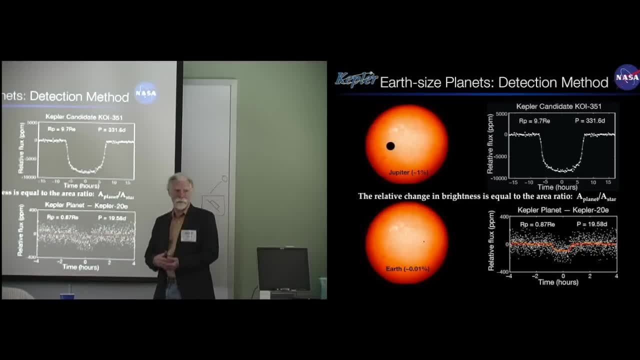 So three or four or five or six or something is what you really want. So you have to look for a period to care about it. After a couple you can see it, You don't? So just to show you that Kepler finds lots of these: 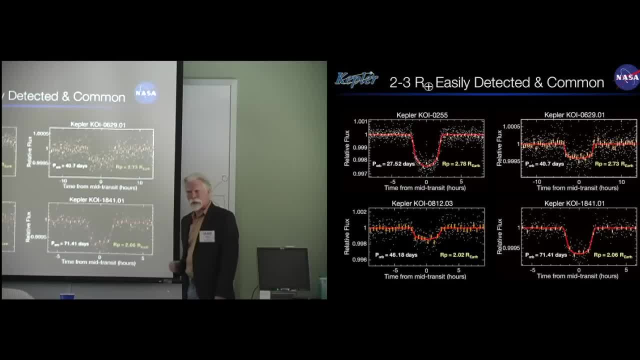 and they're really easy if they're bigger. These are now things between two and three times the size of the Earth, So sort of getting out toward Neptune, And these are trivial to find. now, The software is so good, The detection algorithms are. 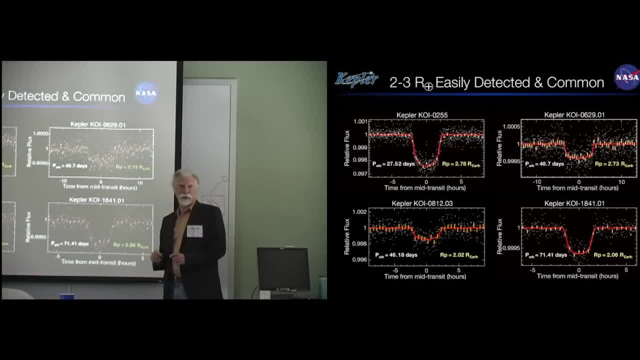 so good, The light curves are so good, So we have no problem finding them. But we're always at the limit, because that's what you do: You push to the limit of your experiment. What can I just barely do? So if these 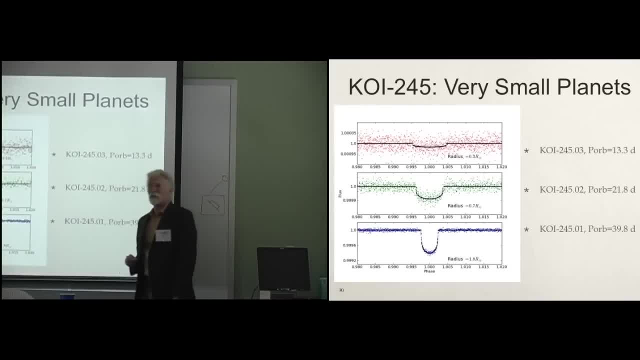 were not easy to find. we'd be in trouble finding one or three. So the latest discovery, which will be announced soon, so you're hearing it here first, is this particular object here, Kepler, Object of Interest 245, which is known. 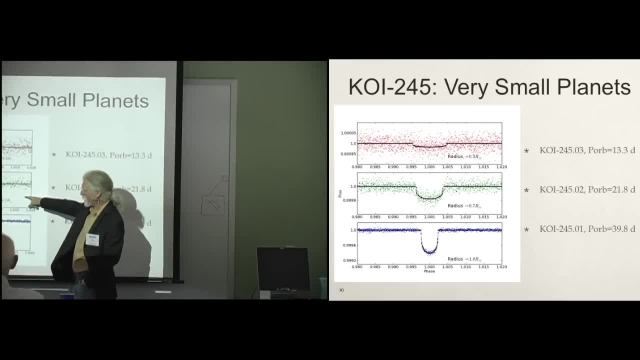 to have at least 0.7 times the radius of the Earth. This is 1.8 times the radius of the Earth. This one up here, if it's real, and the paper will tell you it's real, we all kind of. 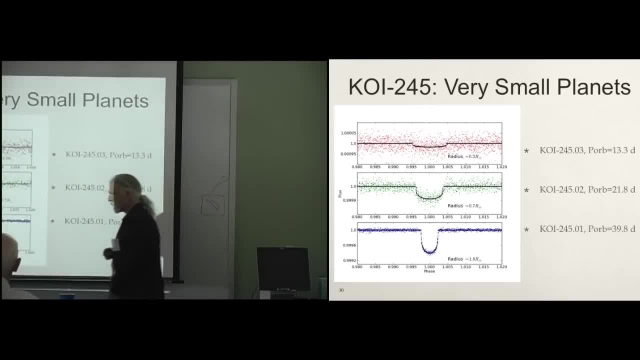 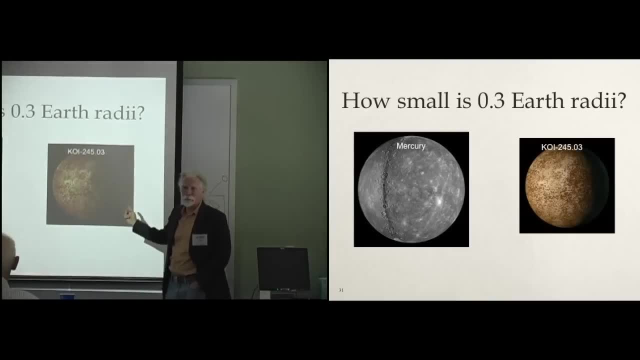 believe it now- is only 0.3 times the radius of the Earth. So this is a little smaller than Mercury actually, So it's the size of that planet. So it's pretty cool. Kepler is finding tiny things. Again, you win. 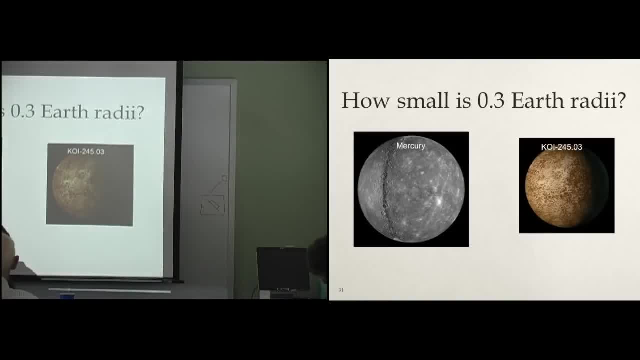 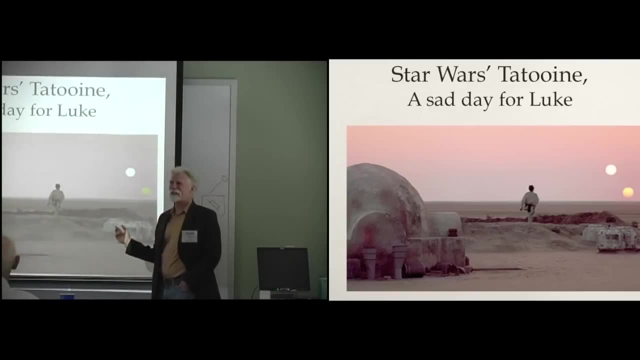 because these things have a lot of transits, So we won't be finding 0.3 in Earth moments. So how many of you have seen this movie? A few, right. Well, here's the Kepler picture of the same. 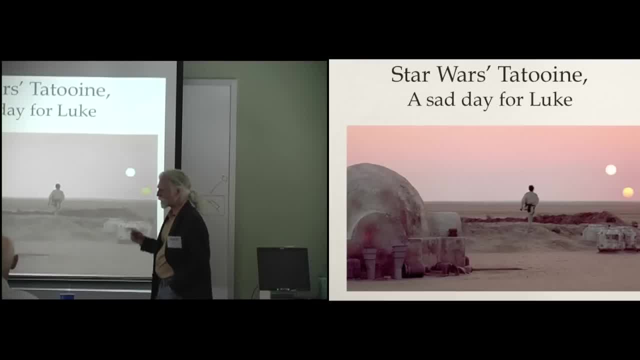 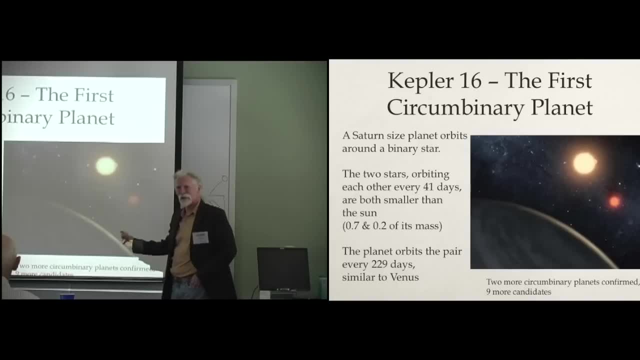 thing. So this was Kepler's discovery of a planet orbiting and closing binaries. So this is the Kepler discovery of a planet orbiting and closing binaries, And this is the first one that was found, And we now have nine more and maybe even. 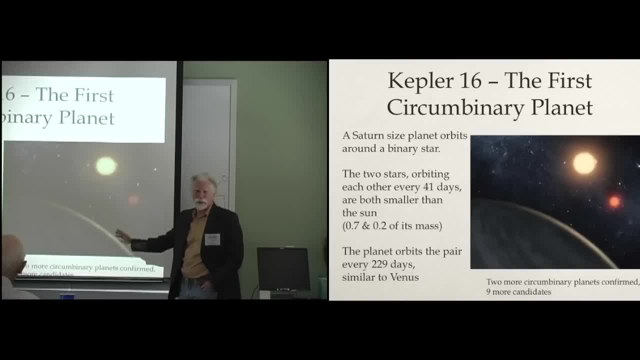 25, that are even canadians. So it's certainly not as common, it seems, as single stars. And this is a Saturn-type object, It turns out this particular planet is close to the magical habitable zone, But the planet itself is. 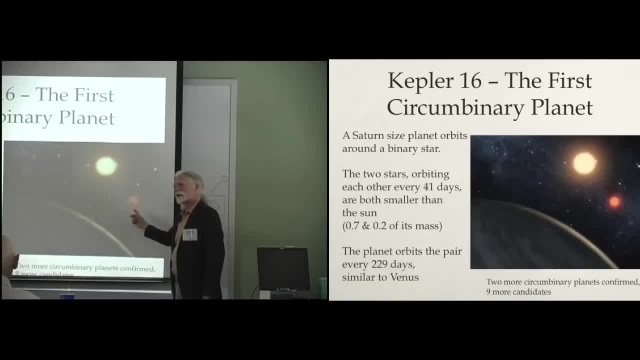 like Saturn. so it's probably itself not something really messing with each other's orbit, these two eclipsing rockets, these two stars, But this object, here they are so far away, it just is a point: mass And the planet. 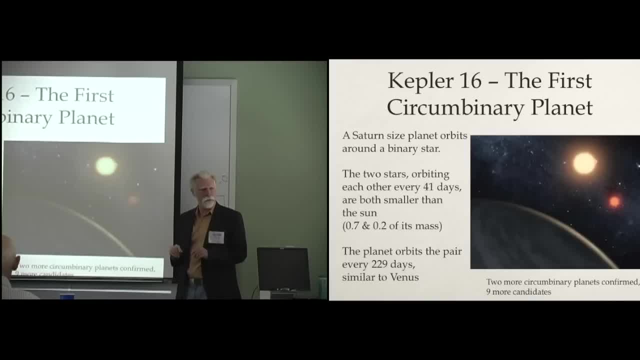 has a happy circular orbit. It will be stable for the next five billion years at least. So this is one of those great, you know Newtonian things where you're doing calculus, where it says, well, here's a big mass, and your teacher 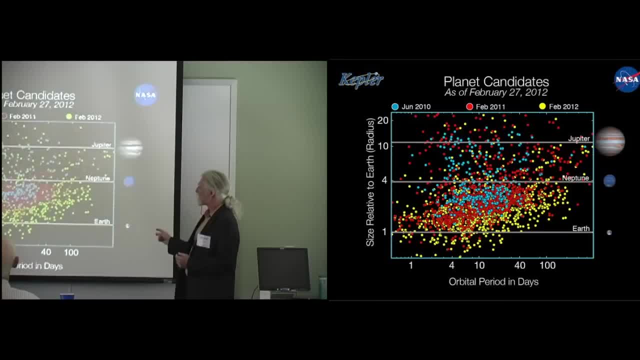 and your teacher is all about makingotoment, Right, So that will be our assignment in the future. All right, So I just wanna finish up on extra planets. This is our current level of February. There's actually about maybe a thousand more. 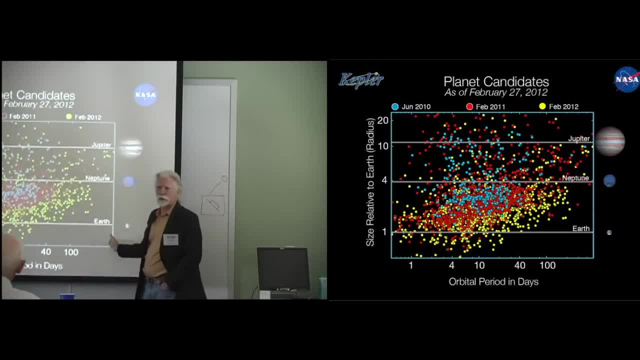 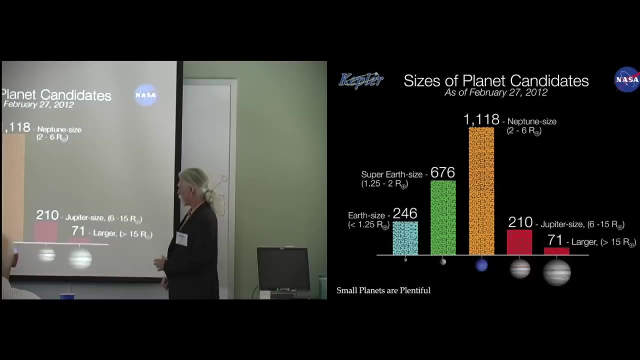 now that are coming through the mic And you can see that if you look at the times here- from June to February to this current- We're going in the right direction. And if you take a census of the size of planets and you bring them up into these sorts of bins here, from Earth and the magical super Earth. we don't know what to call these because our solar system doesn't have any of these. And we have these and we jump to this. So it turns out that Jupiters aren't all that common. 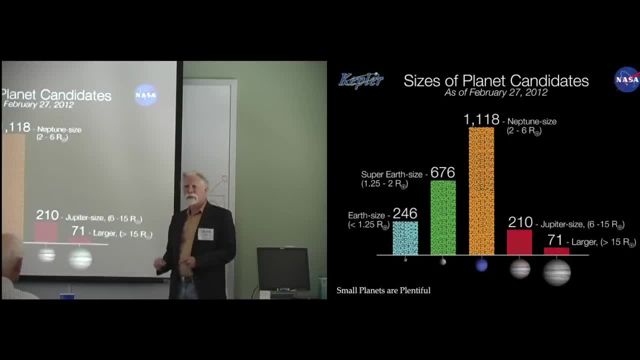 And Kepler now is essentially 100% confident in finding Jupiters. There's not a single Jupiter that we would miss, possibly a very little raging one, But so this is a really well-validated number. There just aren't many big planets in relatively short. 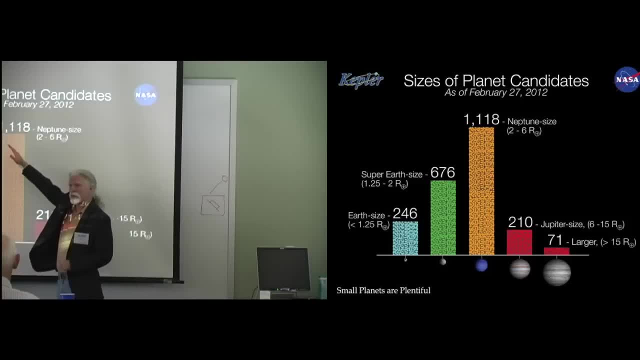 period orbits, But as you go to smaller planets this arises, And these are not yet statistically significant because we just haven't found them all yet, But I bet it's going to be that this is just going to shoot up, Like with everything, there'll be more small planets by far. 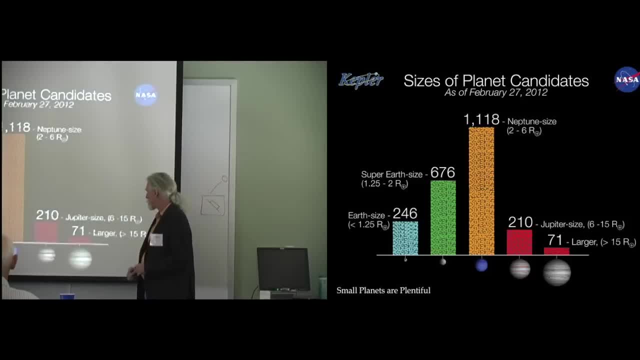 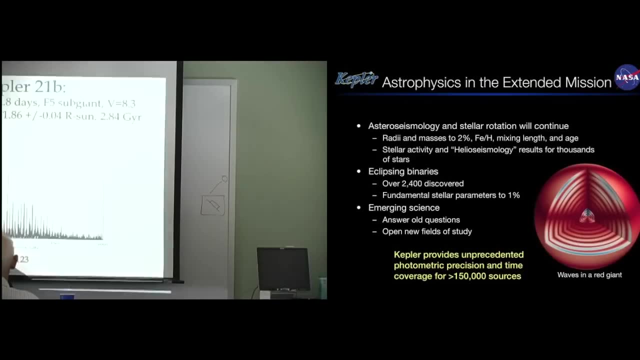 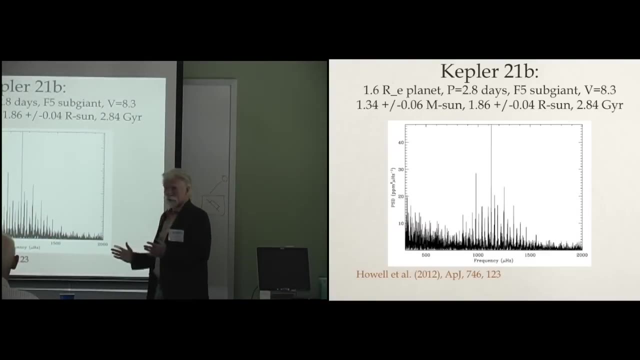 than big planets And small planets are going to move the universe. OK, so running late. Oh, I just want to talk about a few cool things in And I'm happy to talk to people afterward about stuff. So seismology: you've heard about seismology. 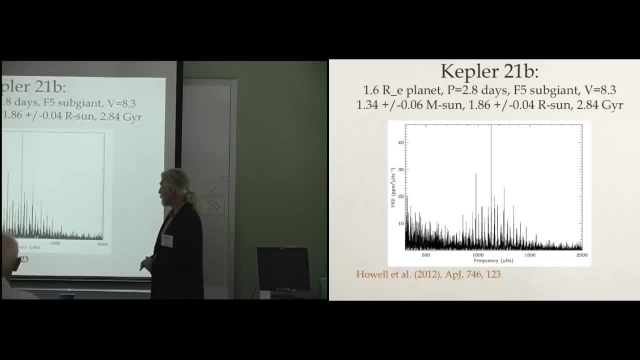 Well, Kepler is doing seismology with its light curves, people working on the data, all sorts of people. This is a power spectrum of a particular star that has a planet. This happens to be an apple sub-giant. It has a pretty small planet, 1.6 Earth radii. 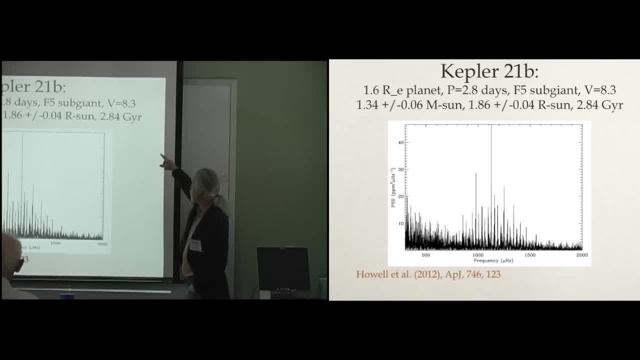 in a short period orbit, But because we have seismology on this, we know the values of this star And we know the size of this star incredibly well in terms of its mass and radius. So we know the planet size incredibly well. 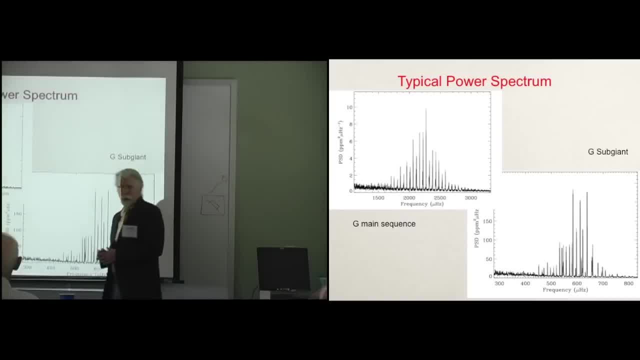 So that's one of the neat things you can get from seismology. And the other really nice thing about seismology is you can tell main sequence stars from sub-giants and from giants, And remember earlier on we talked about, if you don't know, 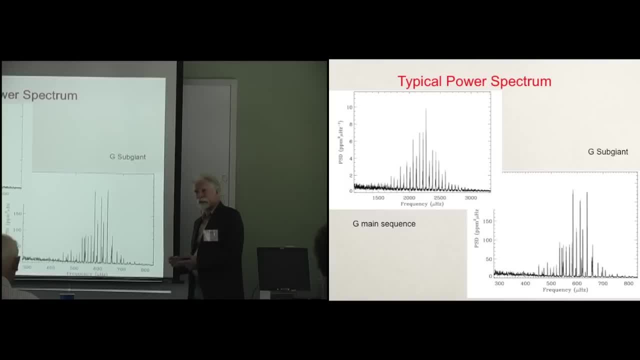 the size of the star. you don't necessarily know the size of the planet. It's just a ratio And so if I think a star is a main sequence star and it's really a sub-giant or a giant, the planet will be a different size. 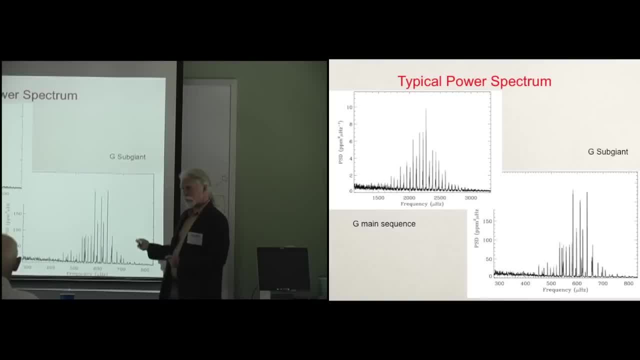 So if I can get seismology information, I can tell from their power spectrum, because they tell me how the modes work inside these stars. I can tell them apart. That's very nice. I have a question? Yep, All right. 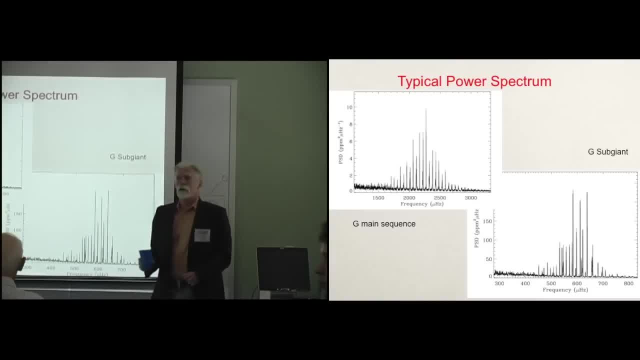 So you're only looking maybe three, four, five pictures on a star. How do you get the seismology on that? It's all just coming from the light curve itself. It's just the variations of the light curve. It's little pulsations in the star's atmosphere. 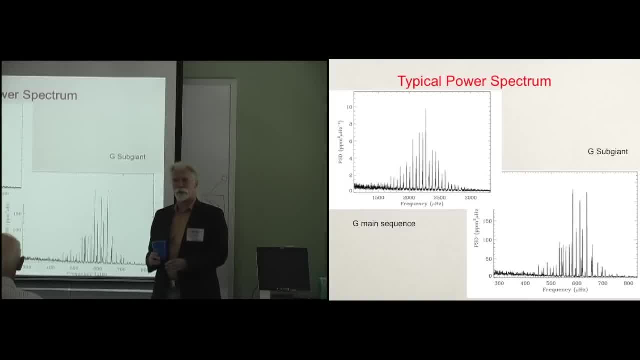 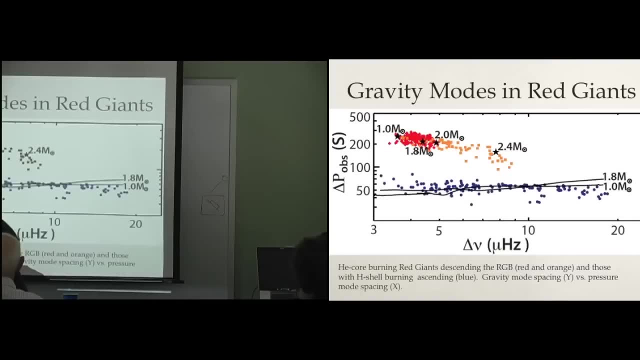 that are telling you about the modes that operate in the star. You're not resolving the star, You're just seeing them all in the light curve. So the things you can do with that, which are really neat, are you can separate stars on the red giant branch. 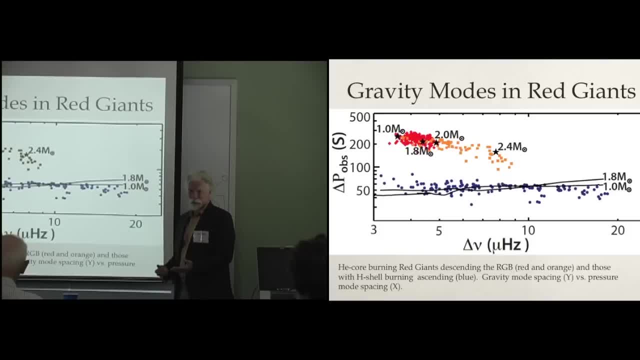 between ones that are ascending the red giant branch and ones that are descending the red giant branch. You can't do this any other way because they look the same to you on the outside, But they're fundamentally different on the inside, and that's where these pulsation modes really help you. 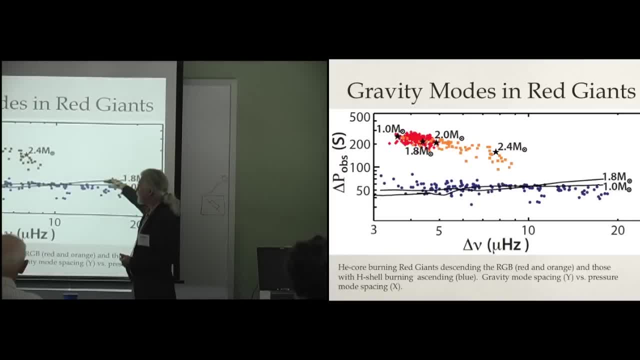 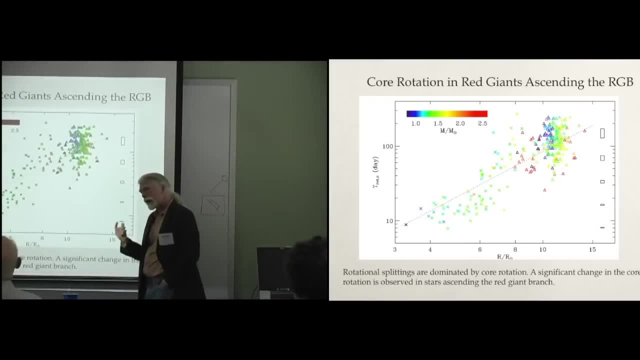 So you can separate the ones between these particular pulsation modes in the middle. So that's really a neat thing to do. Another really new result here is the rotation period of the core of a red giant, And you can get the rotation period of the core. 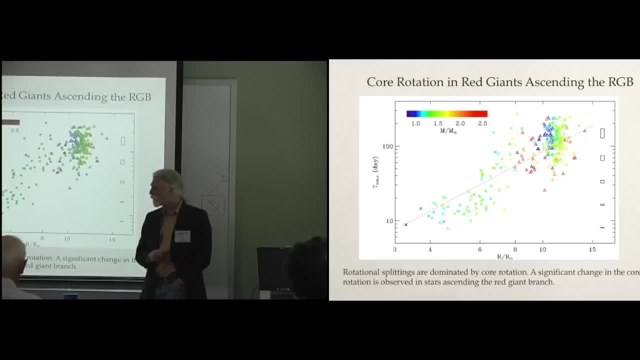 You can never see it, but you get it because of the modes that propagate through the star. And you can see that for these red giants here, the ones that are relatively small and still moving up the red giant branch, they have a very different rotation. 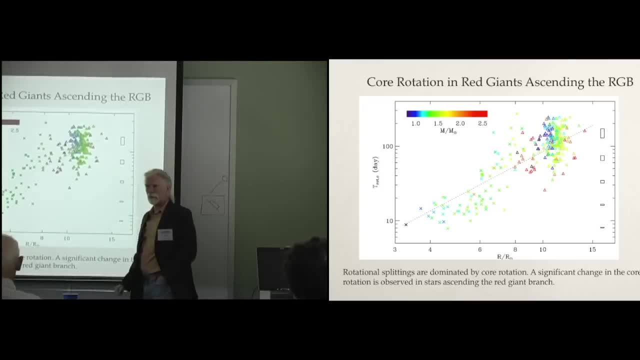 and it breaks very quickly here and goes to another level of rotation. So this down here is the size of the star in solar radii and that's the rotation of the core in days. So that's a really cool result here. Now, these two last results are red giants. 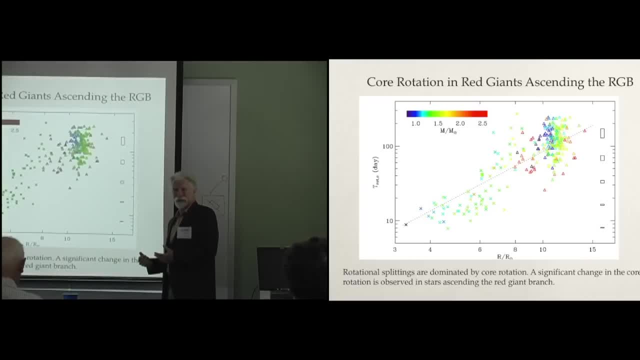 and that's because red giants tend to be great. They have very luminous stars, So the seismology for them so far has been superb. Now it's moving down to main-sequence stars, where again, you just look at it longer and longer and longer. 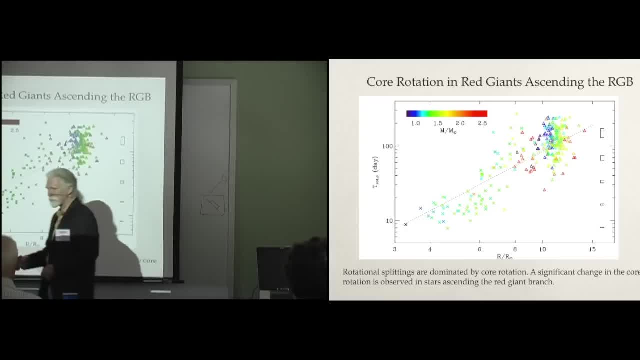 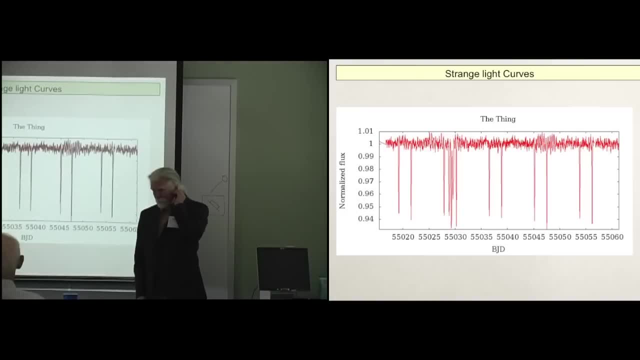 and you co-add all your data and all these pulsation modes just pop right out. So it's working on those. Let me just show you one more example here. This is a really cool light curve. See, you can read me for it and I'm saying it. 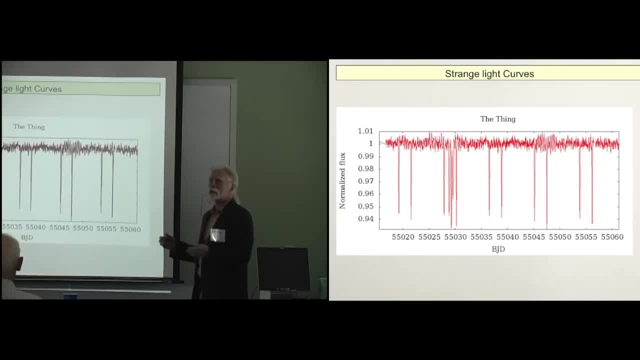 This is one of my students. This is their clever thing. They're naming all the light curves. now, There's a lot of them. They're running out of names. So what is it? This is really tricky. Could be planets, could be stars. 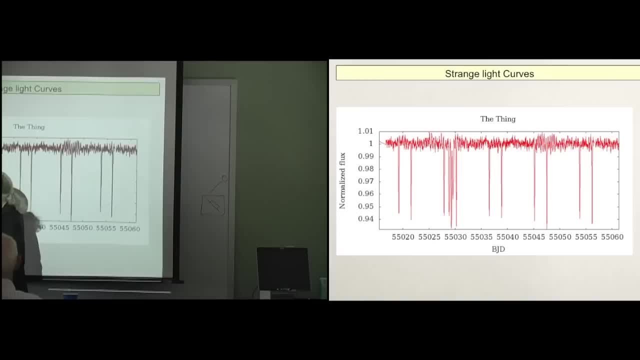 And you can see over here this is a normalized light curve, so the depth over here this is 0.95, and that's water That looks awful big for a planet. So right away you think, oh, maybe this is an increasing fire. 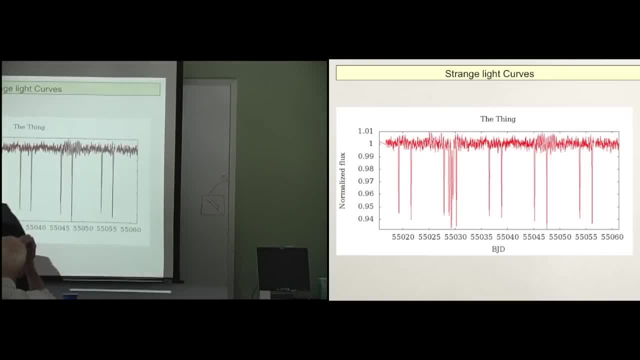 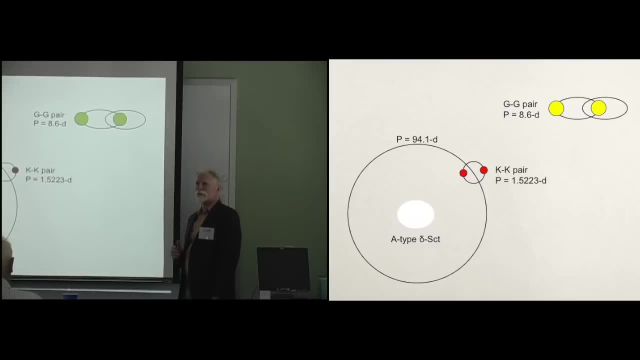 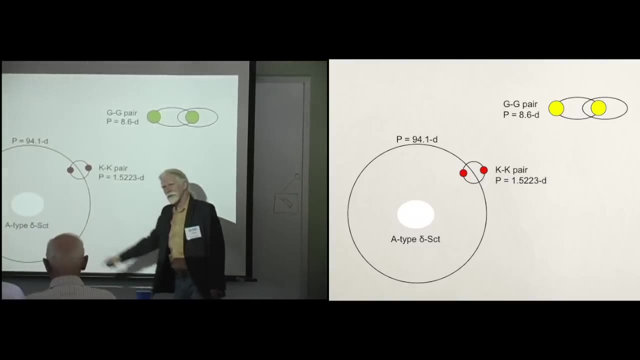 So it's a ground-based spectra seen with the stars, and now we came up with this model, this object. It's a system containing five stars, where this pair orbits these three and that pair orbits that one. So it's just a really complex star. 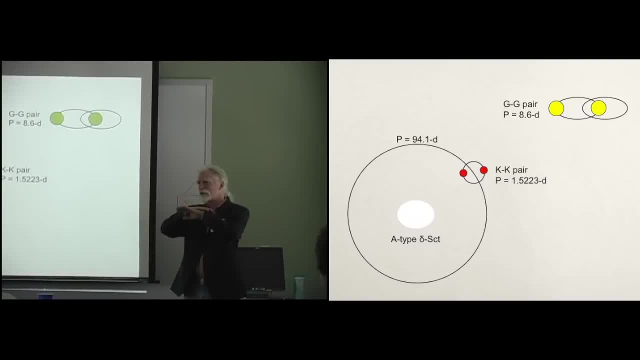 And they all, of course, are perfectly aligned to us, because we see every one of them eclipse every other one of them in crazy sequence, and which one's eclipsing at which time. This is just fantastic. So the neat thing we're going to do. 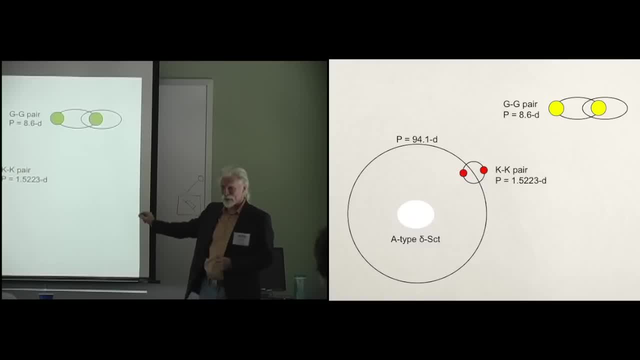 well, it's already neat. the neat thing we're going to do is we're going to get a high-resolution image of this. These two are about a tenth of an arc, second apart. We should be able to see this system for our high-resolution image. 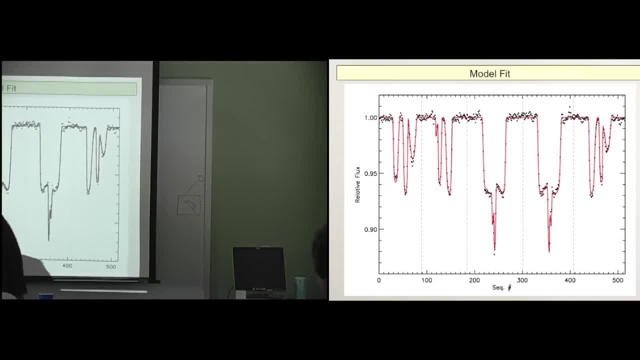 So this is the model and if you fit the model to the particular light curve, the model's the red and the particular light curve's black Works pretty well. Now you might say, with all these eclipses and all the possibilities here. 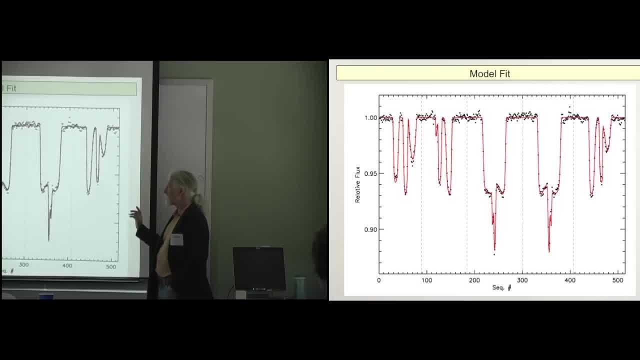 how do you know this is a unique model? Well, it turns out this model is not just running a spline for new data. This model has real stellar parameters in it of sizes and temperatures, so that you can't make these dips be any bigger or smaller. 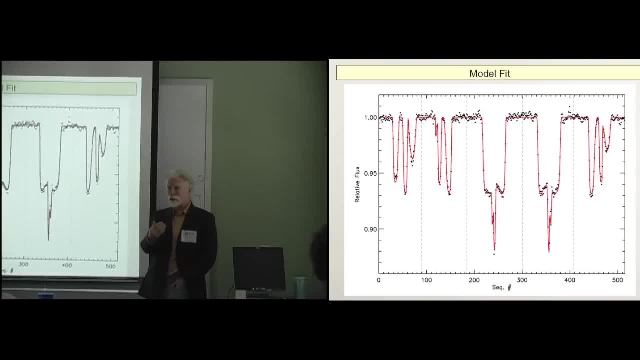 than they would be given. whatever luminosity star is being eclipsed by whatever other luminosity star, You have to have all the orbital periods correct of all those little binaries, And so it's really a much more complicated model. It's not just a spline for new data. 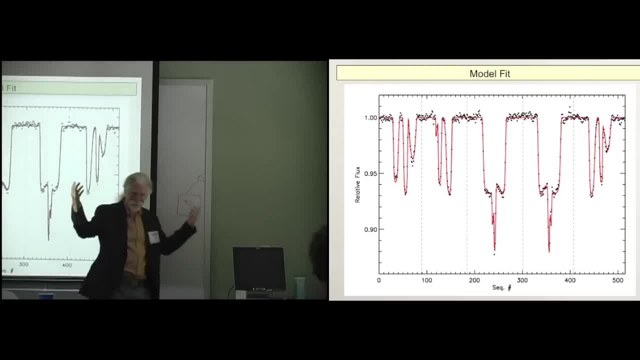 And you see, it doesn't work right there, And you know so, it's not perfect, But it works pretty much everywhere else. So something else is going on there. But what a cool system. Okay, I have one more. Sorry, I have one more. 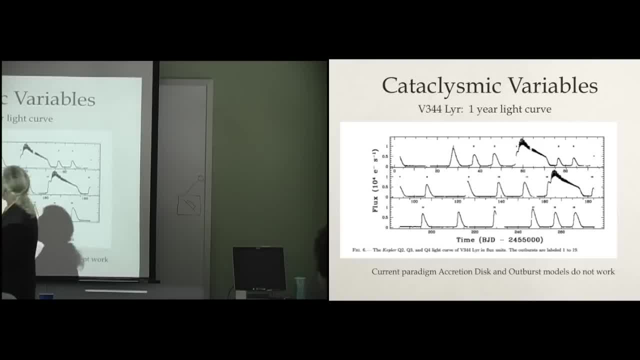 because I promised you an education thing, Okay. Okay, so this is a cataclysmic variable. This is an interacting binary. It's a white dwarf which has something like an M star orbiting it with a period between about 80 minutes. 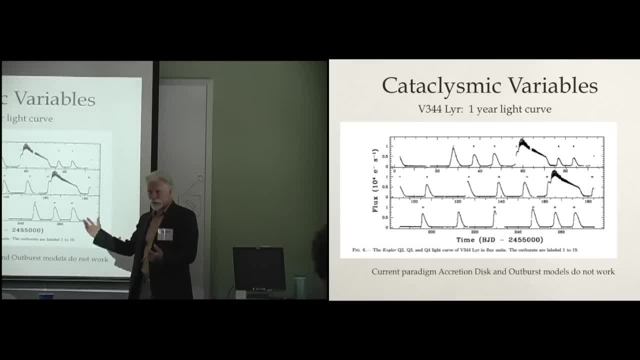 and about four hours. So these have been known for centuries. People don't understand them ever. They have something to do with a disk And there's all kinds of flaring and outbursts, And so the light curve comes along, And every so often it has this brightening. 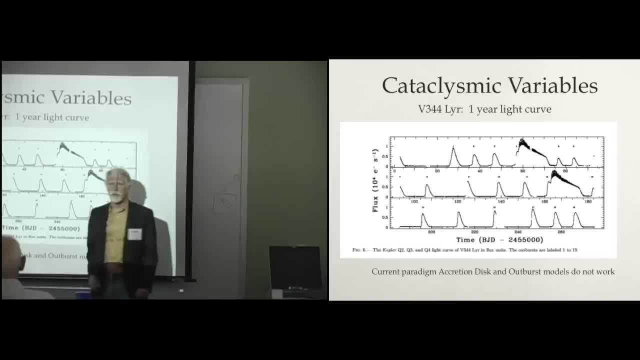 that's about in this case. you can't really tell from the flux scale, but in this case here it's about three or four magnitudes, And this is thought to be. the accretion disk gets brighter, So an accretion event happens. 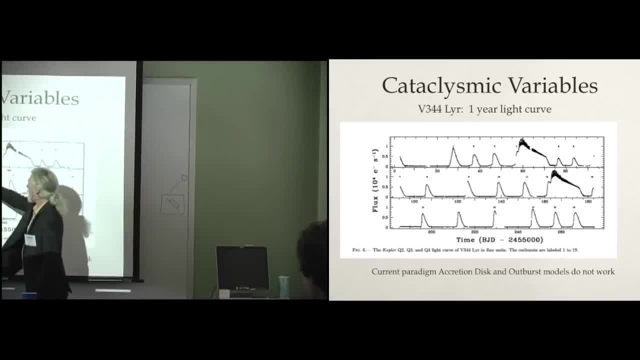 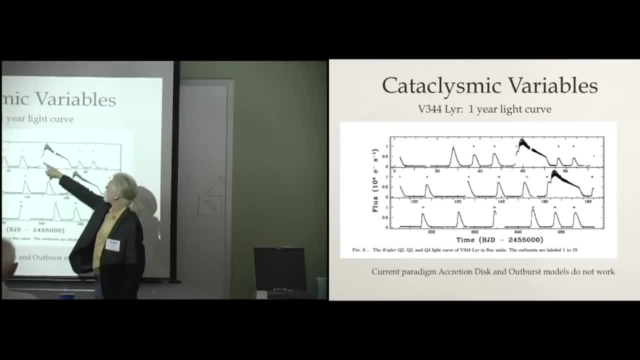 The accretion disk gets hotter and brighter And then it settles down And you can see the outbursts aren't the same. So we don't even understand that Every once in a while it has this bigger outburst that gets much brighter, much longer. 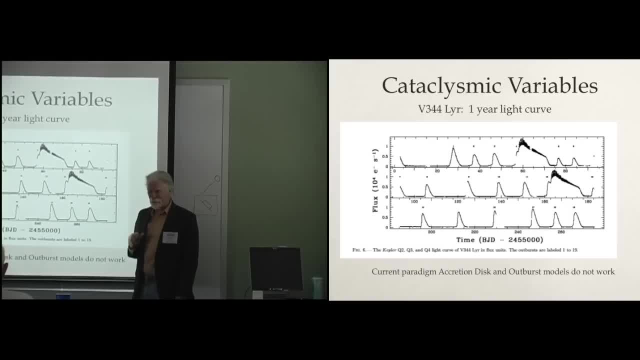 Astronomers have cleverly called this a super outburst, And at the top of these super outbursts there's an incredible pulsation that goes on, which was always thought before Kepler and something to do with the disk oscillating. This particular object was one of the first. 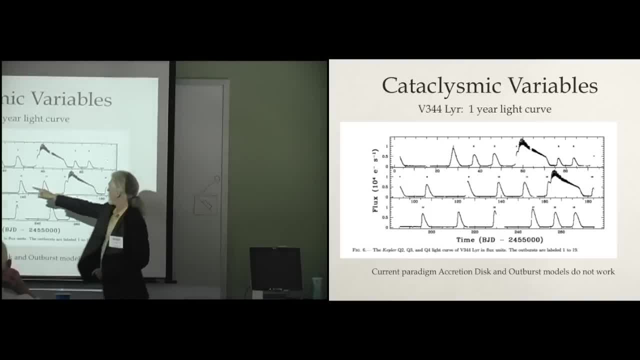 CVs. that was studied in detail from Kepler And by the time this first 90-day light curve was obtained, the sizes and shapes of the outbursts, the way this one worked, completely threw out every theory about how these things worked. 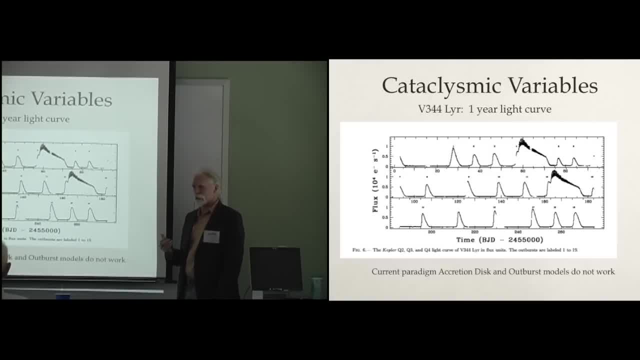 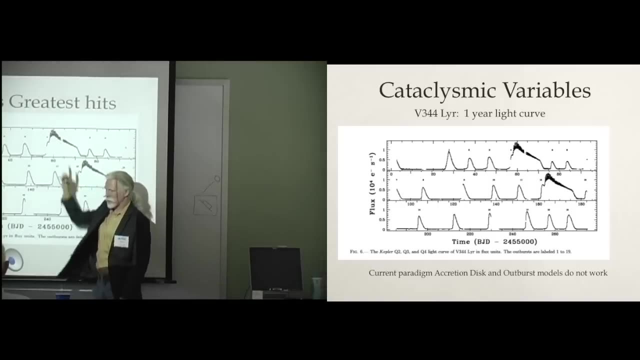 None of the theories worked on this. None of the things they predicted were true. So it's kind of cool. In 90 days you killed 50 years of science. So here's the same light curve. I'm going to zoom in on this little piece right here. 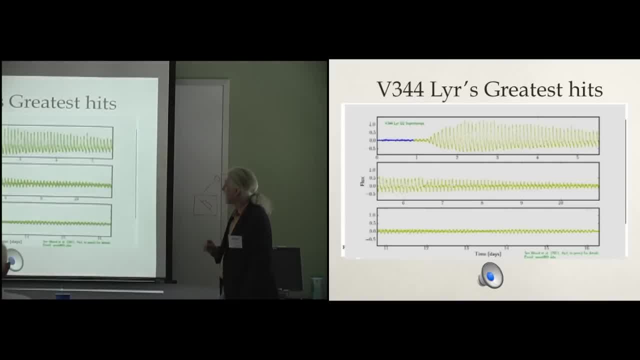 So we're making music out of light curves, and not just for fun. We're actually doing a project with people who are visually impaired. This is the. These are all these oscillations. Your ear is really good at this, because when you look at this, 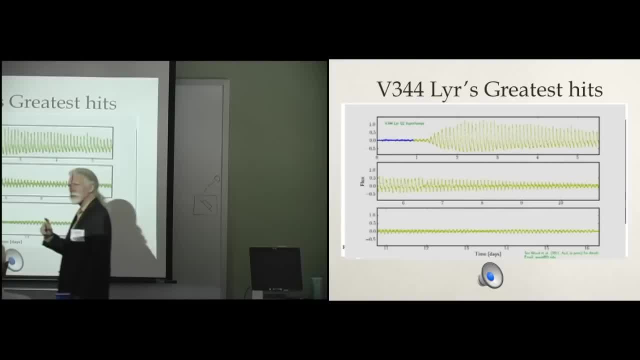 it kind of looks like it does the same thing. Let me jump to another place. Everybody's got that one memorized. It's in F minor, by the way. Now I'm here somewhere And you can just hear. It's not the same at all. 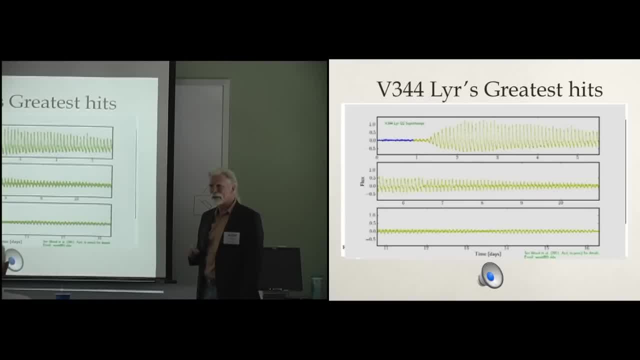 It's just completely different in the structure and the form of it. The amplitude's not the same, The hot work's not the same. Anyway, so that's a lot of fun. So we're doing this with all kinds of light curves. 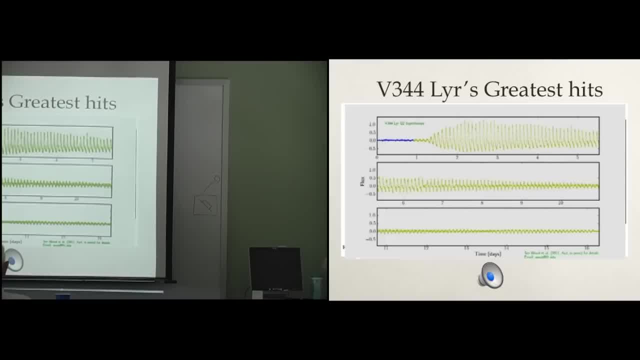 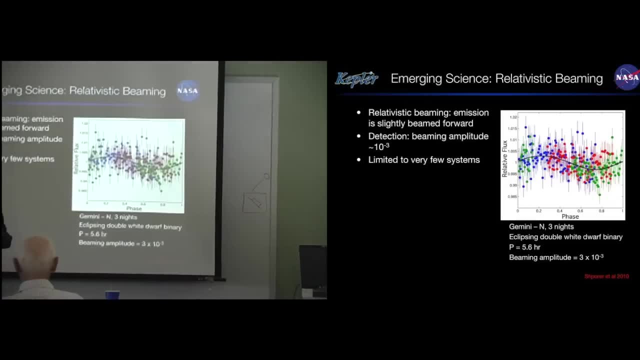 It's amazing the things we're learning. So let me- Yes, yes, That's it. Okay, Okay, One more. really Stop, Because I promised somebody else this one. Okay, So Doppler boosting or relativistic beaming. 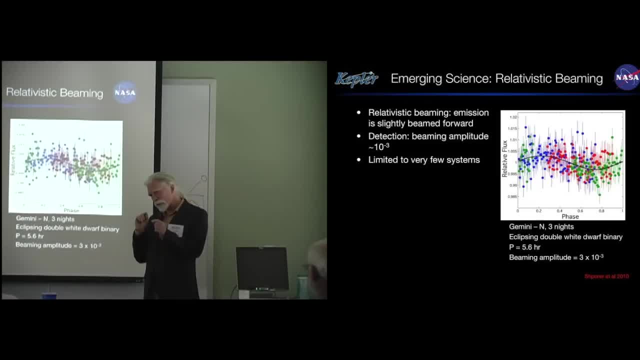 You have two objects orbiting each other. When they're coming towards you or away from you, the light from them, because they're moving, is forced slightly into a cone. They become slightly brighter in the direction of motion because some of that light's forced into a cone. 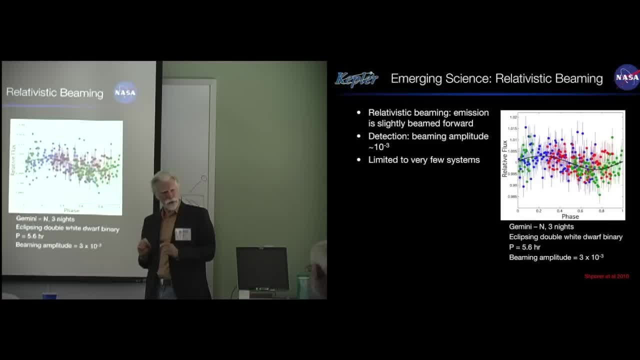 And when they go away from you they become slightly fainter And it's real slight. It's something like at the best case that we thought we could ever do: from the ground 10 to the minus 3. So sort of in the milli-magnitude level. 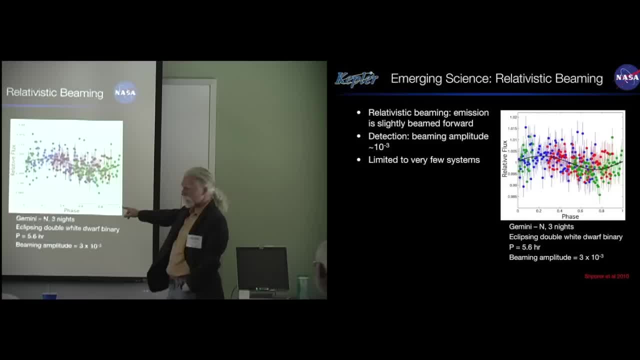 So here's an experiment that was done using the Gemini telescope. It's an 8-meter telescope. It's far bigger than that. We used three nights of data on a double white dwarf binary, So it's two white dwarfs. They were perfectly in line. 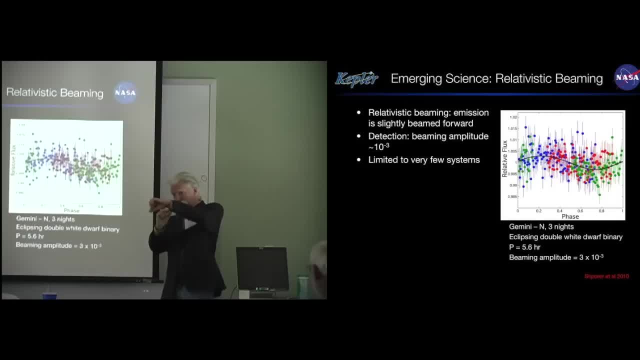 so they're eclipsing like this. So at one point one's moving away and one's moving towards you, And it's a 5.6-hour period in this case, You have plenty of time to set up a light curve So you can fit the so-called beaming amplitude. 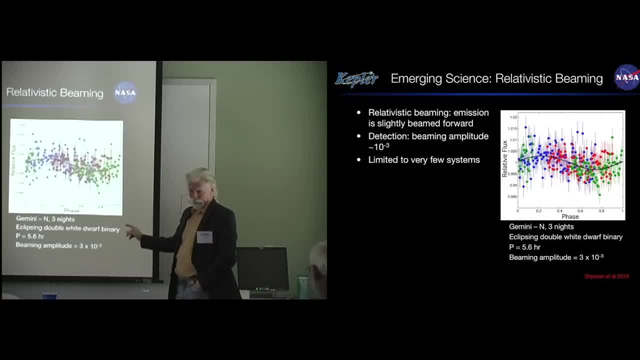 this change in light that's only due to the fact that they're moving towards you or away from you. It's a relativistic effect And you get a sign-like signal from it. This is it. It's a light curve, It's a light curve. 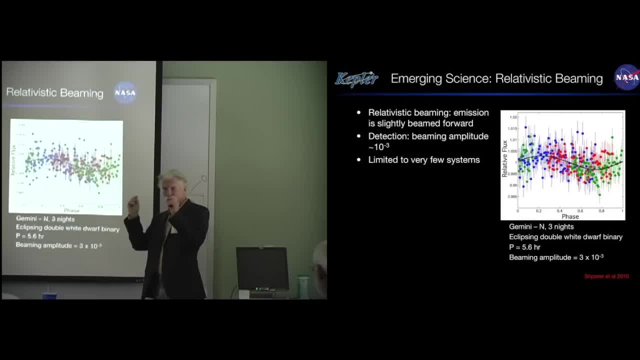 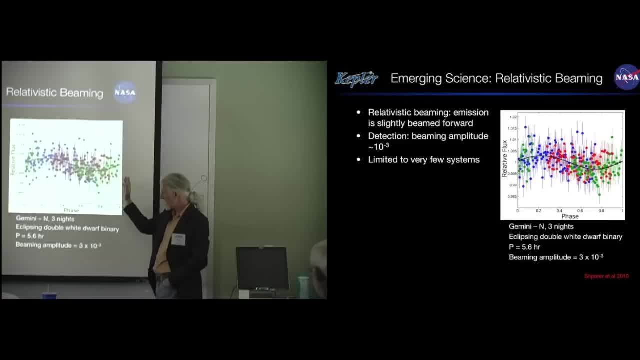 And pretty good, I was involved in it. I'm glad. Okay, Kepler came along. Here's a light curve from Kepler with an orbital period of five days. Remember that other thing was 5 days, So it's a light curve. 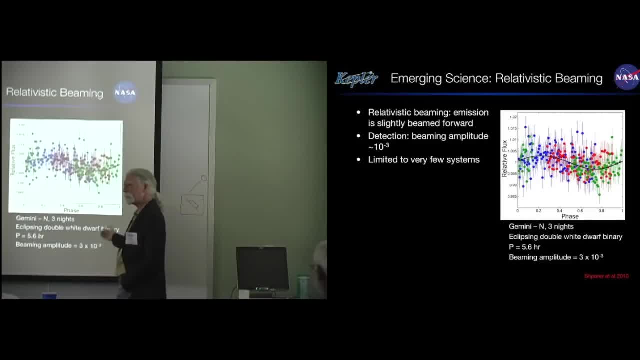 It's a light curve And it's a light curve, So you get a sign-like signal from it. This is it. You believe that's a good fit for the data. The colored points are different nights And this amplitude in this case. 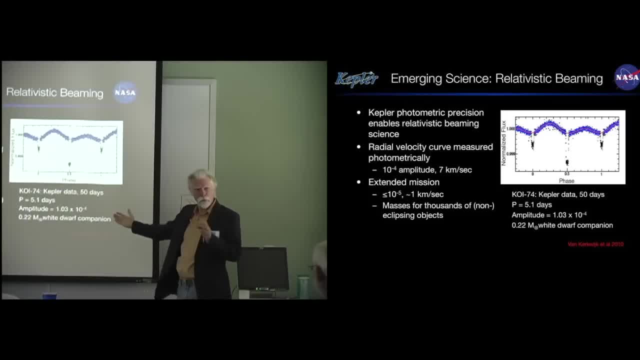 is 3 milli-magnitudes. This was the best attempt to ever do this before Kepler was launched. Remember that other thing was 5 hours, So each night you would get a whole orbital period. So you can never do anything in 5 days. 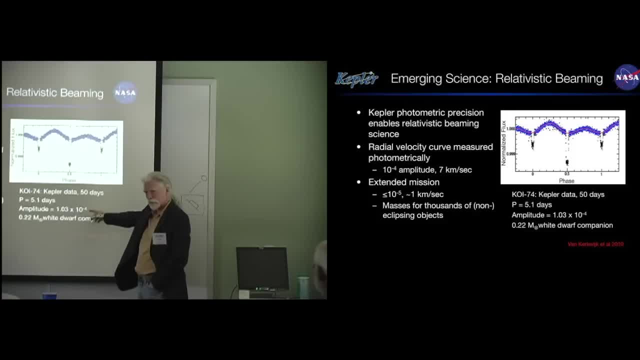 It's just never going to happen. And this has an amplitude of 10 to the minus 4.. This is a white dwarf and an A star, So an A star is much larger and much more luminous than a white dwarf. You can never see this A star. 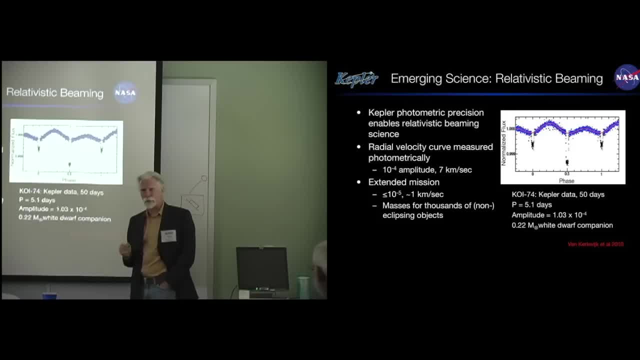 in any kind of observation you want to make. It just wouldn't show up. But you can look at this light curve. I mean, just look at it with your eye And you can see the top of the thing, And you can see. 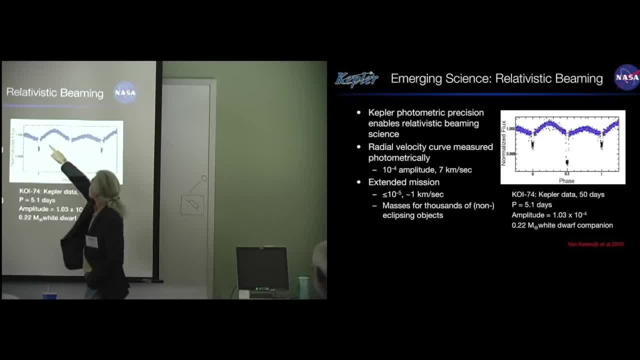 the top of the thing And you can see how it's brighter here than it is here. This stuff just comes out of the Kepler light curves. This is just a phenomenal result. So this was actually fit and found the mass of this white dwarf. 0.22 solar masses. And this was the first example, although ours was kind of the worst. but this was the first real example of getting a radial velocity curve from photometry. That is really cool, If those two terms mean anything to you. 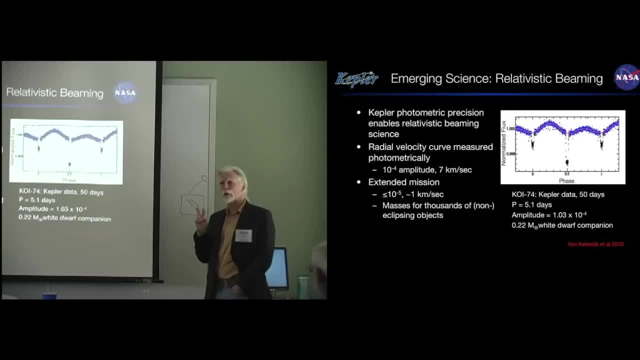 think about that in like 20 minutes or not, You can say, wow, that's really cool. So this is the first example of that. That was really cool. So the neat thing about this is you cannot find the masses of small planets. 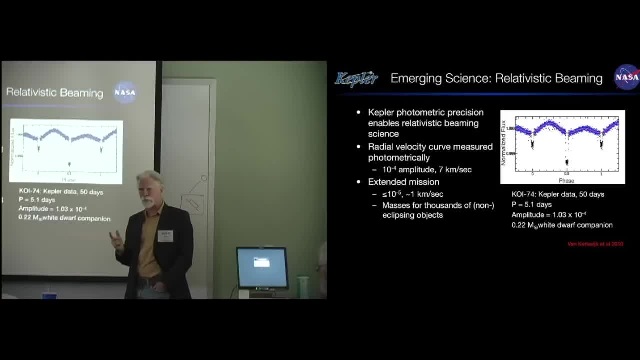 with spectroscopy, even using the Keck telescope, forever, But there's a possibility. we'll be able to get the masses of those planets simply from the Kepler light curve by using this technique and getting basically their velocity, amplitude, their mass by their light curve.